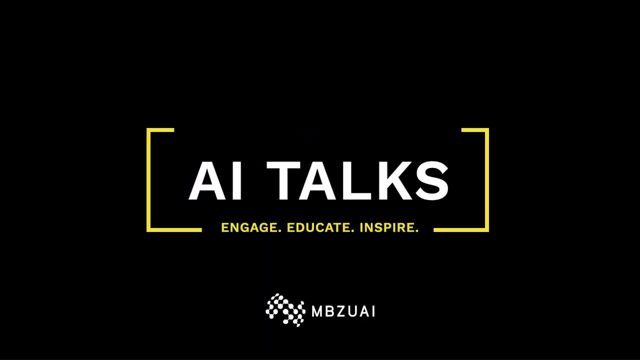 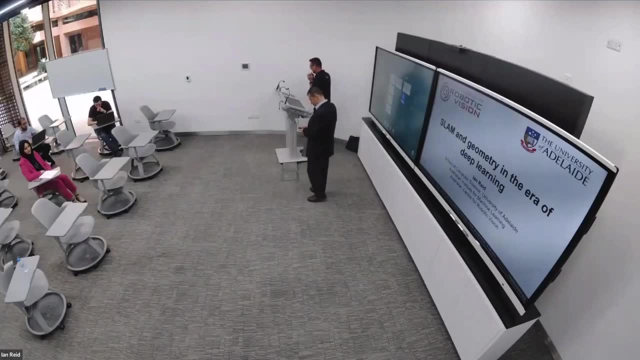 Thank you for coming here. Thank you, Professor Ian Reid, for being here with us today to give us a very nice, hopefully very informative, presentation on SLAM and geometry in the era of deep learning. Professor Reid is a professor of computer science at the University of Adelaide and where he was head of the school of computer science from 2018 to 2022. 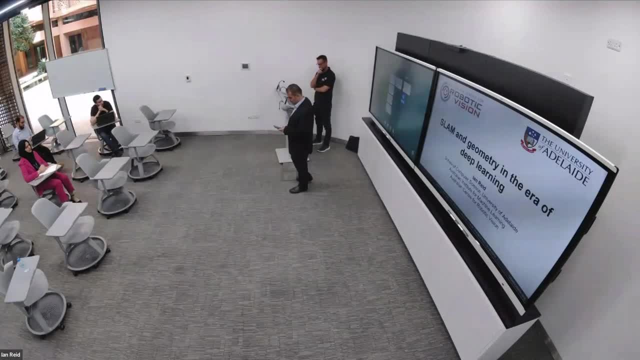 He's a fellow of the Australian Academy of Technology, Sciences and Engineering of the Australian Academy of Science, former Rhodes Scholar, and he held the Australian Laureate Fellowship from 2013 to 2018.. He has been, Or he was, a deputy director of the Australian Center for Robotic Vision- so we can see it roboticvisionorg until last year and worked on computer vision for more than 30 years, with research interests ranging across broad fields of the computer vision, and he completed his PhD in Oxford in 1992.. 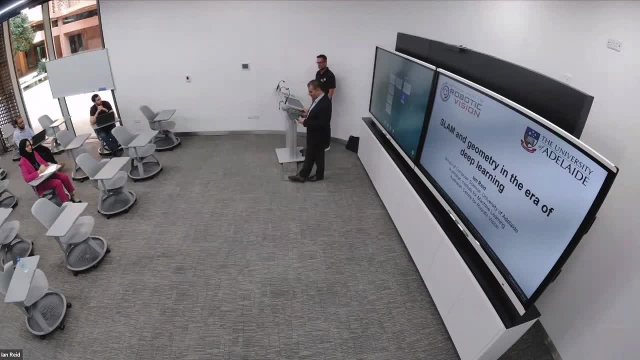 He was appointed as a lecturer professor in Australia in 2018.. He is currently in Oxford from 2000 to 2012,- and in 2012 he returned to his native land, Australia, where he enjoyed watching birds at the University of Adelaide. 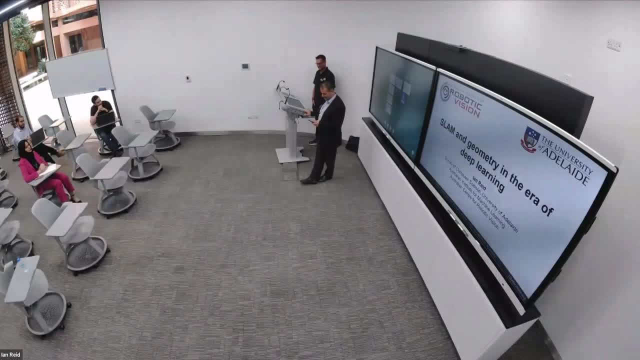 He has made landmark contribution in areas such as active vision, visual SLAM, visual geometry, human motion capture and intelligent visual surveillance. He is currently focusing on lifelong deep learning. He has published extensively and widely with high impact research and his citation counts close to 50,000, and with an index of 97.. 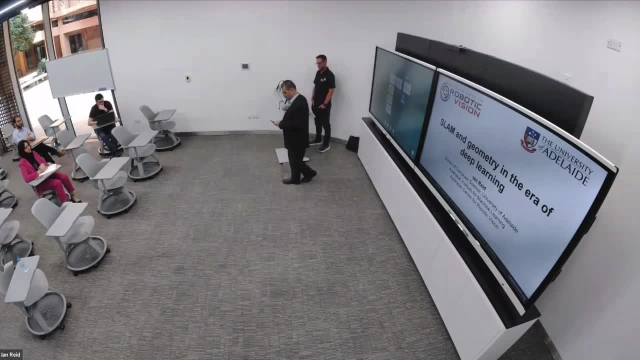 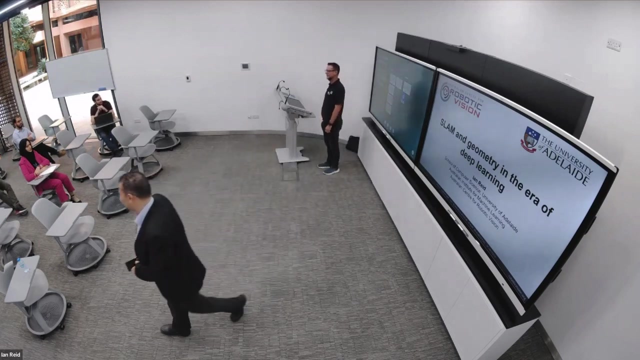 He was recently awarded the Australian Computer Society Artificial Intelligence Distinguished Researcher in 2022 in recognition for his lifelong learning contribution to computer vision. Thank you, Thank you very much. Thank you very much. Thank you very much, everyone for coming here and everyone online. 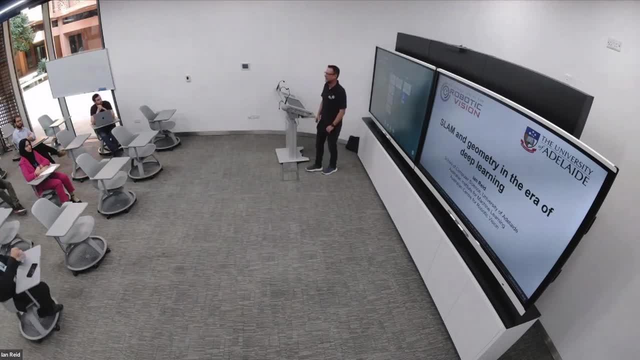 And I hope I can give you a sense of the journey that I've been on in research over the last decade, How that's changed over the last 60 to 90 years, changed over the last decade in the era of deep learning. so for those who don't know, I hope 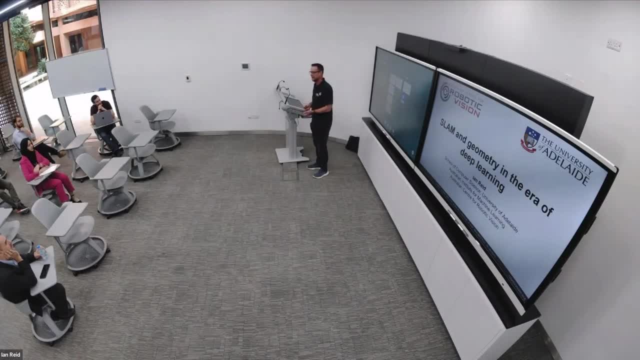 everyone does know that SLAM is an acronym that stands for simultaneous localization and mapping and it's the idea that a camera or a sensor in general- so visual SLAM, if it's a camera- can move through an environment and using the geometry of the 3D to 2D projection and the 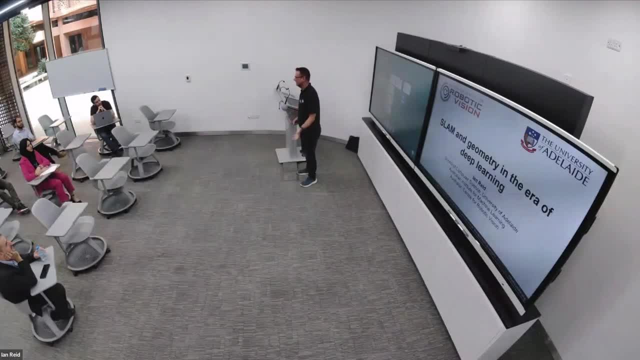 sequence of images, you can work out a map of the environment, so where points are located in 3D and where the camera is relative to that map you're building and I'm interested to talk about the journey that I and my colleagues- so I've got a lot of collaborators here- postdocs- 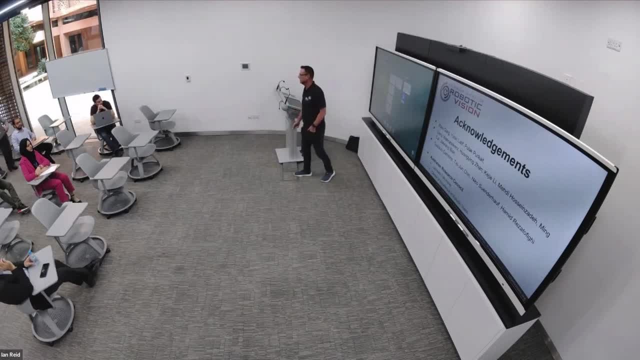 students and fellow investigators, fellow lecturers, people like Gustavo Canero Tatra Chin, Niko Sundarov and Hamed Rizat Afegi have been collaborators for many years. and then I've worked with a series of excellent students and postdocs, some of whom I'm still working with, and this work was funded. 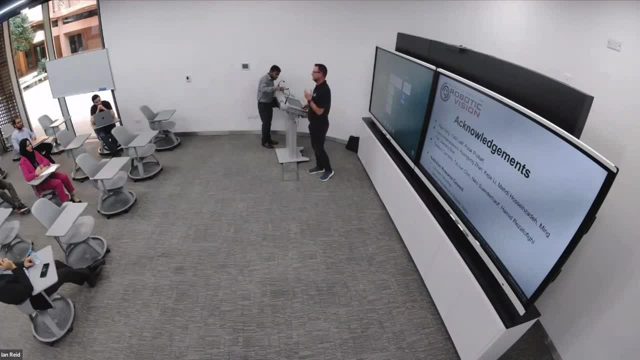 I should do my standard acknowledgement funded by the Australian Research Council through, as you heard, in my bio Laureate Fellowship, which is a fellowship from the Australian Research Council, Australian Government and also the Centre of Excellence in Robotic Vision, which was a seven-year, multi-year multi-institution research program in which I was deputy director in association with Queensland. 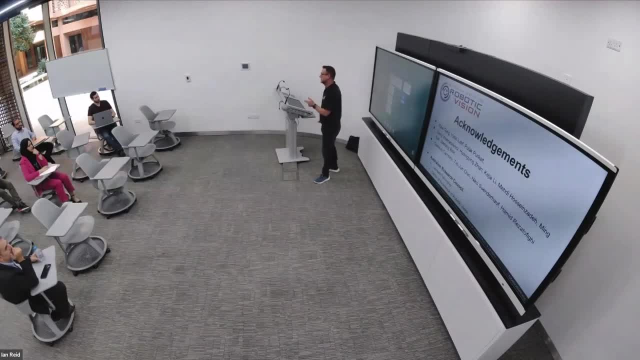 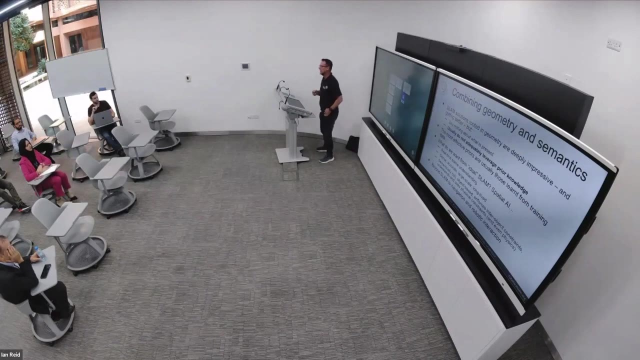 University of Technology, Australian National University, Monash University and University of Adelaide, where I'm based. so I'm interested in how we can go beyond pure geometric slam and slam solutions over a number of years got better and better and to the point that they're deeply. 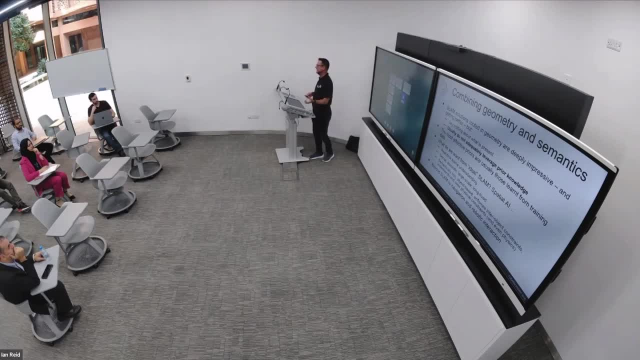 impressive, but were rooted in geometry, by saying nothing about what was present in the scene. there's just a point cloud and where the camera happens to be relative to that point cloud, and rarely have they adequately leveraged prior knowledge and what we've learned over the last, I would say, 15 to 20 years in. 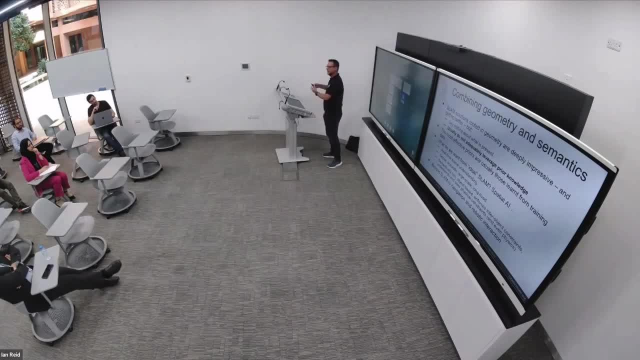 computer vision, is that often the most effective priors that we want to use to, to be able to leverage prior knowledge are ones that we learn from, from data, and, and hence the important importance of training data. I also want to think about the question: what do we want from ideal slam? 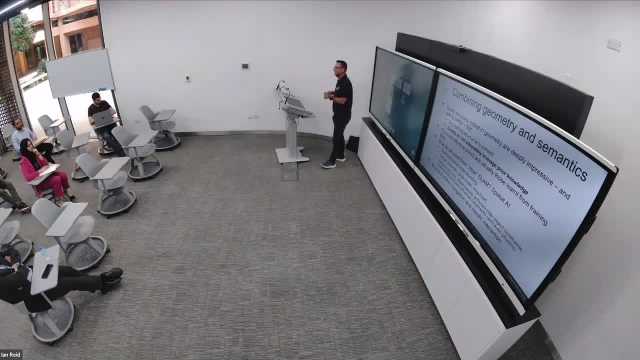 is it just about localizing a camera or do we have the possibility of going beyond slam to turn the camera into a spatial AI sensor? and I don't. i'm not going to lay claim to the the term spatial AI, that that was one that I first heard my my close colleague, Andy Davidson referring to, but it's. basically the the idea that we can turn the camera into a real-time situation of future AI and make a difference from what was earlier important to us: making a change and making a change actually, that's something that we have to be aware of and we've got to embrace where we need to be and we have to. 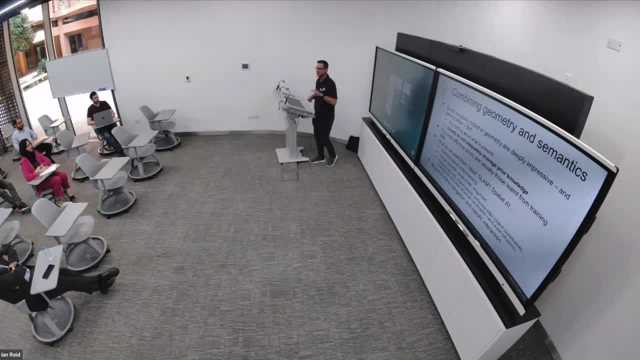 be aware of what's really important to us and how we can actually work together. and how we can work together and how we can actually do a good job at that and we can actually expect that we can work together. a real-time situation awareness device that's telling us not just about geometry, but about 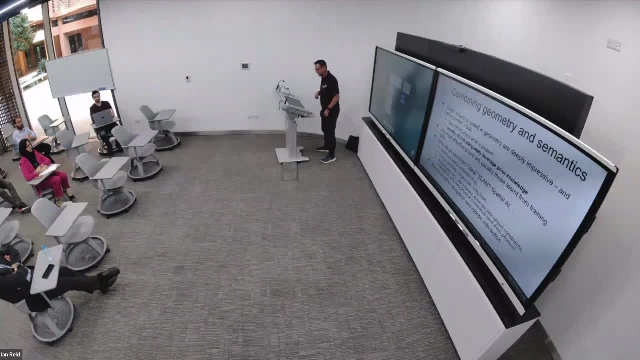 what's in the scene, what's going on and can we anticipate what's going on, and so forth. so, ideally, what we have is something that can do. real-time scene understanding can produce dense, accurate, large-scale and long-lived maps of the environment that are populated in a semantically 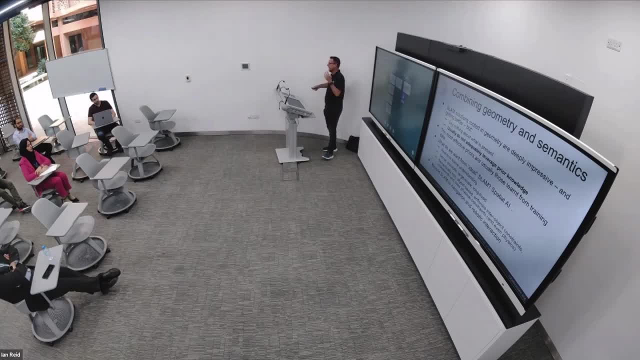 rich way with objects, not just point clouds, but perhaps even enforce inter-object constraints and so forth, and and ultimately from- from my perspective, this is one of the applications of such a such a device- if we could create it- is that we can go beyond, uh, localizing a camera to doing. 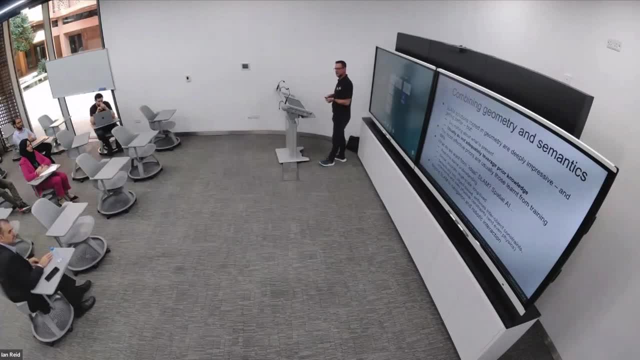 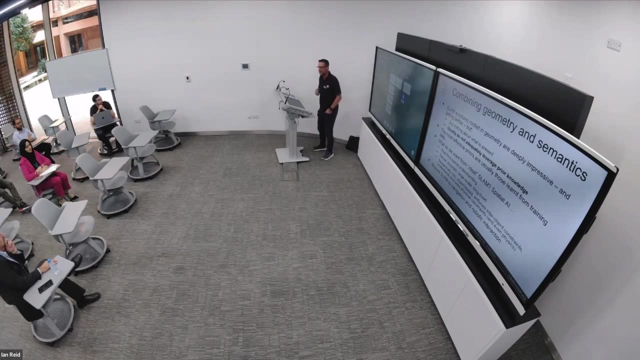 real robotic tasks like navigation and robotic interaction, um just through using the uh, the camera as the sensor for this robot, and there are obviously lots of other applications of um, spatial ai, real-time slam and so forth. one that particularly gets me out of bed is this one that associates it with robotic interaction, so i'm interested. 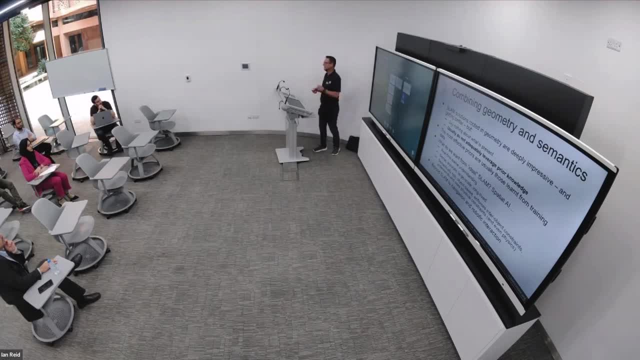 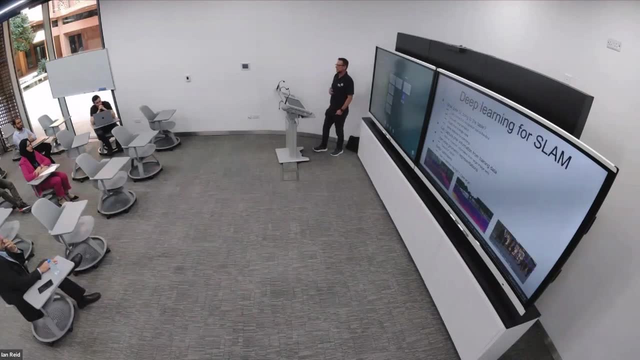 mostly in applications that run in real time, because that way we can do real-time robotic interaction. so it's natural to ask the question, and a few of us have been asking this question for around about seven or eight years, ever since deep learning has well separate what i suppose. 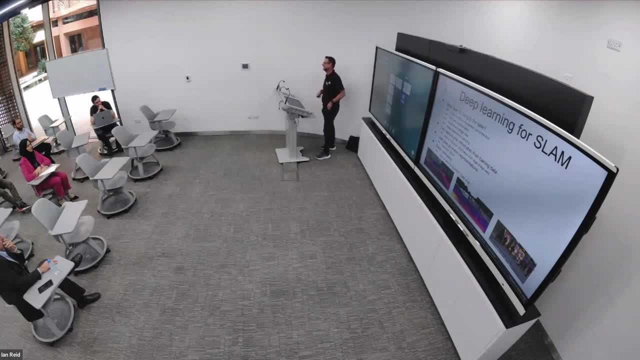 2012 was the the first time it really came into the, the computer vision consciousness, with the, with alex net. um, what does it bring to the table? so it brings to the table a bunch of things that now we take for granted as being just turnkey solutions. we download our favorite. 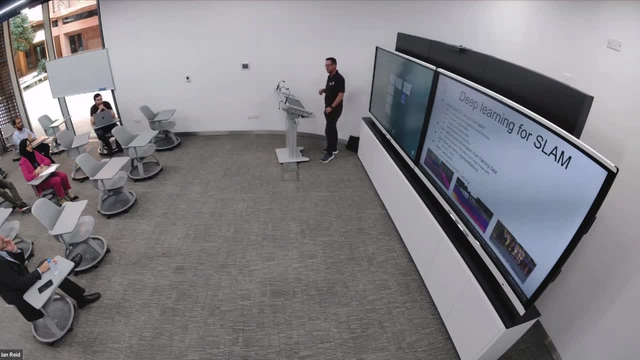 object detector and we can do object detection and recognition out of the box. we can do things like, um, semantic segmentation- uh, we can. so we can add a label to uh, every uh stuff, like if i go down here second, oh no, um, i'm just gonna point. i hope you can see up here that i'm i'm pointing to. 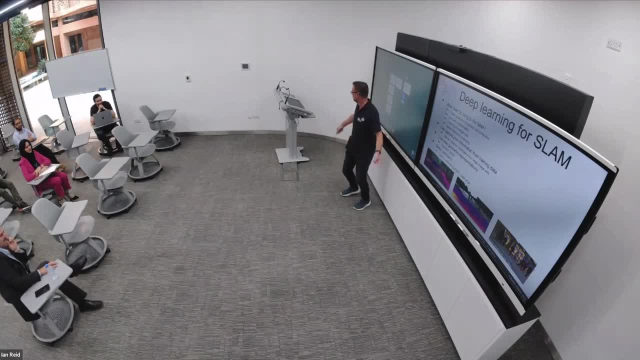 something. this, um, this thing doesn't seem to work terribly well. if i is it, if i move away, high-tech solution is not nearly as good as the the low-tech solution down here, you see, you see, you see an image where every pixel has been labeled with a particular 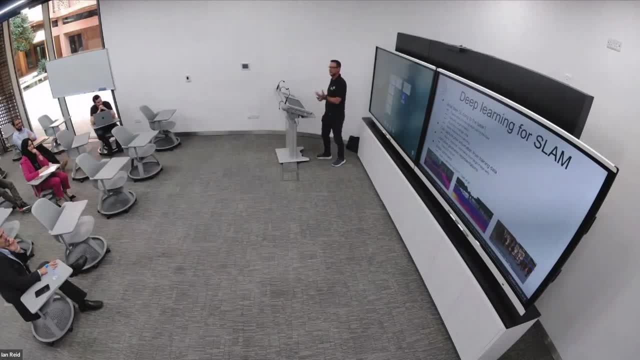 class. um uh, we can do depth from a single view, and i'll talk a little bit about that later on. we can do things like better matching. matching is a fundamental problem in multi-view geometry and a number of other computer vision tasks, and and deep learning produces out-of-the-box better. 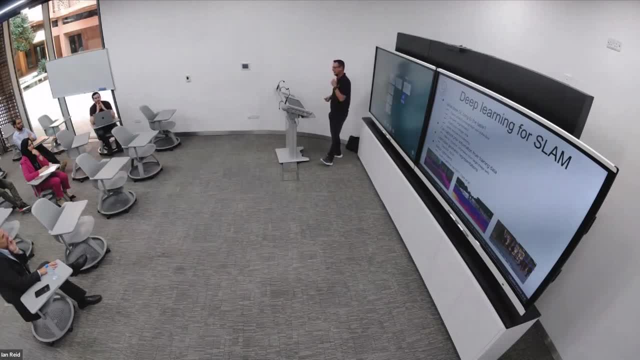 features for matching. i guess, more importantly and more interestingly, you can do things like capture prior information from training data, so perhaps we can squeeze information from large image sets that help us with our reconstruction and, in particular, one of the the very interesting things that is happening, uh, at the moment, and i'll show you some preliminary results and other. 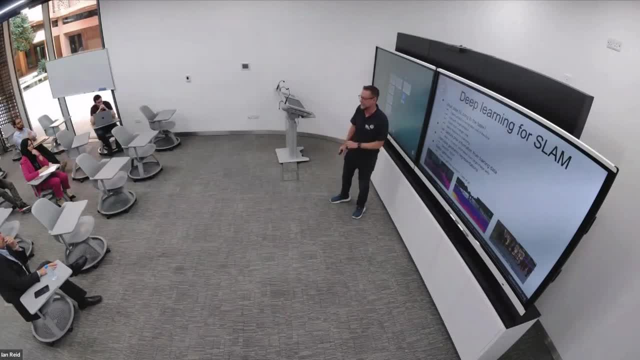 people around the world are working on this as well. so, as you can see at the end of the slide, in this slide we have a another. one of the other studies that we're doing that's really interesting is using the geometric representations, so using uh ideas from deep learning, so to learn 3d representations, uh, rather than rely on point clouds or meshes and so forth. another really interesting thing- and i won't talk about this at all, but i do want to point to some work from um, uh, ronnie clark, for instance, uh, formerly at imperial, now uh, now back at oxford, who's been working on the idea of deep learning for optimization- um, and, and you may have heard of the algorithm raft that's come out of princeton- recurrent or western. 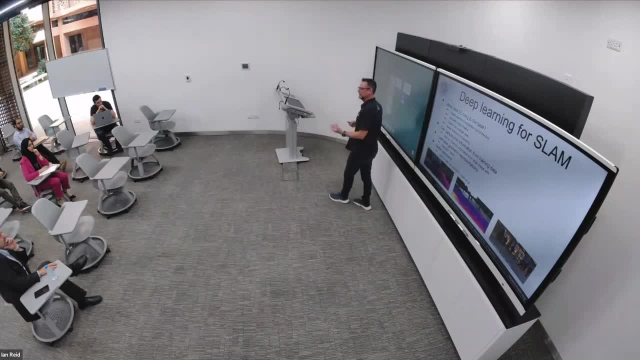 but you may have heard of the algorithm raft that's come out of princeton recurrent or western Feature transform. Both of these ideas are based around the fact that the idea that we already know how to do a bunch of stuff in computer vision And computer vision is often formulated as an optimization problem. 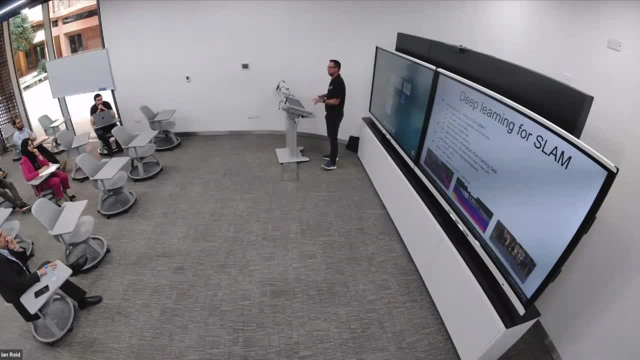 And one of the problems that I see with a modern deep learning approach to computer vision is a tendency, particularly of new students, to pick up latest deep learning algorithm and just say, OK, well, maybe I can do that thing that people used to do in the 1990s in this way. 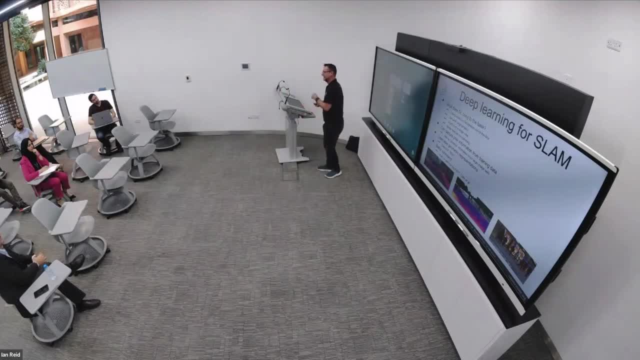 And I can do it with a feed forward neural network And sometimes that works really well. Most of the time it doesn't work really well And unfortunately a lot of students spend an awful lot of time trying to make it work better When I don't think it's the right approach in many circumstances. 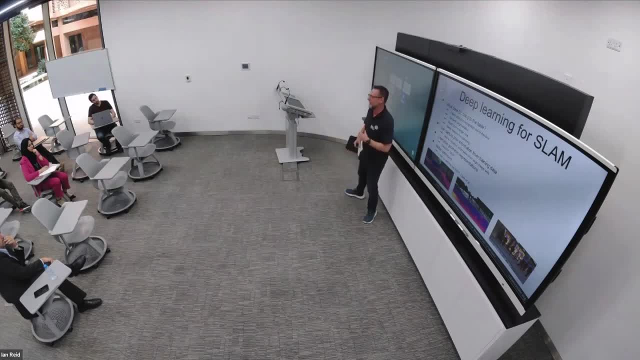 And I think these, these ideas do have a lot of promise, because what they're saying is: we already know how to formulate computer vision problems as as an optimization. Let's use learning to do better optimization. So, rather than learn the solution, let's learn how to update our solution. 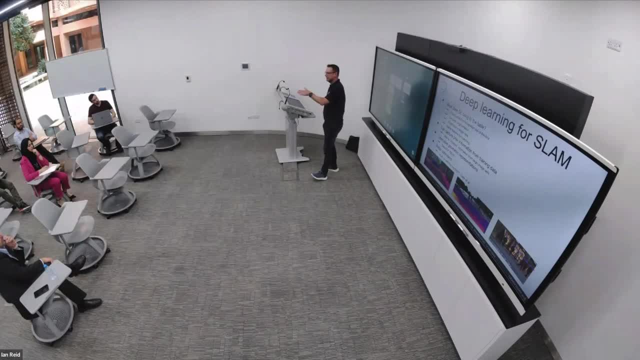 So that, instead of relying on just a gradient that tells us the direction to go, or gradient adhesion that tells us the direction to go, That tells us we're going to approximate our function surface by by, by a quadratic, Let's use a data driven step size. 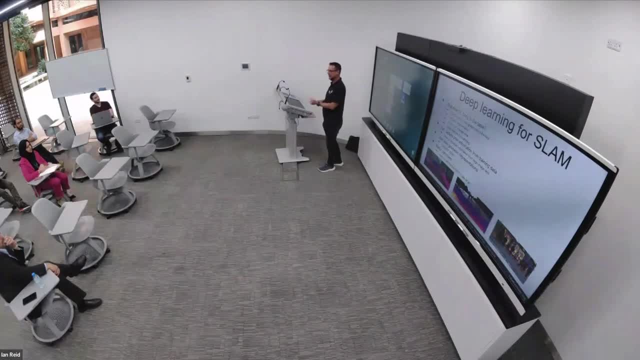 So so we're still optimizing the same function, We're still optimizing the same objective, but we're using deep learning to move us there in a more intelligent way so that we can converge faster. I'm not going to talk about that, but I thought that's a plug for, I guess, the philosophy that I think we should be moving towards in deep learning. 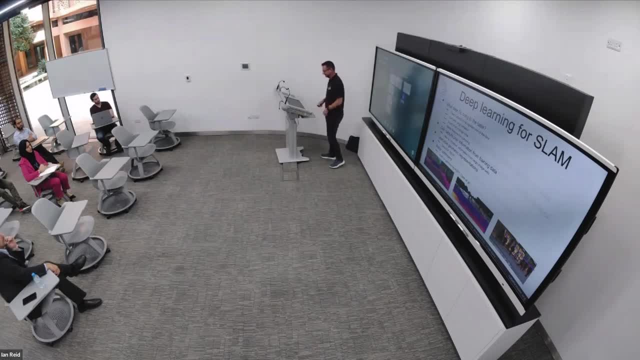 When we already know how to do stuff like geometry. So in this talk I've already used up what 10 minutes of my? a lot of 45, so I'll probably go very fast. I might skip over a whole bunch of things, but I wanted to cover these, these four things. 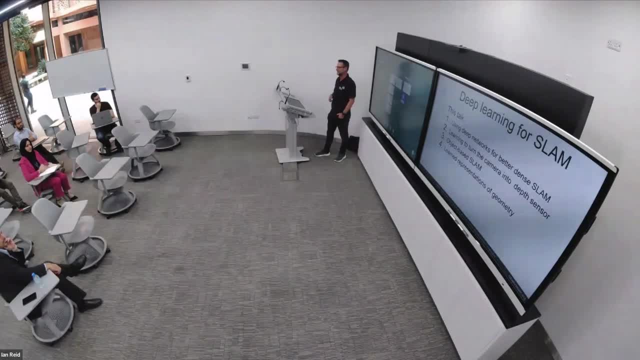 Hopefully not in too superficial detail, but very happy to take questions afterwards. But so I want to talk about just some older work where we're very early work, where we're trying to use deep networks to do better dense slam. Then I want to talk about how we can turn the camera into a depth sensor using learning and, in particular, how we can do that using unsupervised learning. 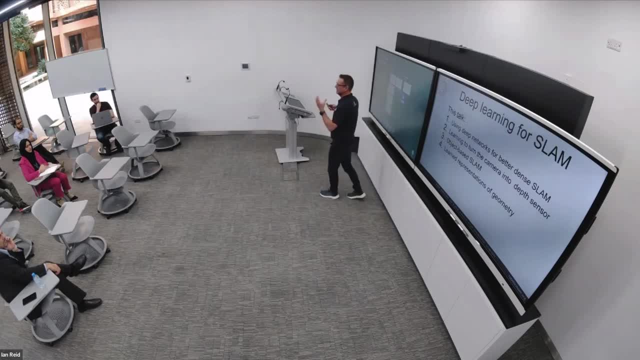 We'll talk a bit about object based slam, so that we move away from this notion of just a point cloud and a camera in the point cloud. And then I'm going to touch on this idea of learned representative, that learned representations of geometry at the end, and show you some work that's happening already. 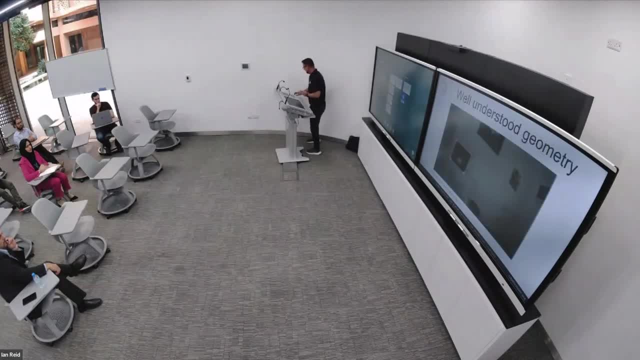 But before deep learning. this is the kind of stuff that that I was working on, So this is some work from the late 2000s, or that started in the early 2000s With Andy Davidson, who's a professor at Imperial College. he was then my postdoc when we started this work in Oxford. 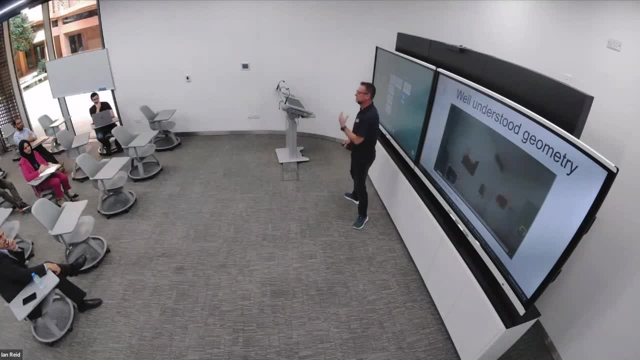 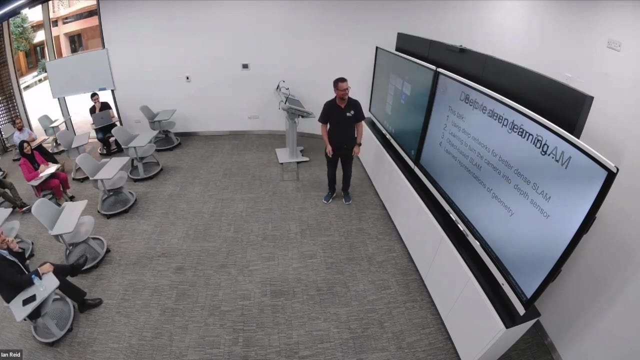 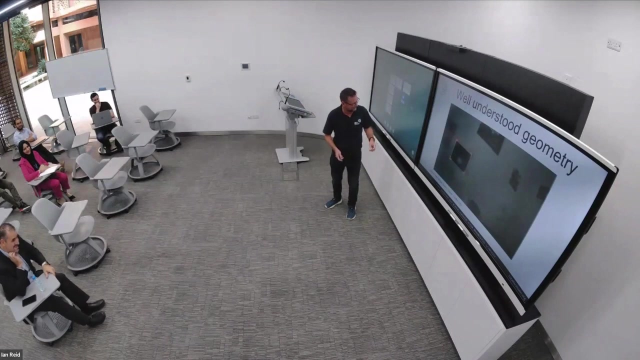 So what you're seeing here Here is the first real time structure from motion slam system And it's detect automatically. Did I touch that? I think I touched that. I'm building technology. I don't like using technology. Okay, So if I do that, 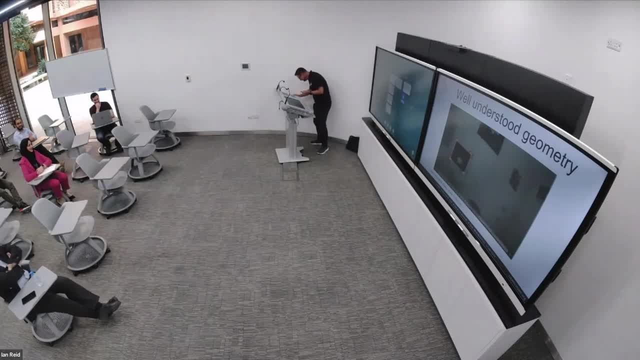 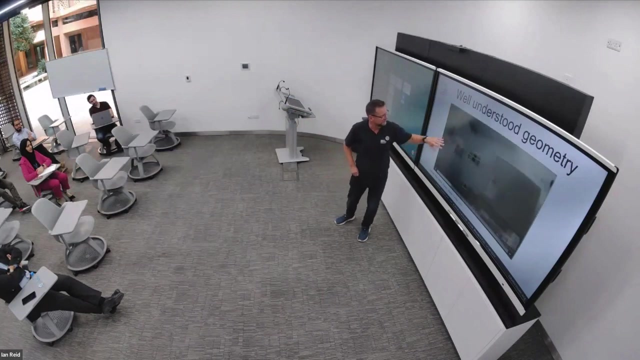 So it wants the mouse to be there. Sorry, I'll put that down so that nothing bad happens. Detecting features automatically- It's a depth- by triangulation and putting them into a map. It's doing. You'll see in a second. 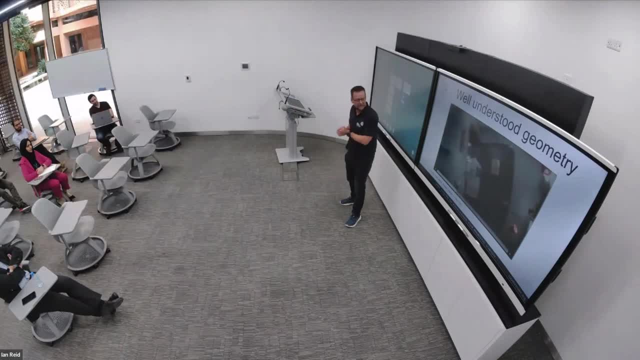 It's doing this active feature search because at the time this was running on very, very limited hardware, And so these circles are actually uncertainty ellipses that are saying we believe that the feature is there. This is happening as part of a common filtering approach. 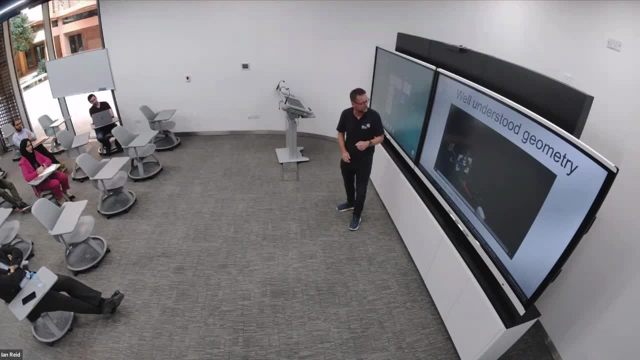 So we make a prediction of where we think the feature should be: to narrow down a search and and then do the matching within that search window. And so you can see here this is the kind of map that 15 years ago we were able to build in real time on fairly limited hardware. 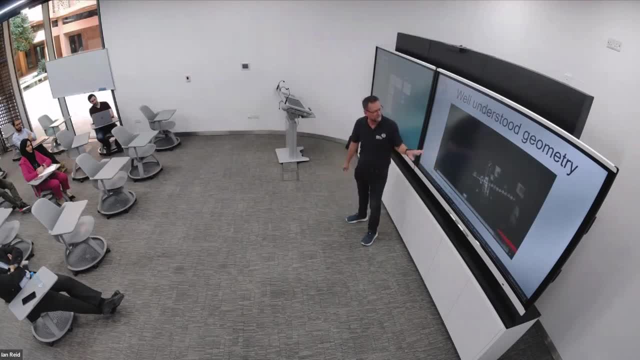 A feature map of around about 30 points And, and you can see that these points are represented by positions and uncertainty ellipses, along with a little patch that says what the feature looks like. I think I'm going to skip over the rest of that. 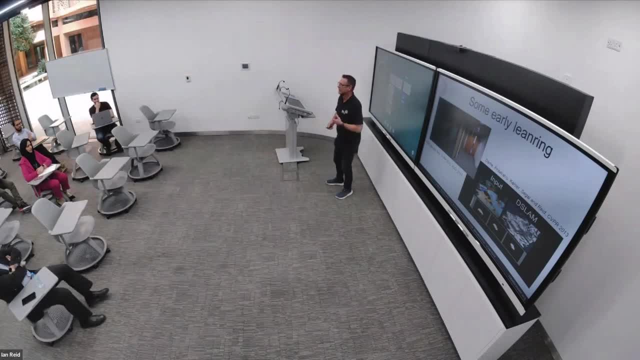 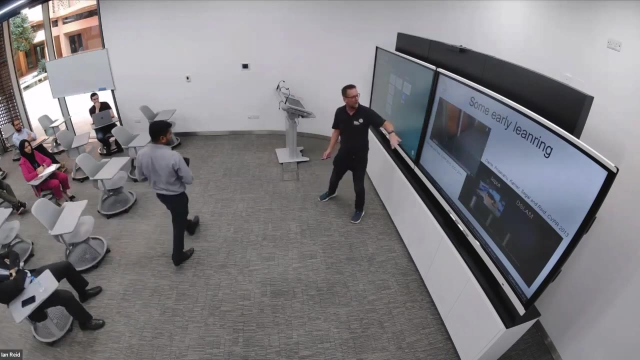 So so we then started to think about going beyond that To some some limited learning, And so this is some work from 2011 with one of my students, Alex Flint, where we said, OK, well, if we can localize the camera, perhaps we can start to do some inference about the stuff in the world. 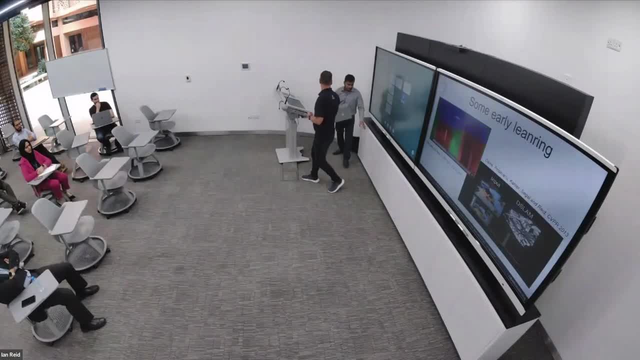 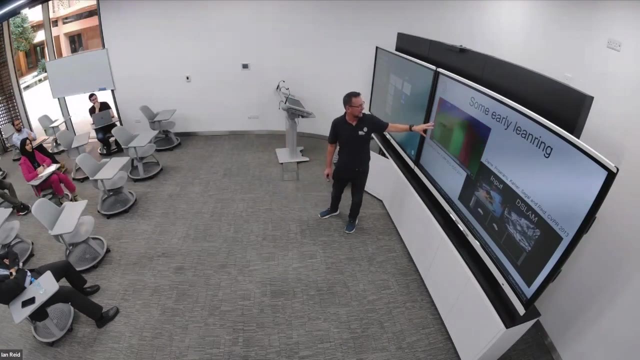 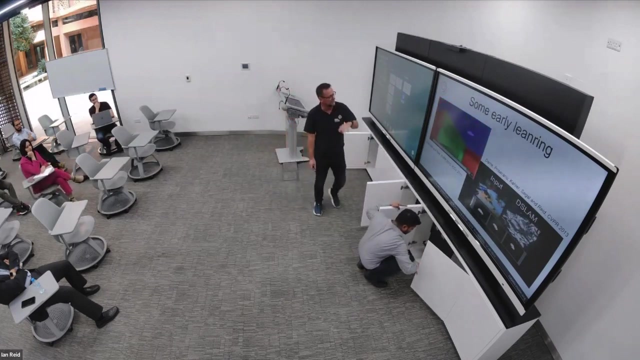 And so, OK, can we pause for a second? It's OK, You can carry on. We're just checking something with the wiring, OK, well, yeah, I'll keep talking. So so what you see here is some. we're using some learning, single view, learning that people at the time were very keen on to augment the, the, the scene that we've extracted. 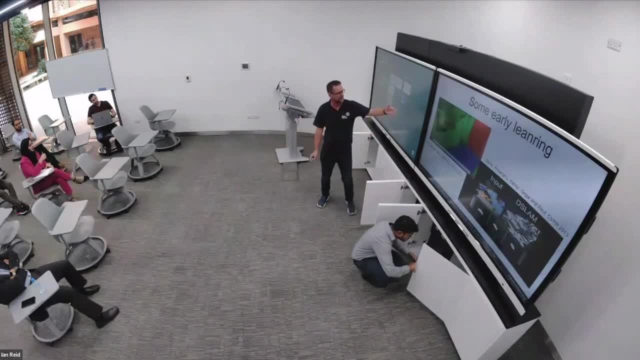 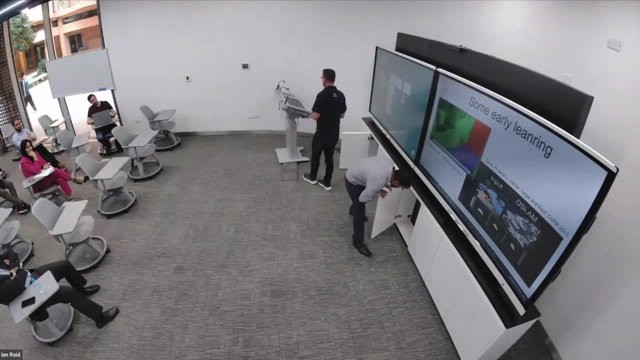 So no longer is this a point cloud. This is something that's telling us where the floor and the walls of the room are, And down on the bottom right, You see that we were able to do things like dense reconstruction and add in object recognition, in this particular case around about 2013.. 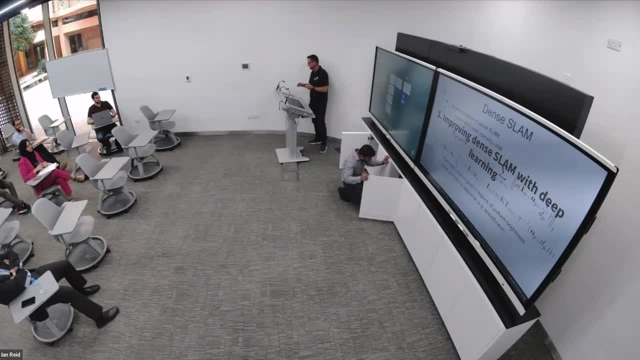 So now I want to talk about how we can improve dense slam with some, some learning, And I guess in the interest of time I'm going to gloss over a lot of the mathematical details. But but this is a fairly standard formulation of dense slab. 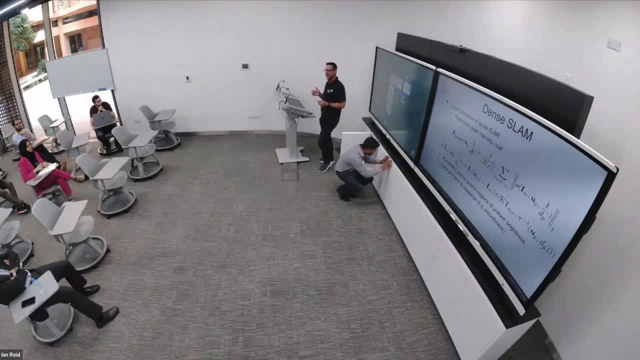 We have a photometric cost, And so, rather than matching individual features That are being extracted from each image, What we're doing is matching a photometric cost that says for every pixel, to optimize the depth at that pixel, And we're going to do so by matching pixel colors effectively. 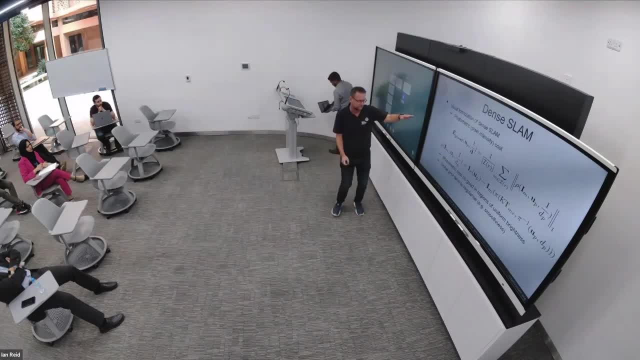 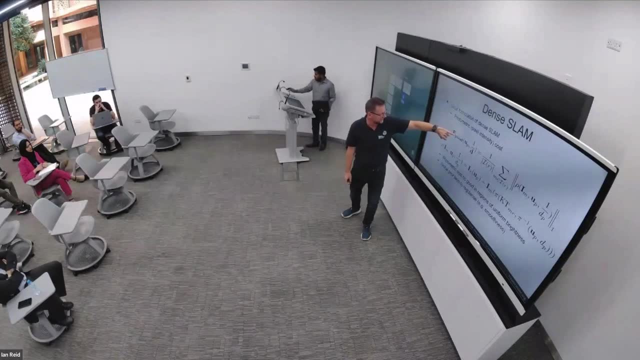 So so that's what you're seeing here. So this is: this is the intensity at a particular pixel, And this is the difference between what we predict the intensity should be, So what the pixel intensity actually is And this is what we predict it should be, by back projecting from a keyframe or from multiple keyframes. 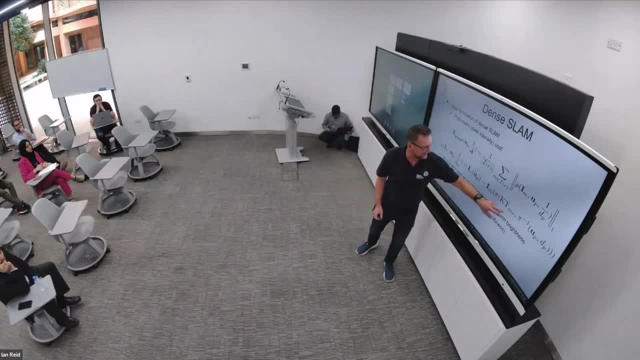 And and then re projecting by the depth that we believe the point to be at and the current pose of the camera, That photometric cost that is basically just looking at. is the brightness of this pixel or the color of this pixel the same over time? 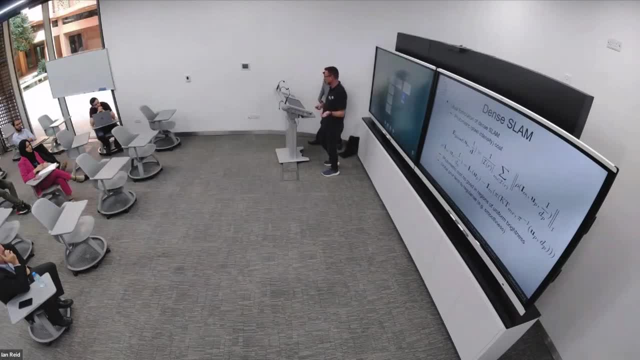 If we've got the depth right. It's no good in regions of uniform brightness, And so what people did previously- So, Richard, you can work with Andy Davidson- produced the first dense slam system And he he had to have a smoothness term in there to say, well, if the photometric cost tells me nothing, then the best I can do is just say it's probably smooth. 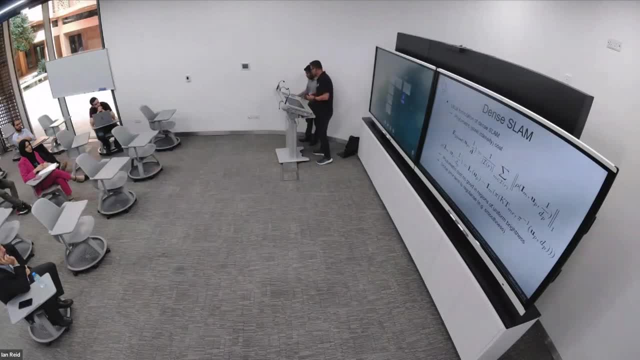 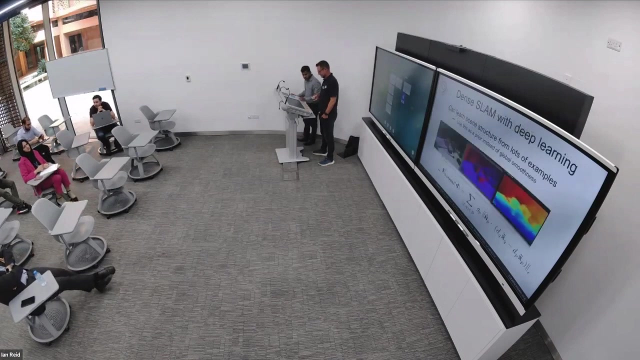 And and that's OK, But it leads to: Yeah, it's a shadow. OK, So I press that. Am I still? Is this still wrong? I have, Oh, I have several questions, OK, First of all, can you show me the size of the last frame? 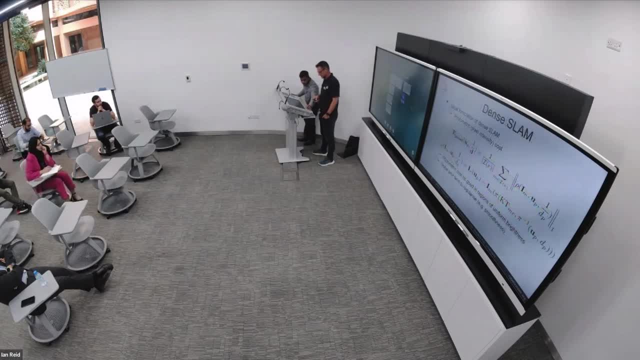 I don't. I don't want to be too brief, I'm just. I'm just going to have to put it in. OK, I'm going to have to put it in. Maybe the how about? You know, I'm. 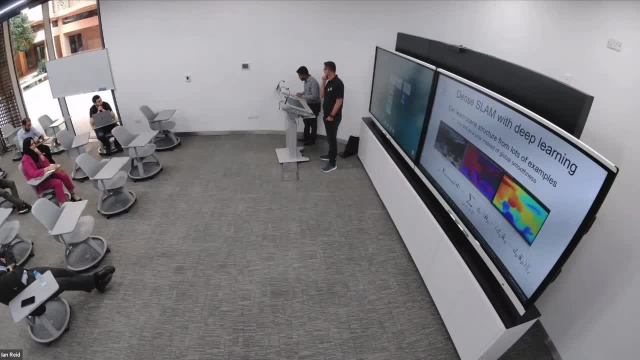 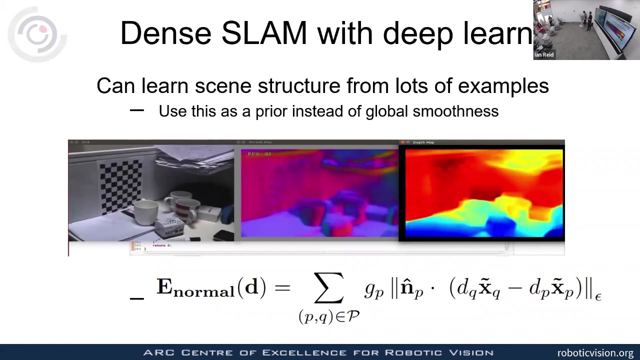 I've got a little bit of time. I know there's a lot of things, But, but So what you're seeing here is the idea that, instead of using global smoothness, which is a pretty generic and not very- How are we doing now? 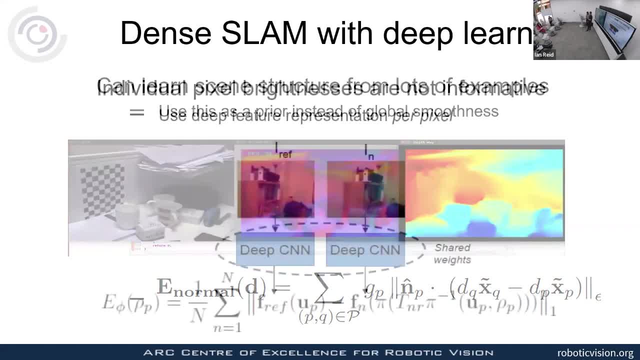 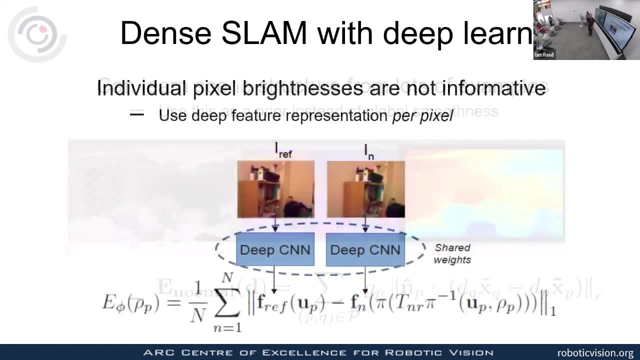 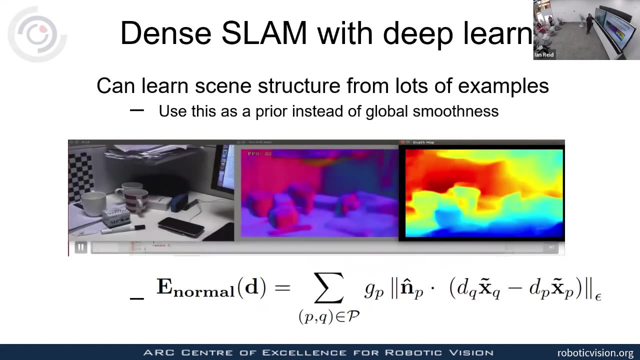 Yeah, Okay, Okay, go on. Sorry, Yeah, Okay, Okay, So I'll carry on. Hopefully you guys can hear me. Oh, what's happening? Yeah, Yeah, Okay. So what? we and I'll talk a little bit more about extracting depth from a single image. 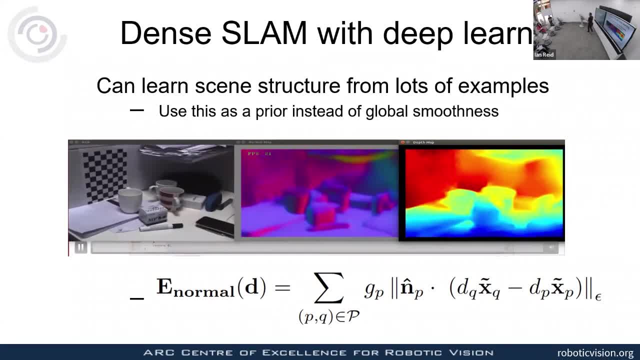 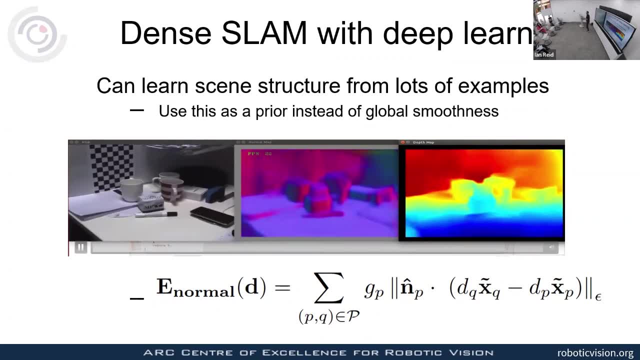 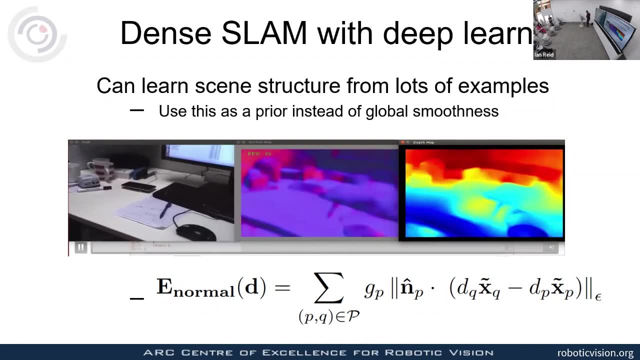 in a bit, but what you see here is we've trained a deep learning network to learn the surface normal, So we're going to use this as a prior for our reconstruction rather than using generic smoothness, And so we introduce an additional term to the energy. 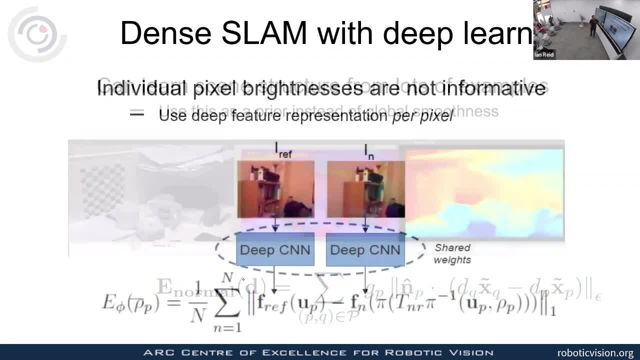 So this energy is dependent on the correct depth of the point. Furthermore, rather than just using the intensity of a pixel, it turns out- and this is true in many applications, including optic flow and so forth- that, rather than using intensity, if you use a deep feature extracted from that particular pixel and its surroundings, 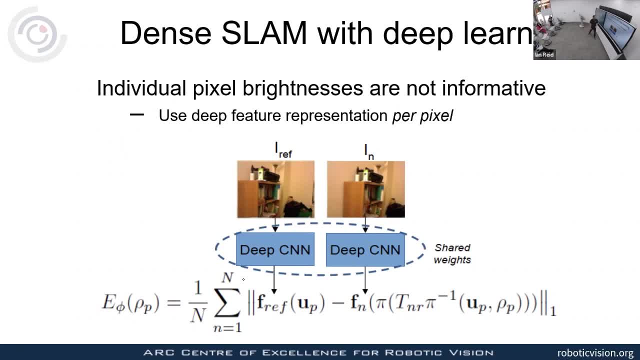 you end up with something that is much more unique to a particular location, And so we can do much better matching using a deep picture represented on a per pixel basis. So we now have an energy term dependent on features, not just on intensities. 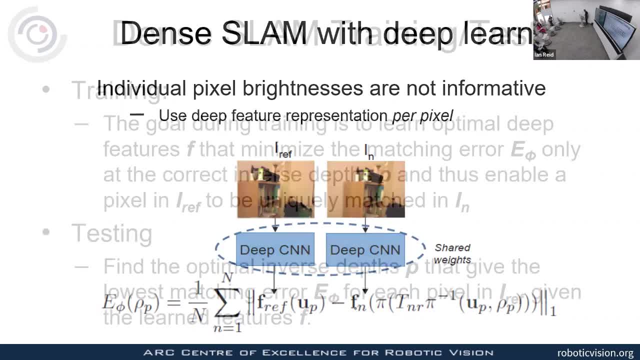 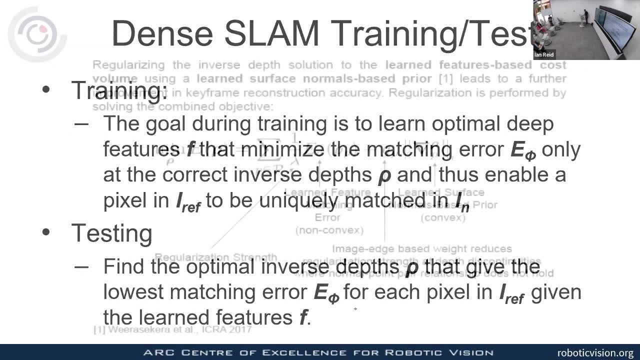 Okay, So I'm not going to go through the detail of training and testing, I'm just going to go through it. Okay, So I'm going to go through the detail of training and testing- and some of this we can do online- and I won't go through the detail of the energy minimization. 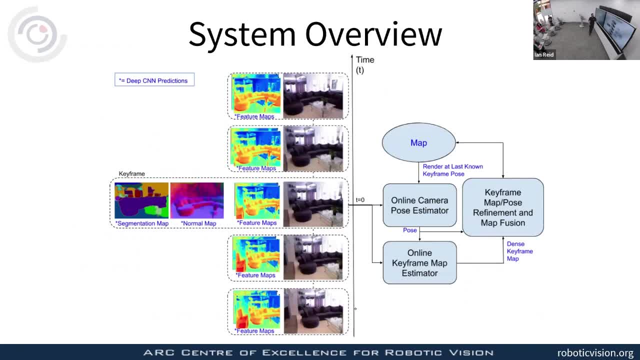 But essentially we have a system now that you feed in. You can feed in a segmentation map or you can compute a segmentation map, you can compute a normal map, you can compute the feature maps of a sequence of images, and they can. 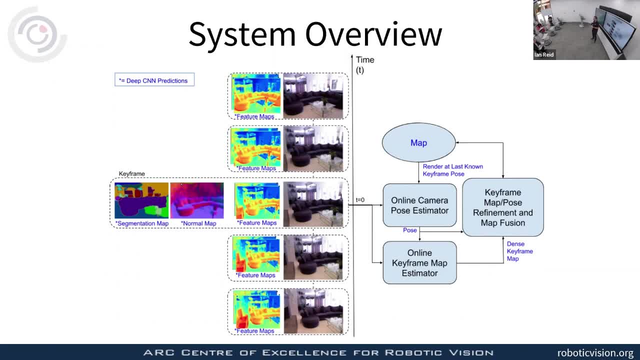 be fed in to do online camera pose estimation as in the standard SLAM, and we can re-render those to do refinement, map fusion and so forth And hopefully next slide you'll see some of the results. I'll show you a video of this in a second. 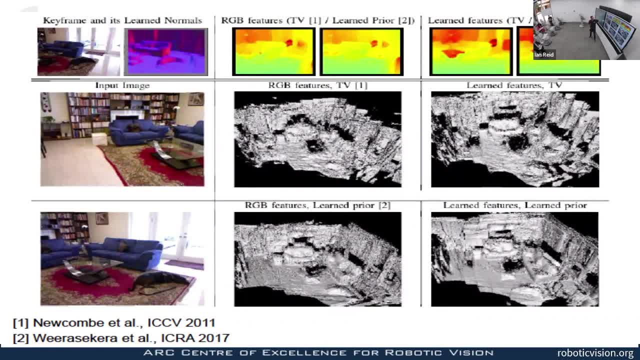 But I just want to compare if we're using, for instance, RGB features. so this is just pure pixel intensity or color and just an ordinary smoothness. So this is the TVL1 smoothness that Richard Newcomb used and we're trying to reconstruct. 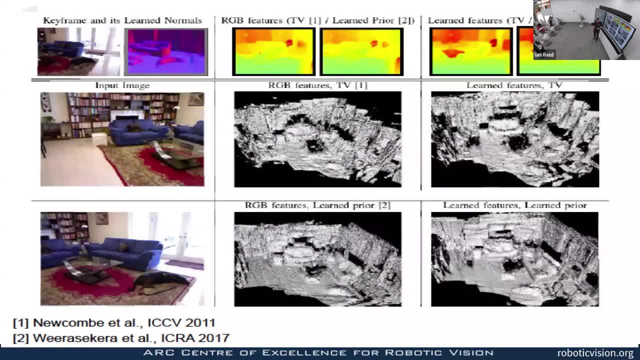 this scene here to get something that's similar. It's fairly noisy. You get something better if you have the learned prior that says I want to regularize according to the surface normal that I automatically extract using a deep network, And if you use the learned features and the learned prior you get something that's much. 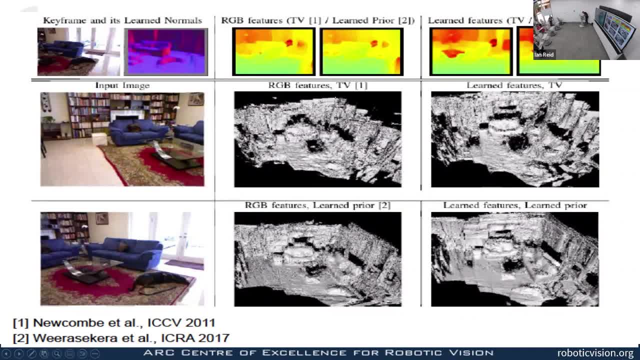 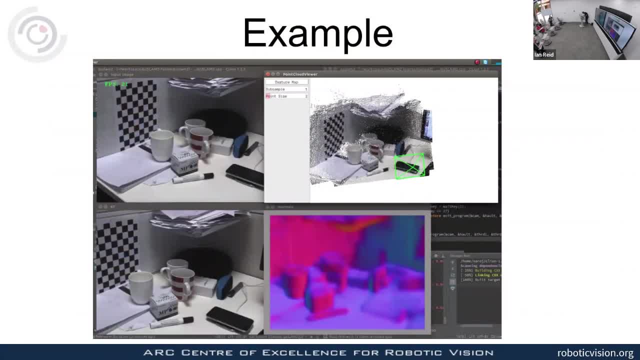 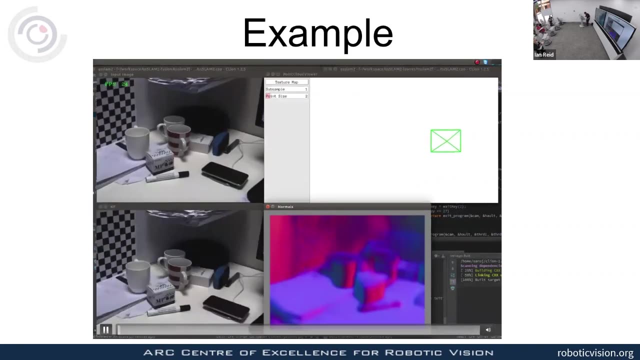 cleaner and that doesn't look as clean as it will in the video. Proceed to this video. Hopefully that is playing, Maybe not. Okay, it is playing now, So original image up here, so this all runs in real time. 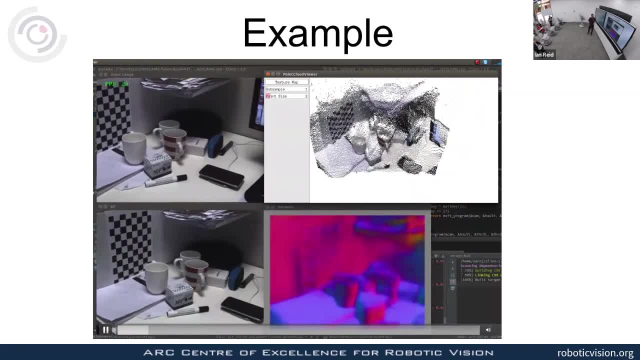 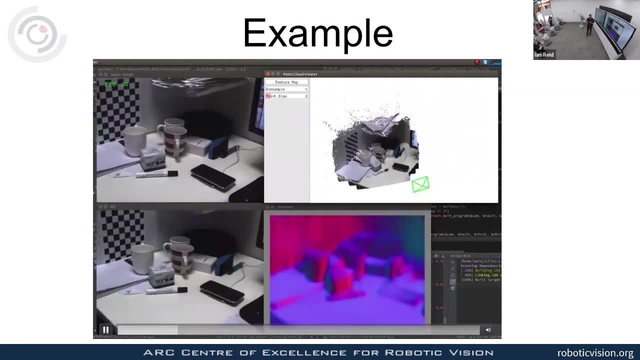 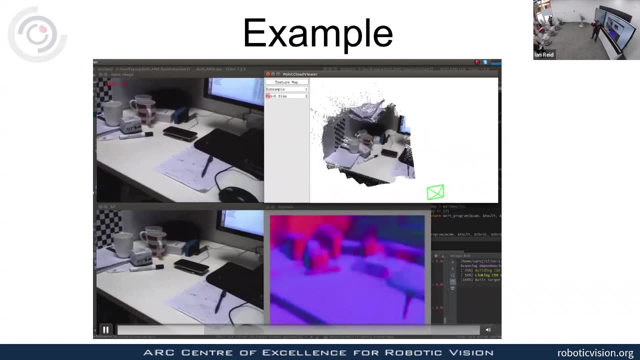 Automatically selected keyframe down here is being displayed as the chosen. What you're seeing here is a real-time extracted surface normal map that's being passed feedforward through a fairly standard AlexNet ResNet18 style map. Okay, And this along with the RGB image and the features that are extracted, the deep features. 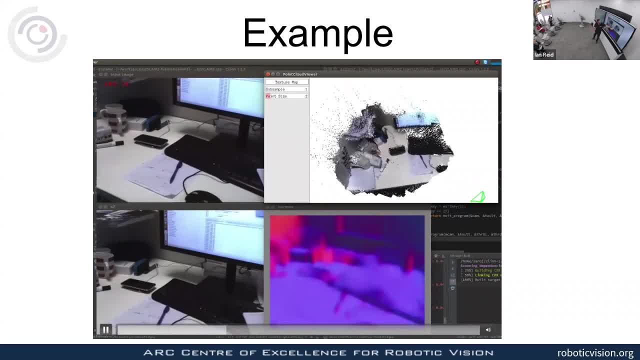 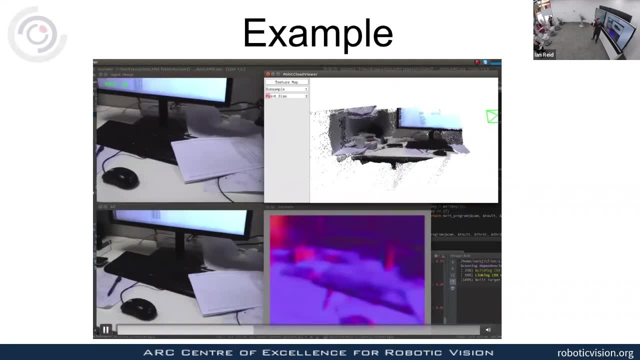 that are automatically extracted go into the energy minimization which is then producing this map up here. I guess the key things to note really about this dense map are that A- it's dense and B- things- like the desk here, which is uniform brightness- would normally be reconstructed. 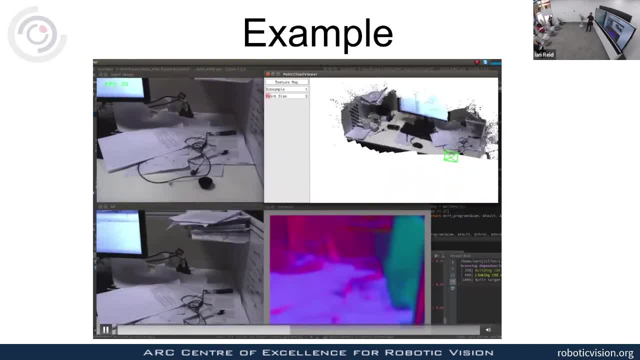 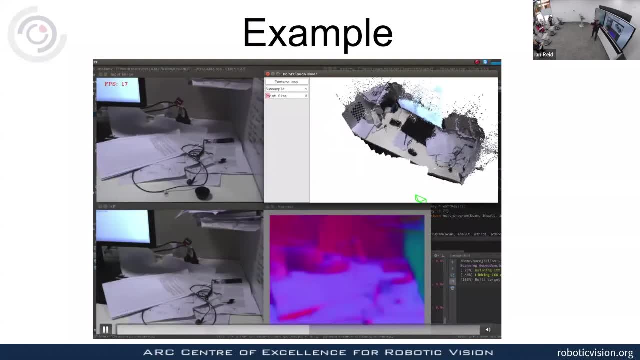 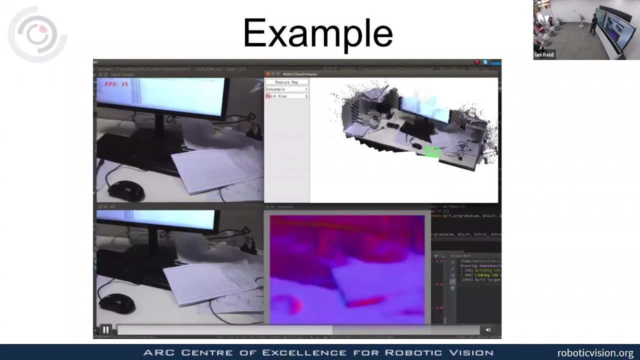 perhaps with curves and waves and so forth, because a smoothness prior doesn't give you the extra constraint that says this is a flat surface, whereas if you've learned that uniform regions tend to be flat via the surface normal, then you can impose that at test time. 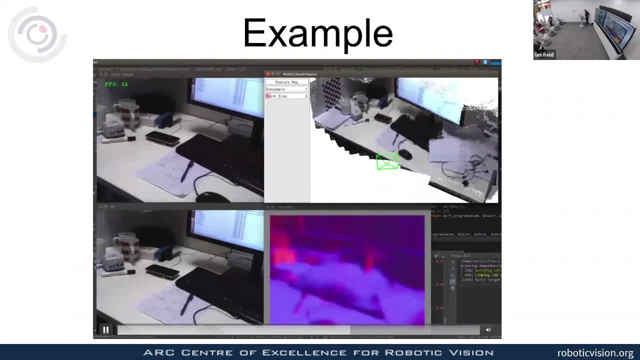 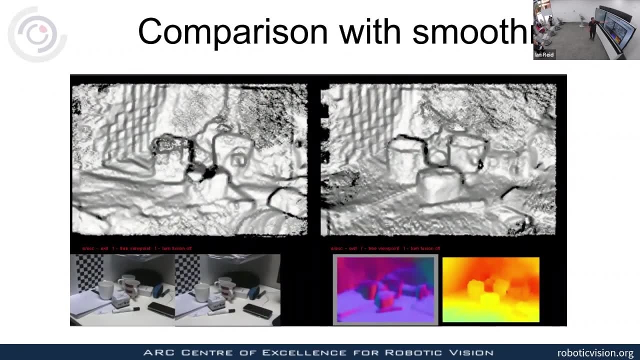 at runtime. So, in particular, you see here a comparison with smoothness and you see which is weak. so this is smoothness. This is using the surface, normal. You can't see that terribly well. Okay, So this is smoothness. 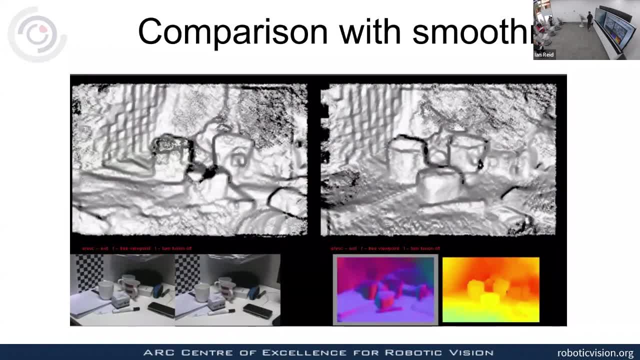 This is normal. You can't see that terribly well, can you? That's an awful image, But what I want you to see is that this is all a bit wavy where it should be flat, and this is much flatter. but you can't really see that because it's a terrible image. 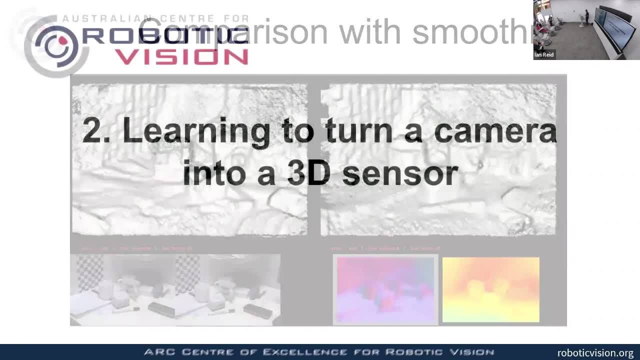 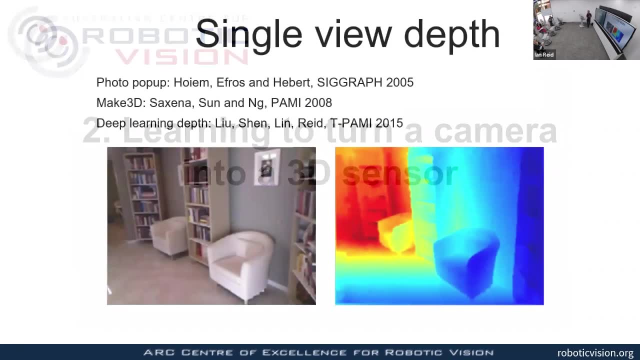 Sorry, But I'm going to move on in the interest of time. So I want to talk about how you can turn a camera into a 3D sensor And, in particular, people have been thinking about this for some time. There's some very early work that Alyosha Efros did, taking a single photograph and turning 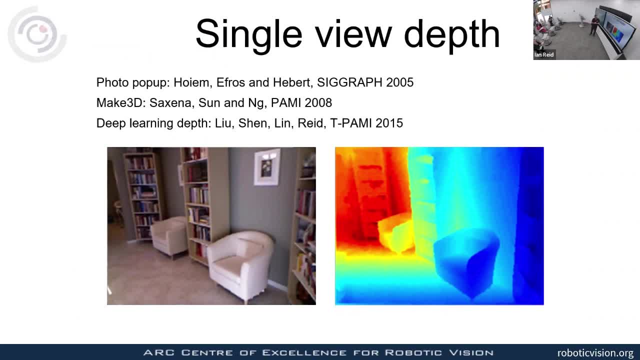 it into a pop-up. Later, Ashutosh Saxena and colleagues did some work called Make3D, where they were using learned features to create a 3D map from a single image, And I guess I was thinking about this and I was very skeptical when I first saw the. 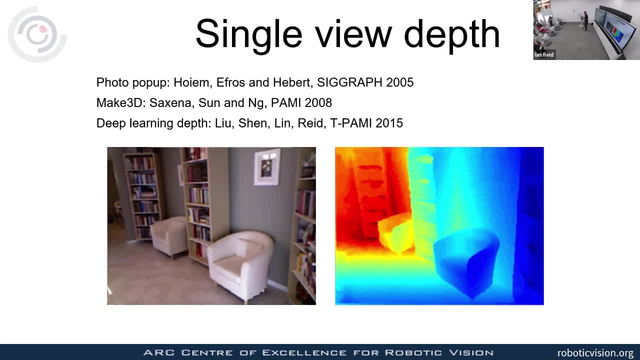 Saxena work. I thought: how can you do this? But actually, if you start to think about it, well, humans can do it. We do it incredibly well. We can look at the 2D image. We can instantly infer 3D, particularly we're good at. the relationship is something further. 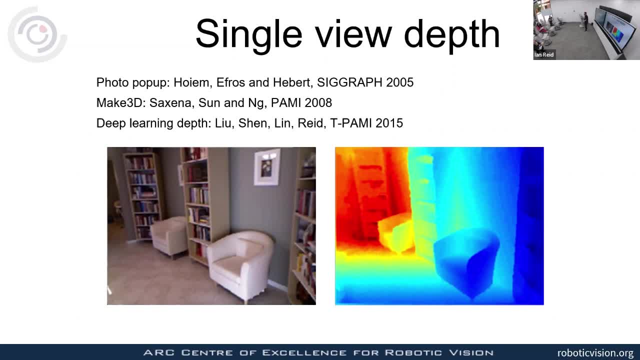 away or closer, And we're using a bunch of cues- cues like scale, cues like vanishing points and vanishing lines and so forth. We're doing that all subliminally, but we are incredibly good at it, And so I guess it was only a matter of time before someone decided to do that in the deep. 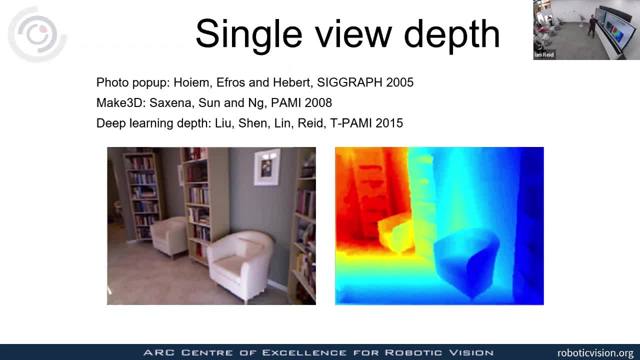 learning era Happened to be a couple of students that I was working with and my colleague, Chun-Maya Shen, And we came up with this system, And it was a pretty clunky neural net system that had a conditional random field sitting on top and so forth. 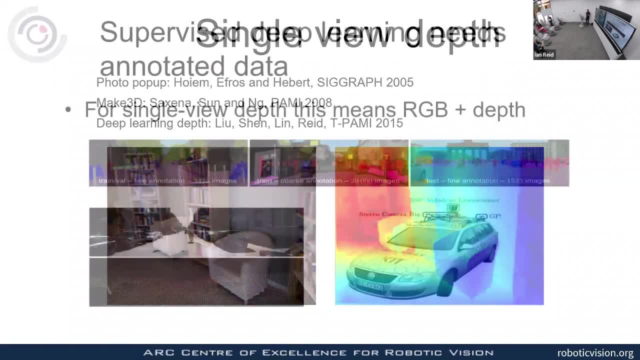 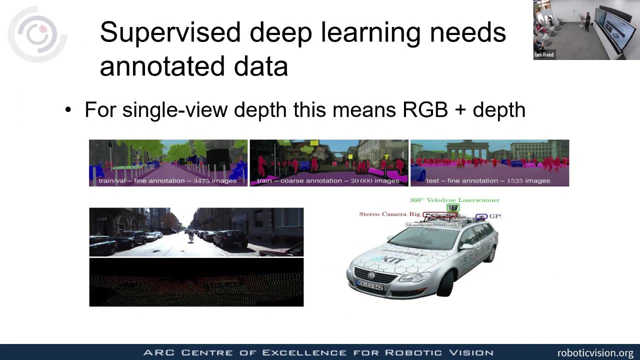 But we started to think about: could we do this better? And one of the problems with trying to turn a camera into a 3D sensor from a single view is the need for training data And, in particular, the training data or the stuff that you saw from Chun-Maya Shen and 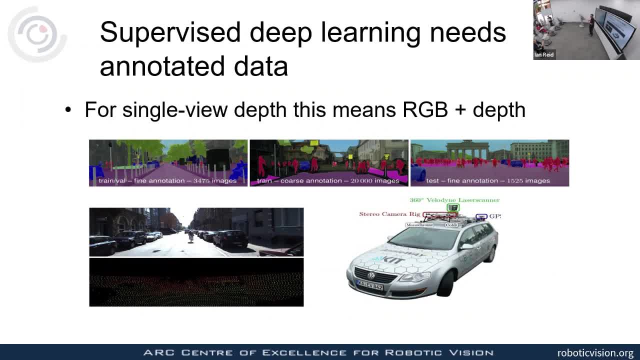 our students was Kinect and a camera. If you want to do that out in the field, you can do that, But it's not the same thing. If you want to do that out in the street, then you go out and you collect loads and 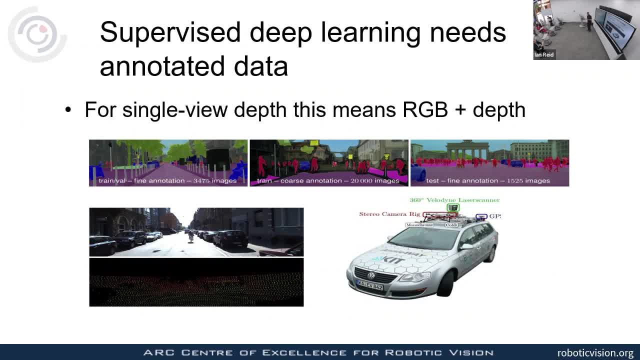 loads of LiDAR data and corresponding images And then you've got a ground truth And you can train your network using ground truth. But that's a costly process And because you need something that's kitted out with synchronized cameras and LiDAR and 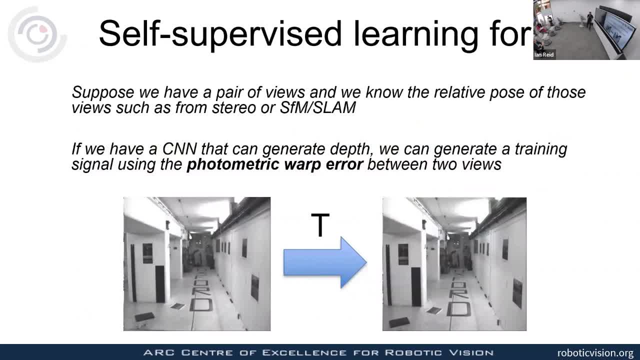 so forth. So my then postdoc, Ravi Garg, had this really beautiful idea that's now being imitated much, But he had the idea first, back in 2015.. And we published it in 2015.. And the idea is this: 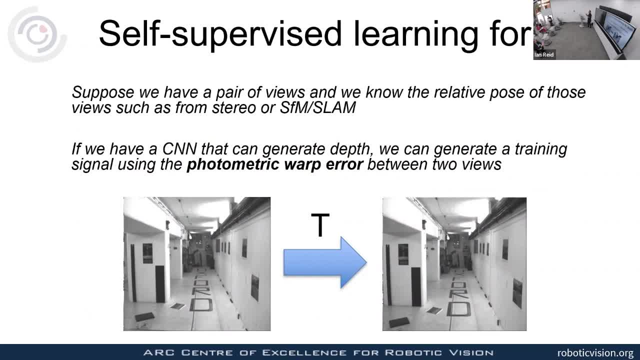 Suppose we have a pair of views and we happen to know the geometric relationship between those two views. In the first instance that could be stereo, But it might be that we're also solving the structure from a motion problem. If we then had something- an oracle, a CNN in our case- that could generate the depth 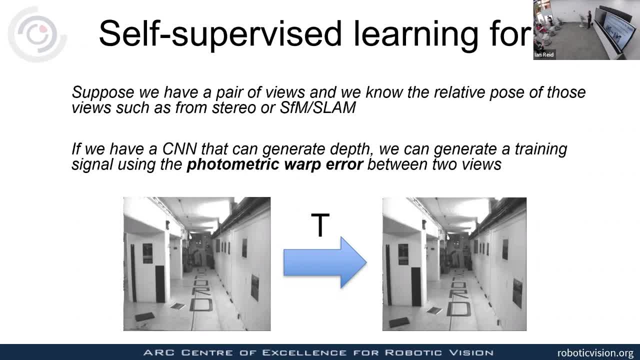 we can generate a training signal using the photometric war para between two views So we can take a A real view And an estimated depth for that real view and a known transformation to generate a synthetic view that should align with another real view. 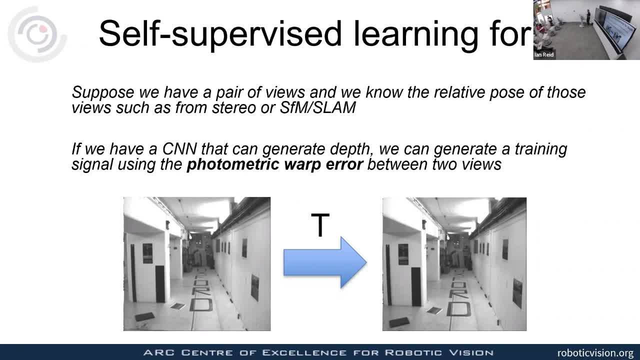 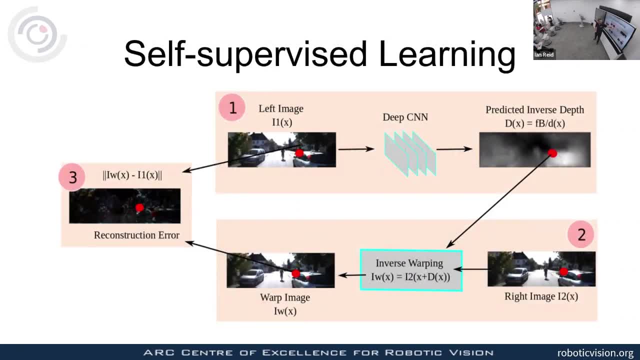 And that gives us a training signal, And that training signal can be used to train a deep network. So that's exactly what we did. We have up here left image, We have a CNN, We predict a depth. In fact, we predicted an inverse depth. 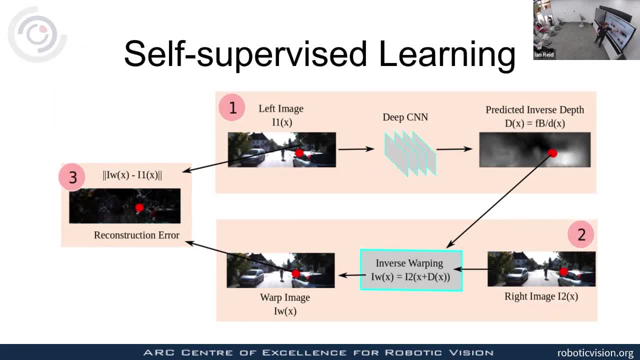 So a disparity, And from that We then, From that we can take a real right image in a stereo pair, walk it back towards what it should look like as viewed from the left, if the depth were right, And we can look at the difference between the warped image and the actual left image. 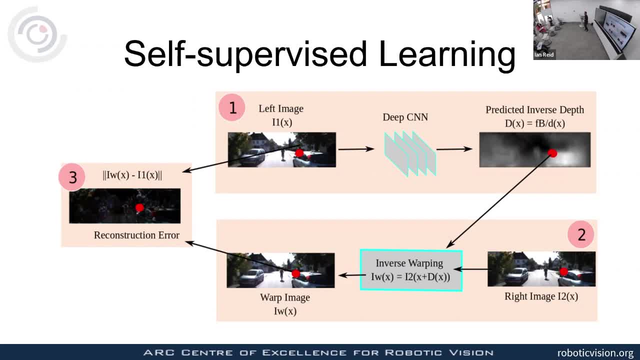 And if there's a difference, that generates a signal that we can then back propagate through our network to train that network. So this is the reconstruction error that becomes the photometric loss for our deep network. So obligatory Picture of a clunky neural net. 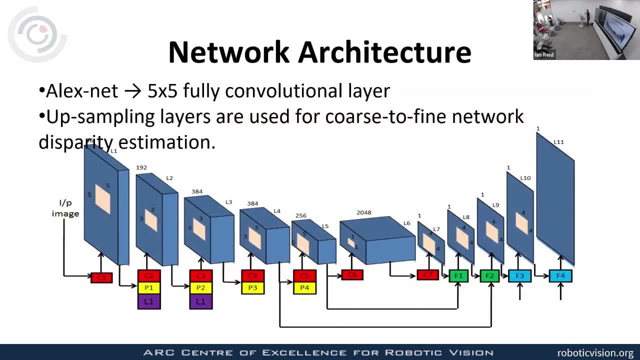 We were using a very simple Alex net type architecture. I had a conversation with with Rich Bowden, who's at University of Surrey, about four or five months ago. He's just completed a survey of all of this self supervised single view depth work. 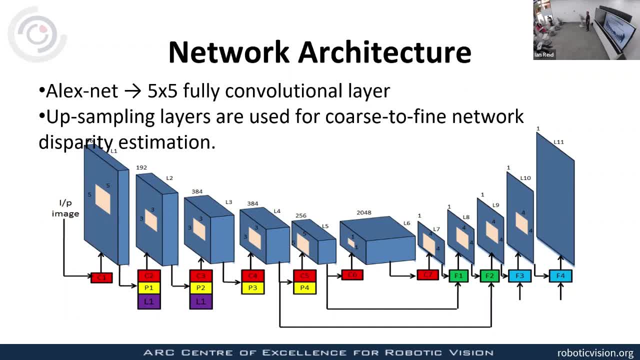 And he said: actually your method works as well as any of the ones that have been published subsequently If you use an up to date architecture. So this is using a really clunky architecture And there's lots of work being published subsequently. 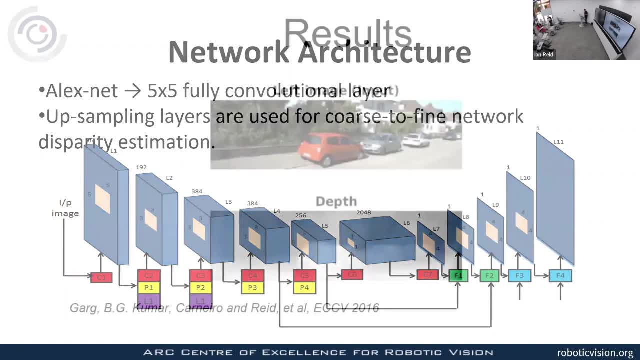 So we can do this, We can do this And then subsequently say we can do something better. It turns out mostly down to the architecture. So this is the early results that that Raleigh was able to generate. Again, so this is from 2016.. 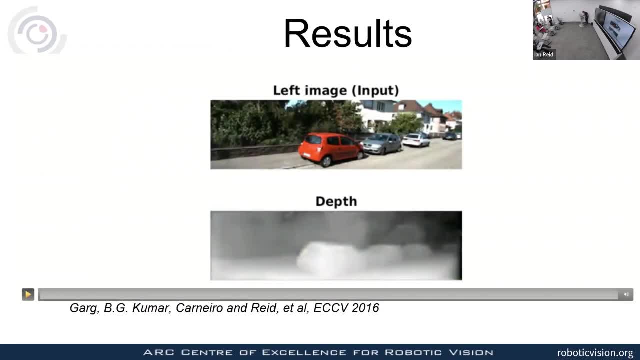 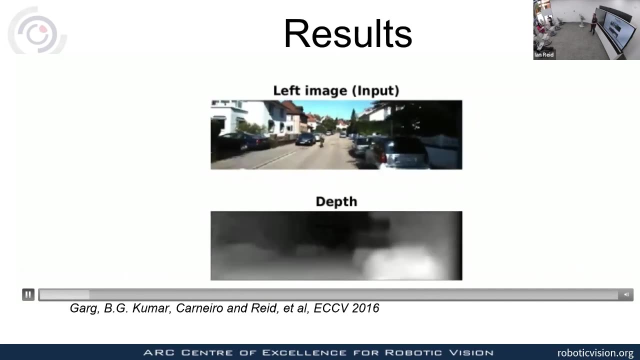 So this is the input to the neural network, And what you see down the bottom is the depth that's been predicted in a single feed forward. pass through the network. where light is closer to you, Darker is further away. So this is the depth that's been predicted in a single feed forward. pass through the 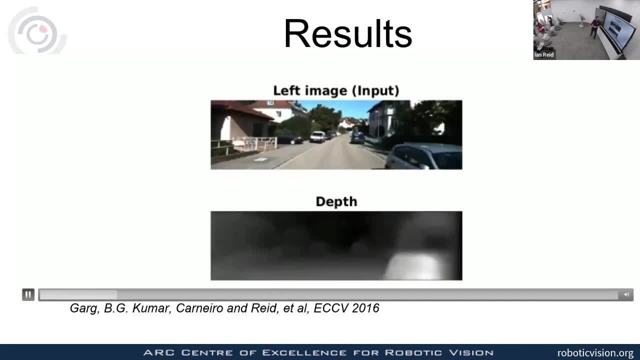 network Again. light is closer to you, Darker is further away, And so I thought it was really quite remarkable that we were able to learn. for instance, as you see the pedestrians walking across here, you can actually see them being extracted. 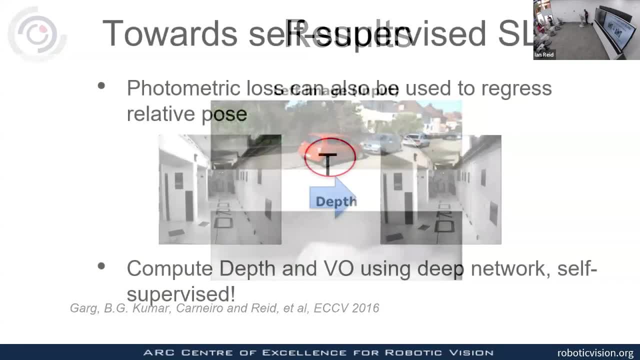 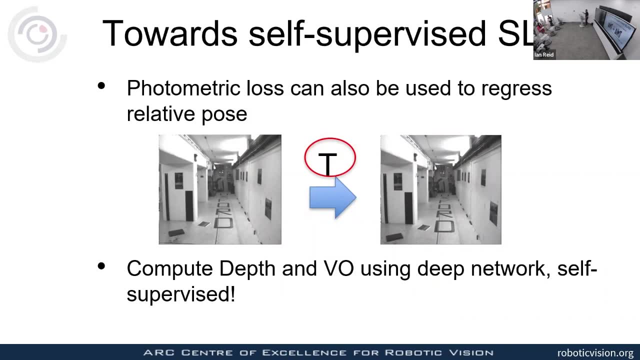 in the depth map as well. So then, we've moved one step beyond that to say, well, if we're doing a slam and we know the relative pose between camera one and camera two, This is where we're doing slam- We can do the same thing. 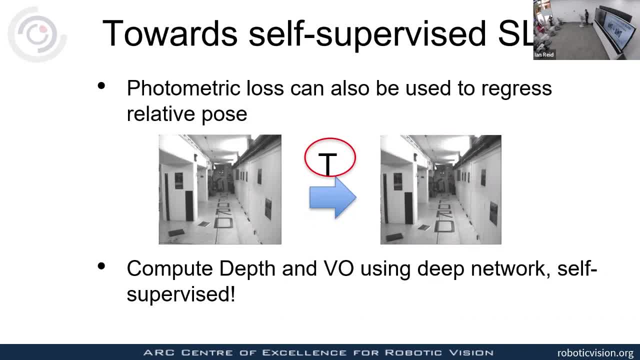 Instead of being a stereo pair, this can now be a single camera moving through the environment And we can compute depth. We could even compute visual odometry just using a feed forward network. It turns out to be a really bad idea, but that's what we did in this particular example. 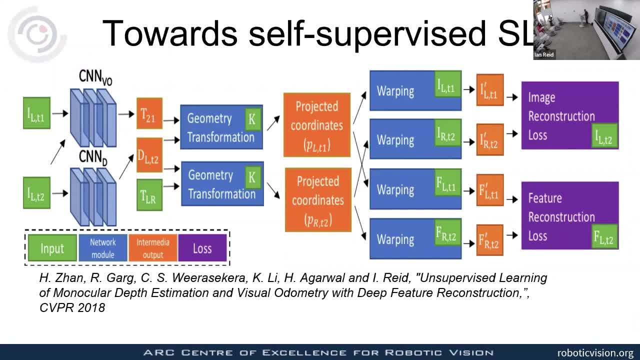 And again, I'm not going to go through and bore you with the detail of this block diagram, but the basic idea is the same, except that now we've got a single camera moving through the environment And the photometric loss comes from the combination of a single camera moving through the environment. 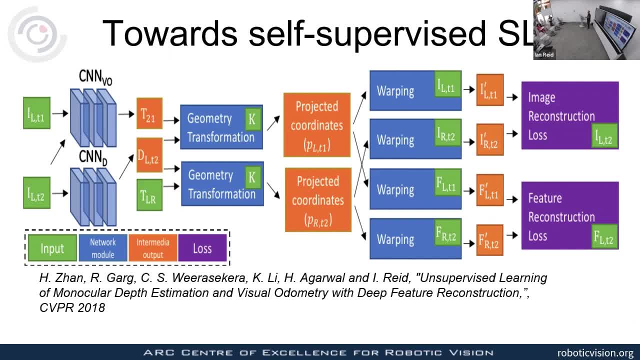 and the photographic loss. If you look at that, we can see that the photometric loss is due to the error that we have in estimating the relative pose and the error that we have in estimating the depth. But it turns out that there's still a strong enough signal that we can regularize both. 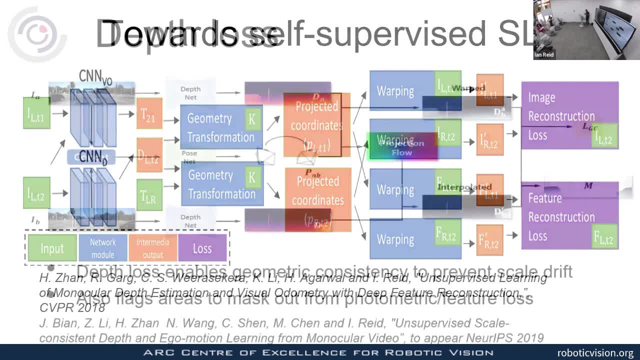 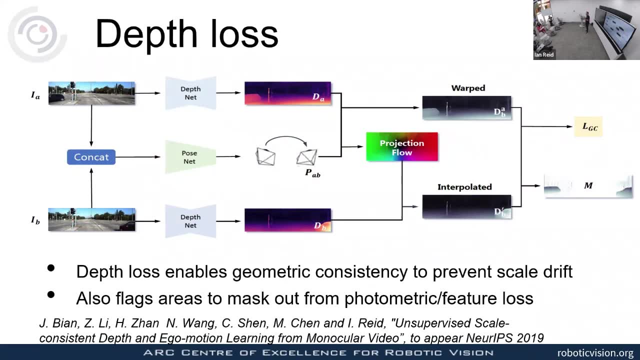 of those. And then there are further things that we can do. We can look at not just if we're looking at a sequence, we can look not just at the photometric loss, but we can also look at the depth loss. We expect that images, depth maps that are predicted at time t should be basically the 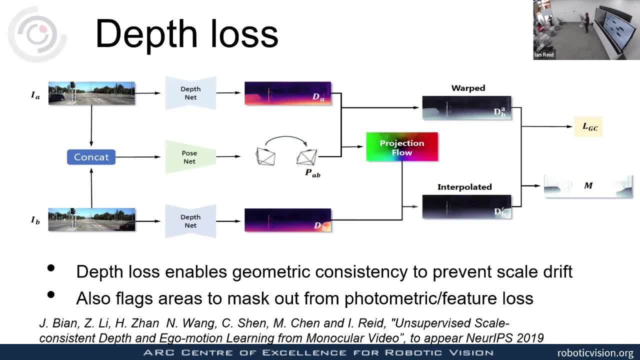 same as, or completely alignable with, image depth maps that we create at time, t plus one- and and if we do that, then we can regularize issues such as scale, drift and so forth, um, and so that's some some work that my student, joanne bian, did um, so this depth loss enables 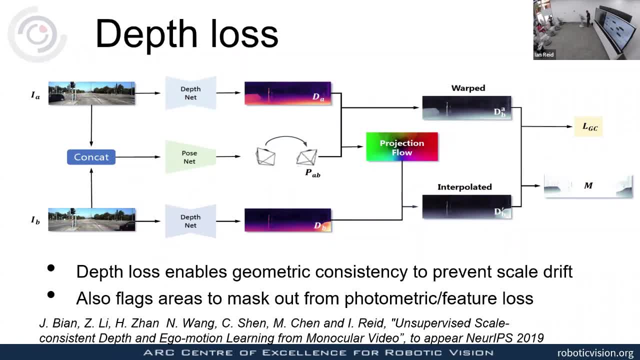 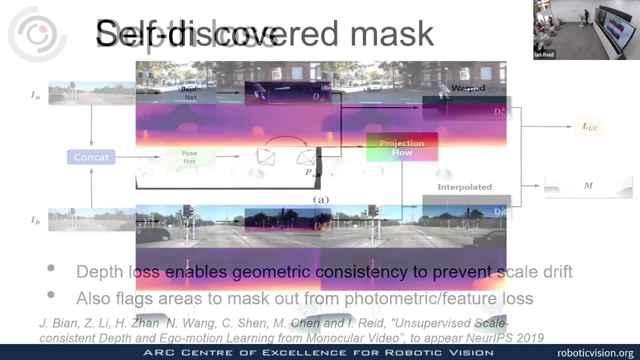 geometric consistency to prevent scale changes between between images. it also automatically enables us to flag moving regions, because the moving regions are inconsistent with the geometry that's predicted in the in the two views, so we can mask them out. um and uh. that can help mitigate drift of the network as, as we're learning so, it creates these self-discovered. 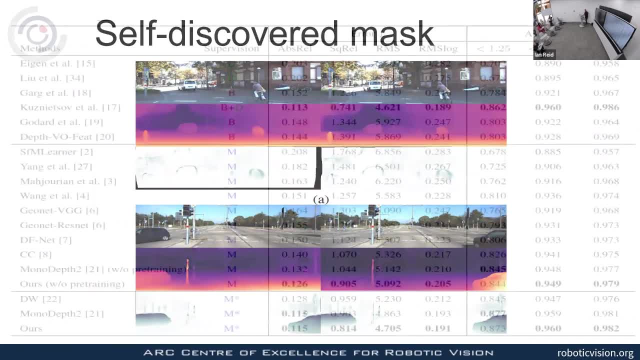 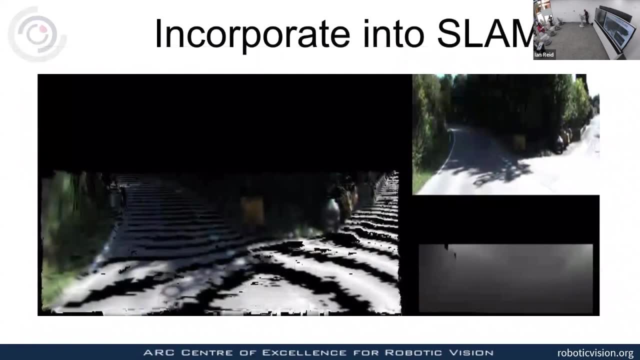 masks of places that are good to learn. again, there's some bold numbers. go and read the paper if you want to see bold numbers. they're all a bit small in these slides. um, nicer to see a video, but even this video isn't particularly interesting. this is really just saying okay. 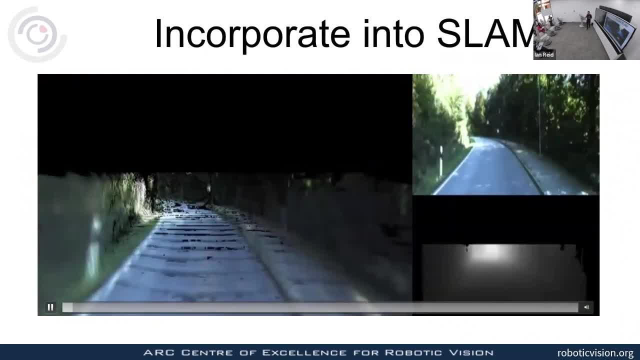 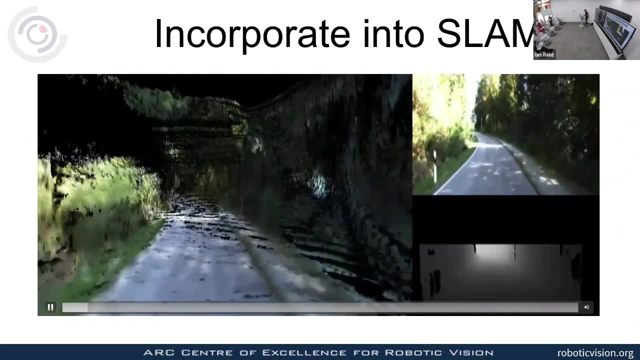 well, we're generating some, um, some depth map for our images, so we're going to go ahead and align them up from a single view and if we align those depth maps, then we can create a fly through of the environment that we're moving through. um, there are still some issues. 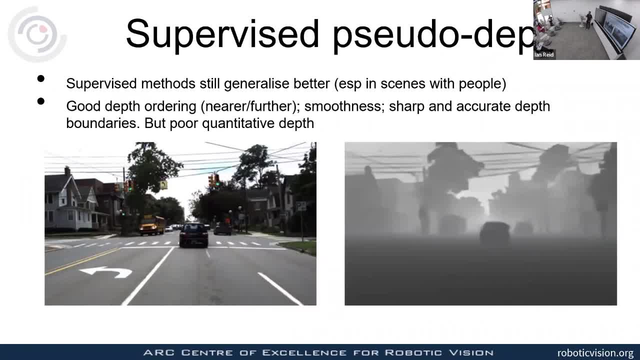 with with that um, and subsequently people have come up with supervised methods for estimating depth for a single camera that are significantly better in a qualitative sense. we're not very good at finding the depth boundaries between object, particularly where there are moving objects in the scene. uh, we're not very good at enforcing smoothness across objects. we're 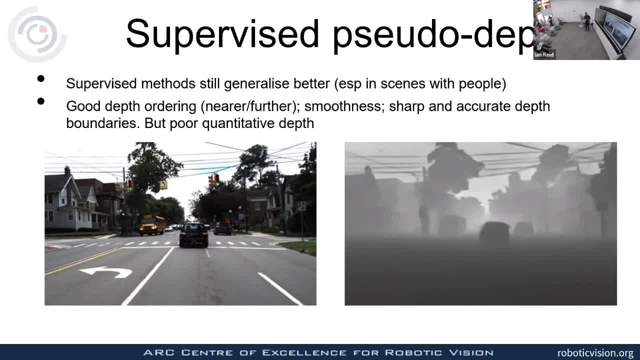 and the supervised methods, particularly this method that my colleague Chunhua Shen and his students came up with for doing what we're calling pseudo-depth, was very good at qualitative depth was very good at getting the ordering correct, So you can see here same kind of false colouring. 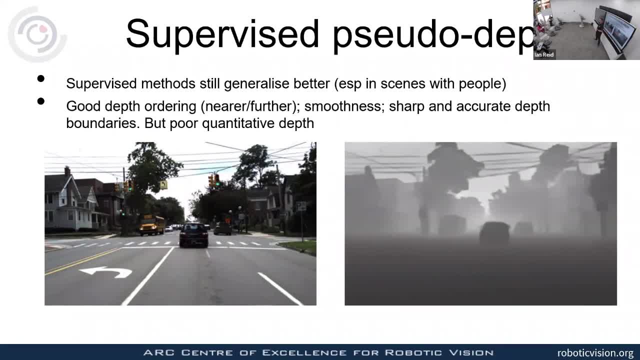 things that are closer in this case are darker. things that are lighter are further away. The actual accuracy of this as a depth map is pretty poor, but actually it's very good at getting the depth ordering right. Closer things are darker than the things that are further away. again. 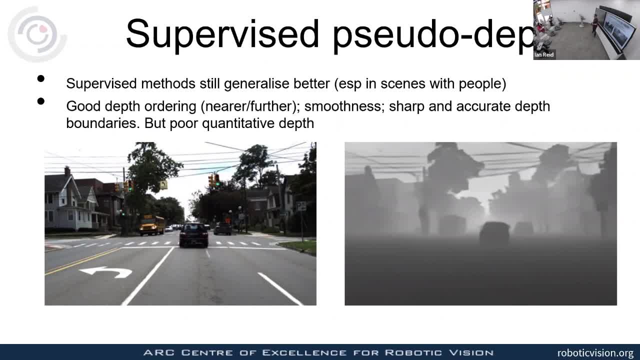 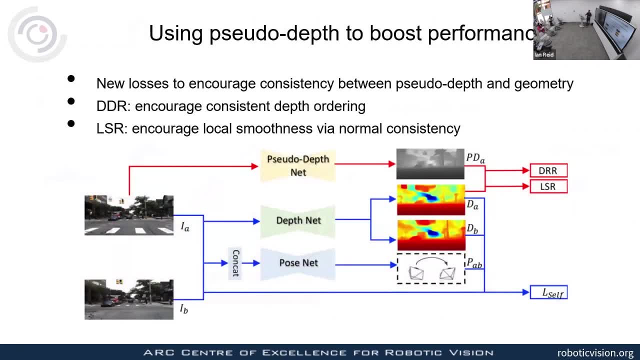 It's also very good at smoothness, sharp and accurate depth boundaries, but, as I said, poor quantitative depth. So Zhouen had the idea that we would use that as an additional loss to regularise a self-supervised system. So you learn your pseudo-depth and you can learn that from a massive data set. 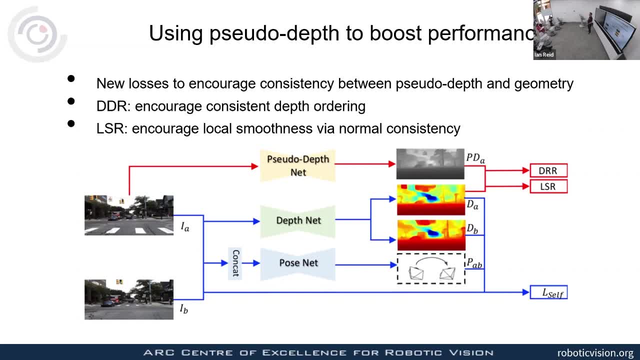 and it just sits there as an oracle saying, yes, you've got the depth Ordering right or no, you've got the depth ordering wrong, And you build that into a loss function or two additional loss functions. here the dynamic region thing, which encourages a consistent depth ordering. 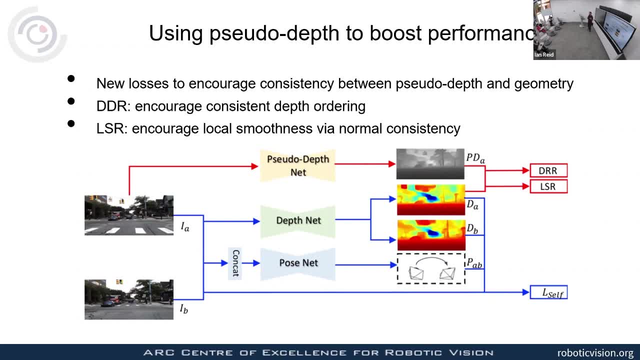 And this local smoothness that encourages local smoothness by looking at the relative surface normals that are predicted both by the pseudo-depth and by the network that Zhouen is trying to create, And you can learn in an end-to-end fashion. well, so this is an oracle that think of it as being a teacher that says: 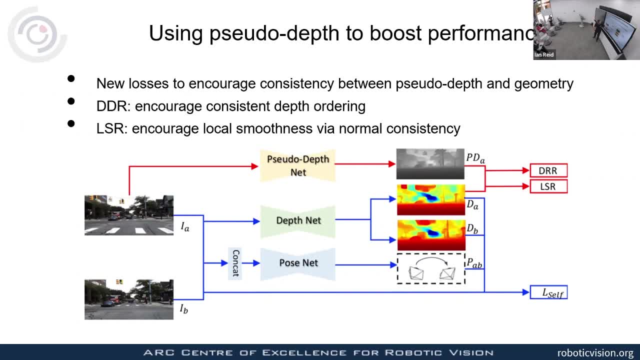 yeah, you've got the depth ordering right. You've got the depth ordering wrong. And these are the two networks that we're trying to learn- the depth net and the pose net- And it turns out that that gives you no degradation in your ability to estimate quantitative depth in static scenes. 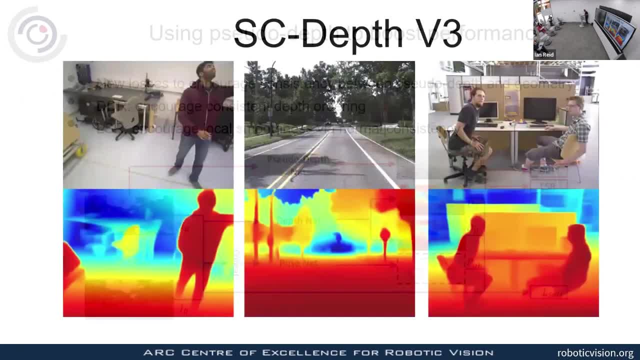 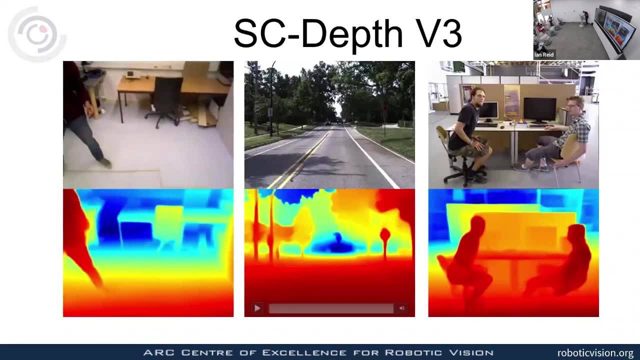 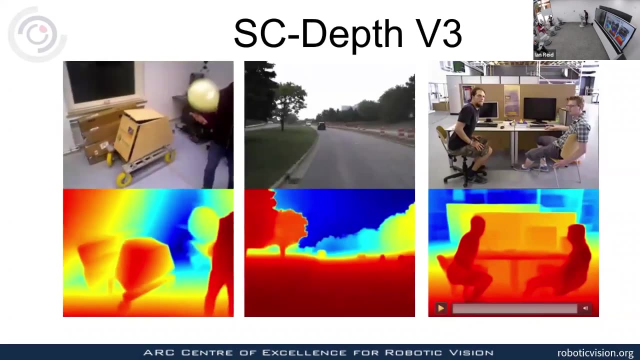 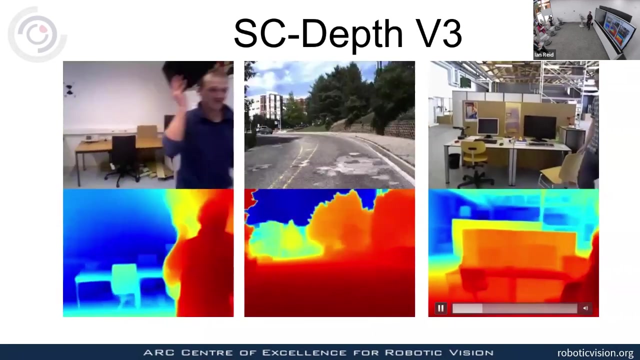 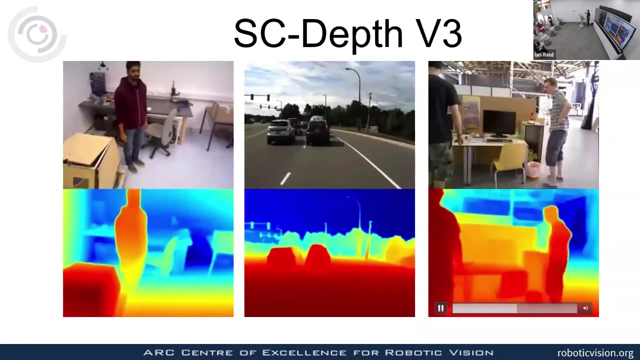 but does a whole lot better on dynamic scenes. So here's some examples that Zhouen has produced. And again, this is: this is false colouring. dark red in this instance means very close and dark blue means very far away. So this is now approaching the kind of accuracy that you can get from very, very strongly supervised networks with massive, massive data sets. 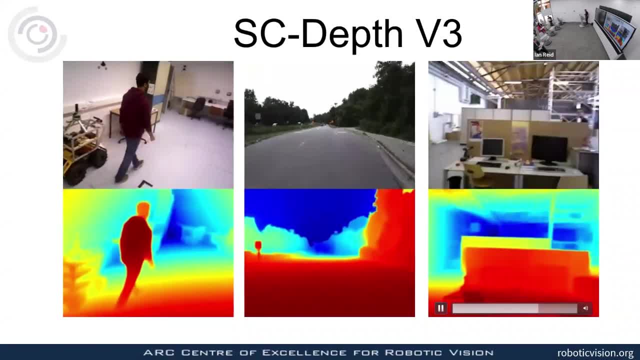 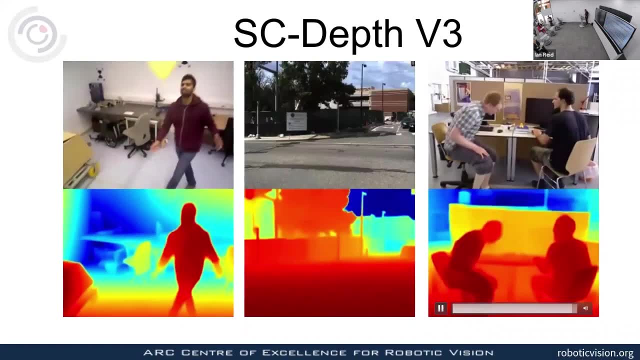 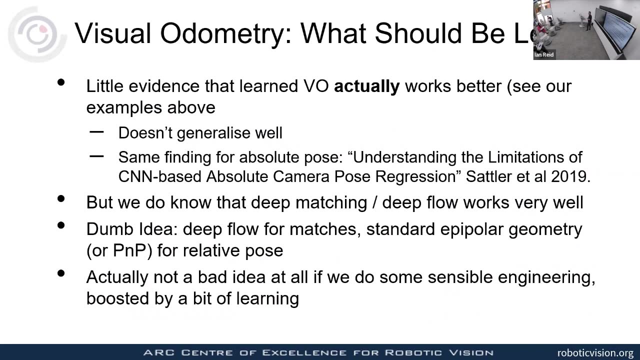 but has the ability to continue to learn Over time. Again, in the interest of time, I'll skip over So one of the questions I posed at the start, or I didn't pose as a question I just said- I'm not sure we're using deep learning in the right way in some of these 3D vision problems. 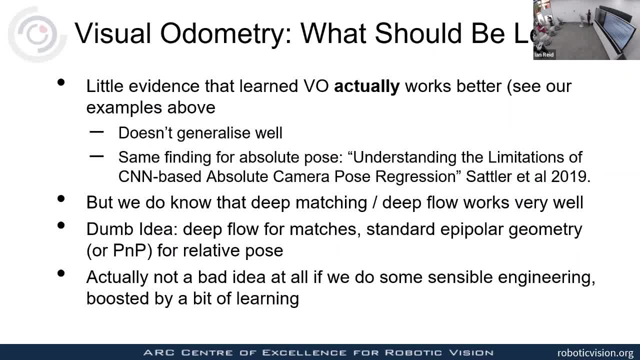 And one of the things we wanted to think about was is learning visual odometry, as we were in that previous example, and a number of other people tried to do the right thing to do, And I'm pretty convinced it's not the right thing to do. 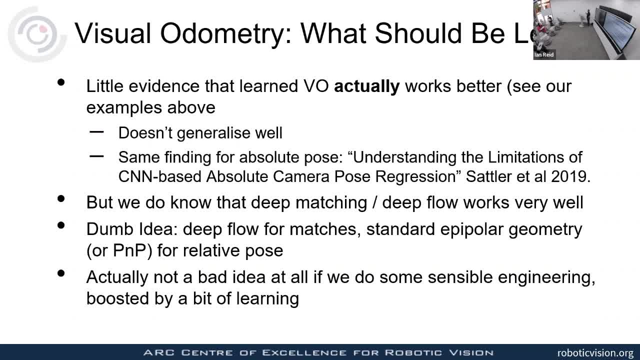 And in fact there's. there's some, some work from Torsten Sattler where they looked at estimating camera pose using a convolutional neural network And said, actually it's a bit, it doesn't work very well. 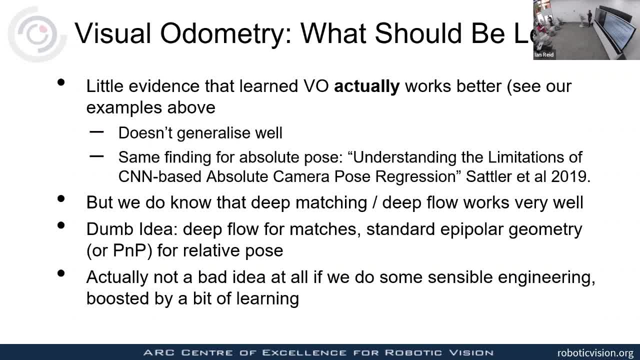 And and likewise the visual odometry turns out that it doesn't generalise very well. It doesn't work that well. We've not been able to do better with with a deep learning approach directly applied directly to visual odometry. it doesn't work that well We've not been able to do better with with a deep learning approach directly applied directly to visual odometry. 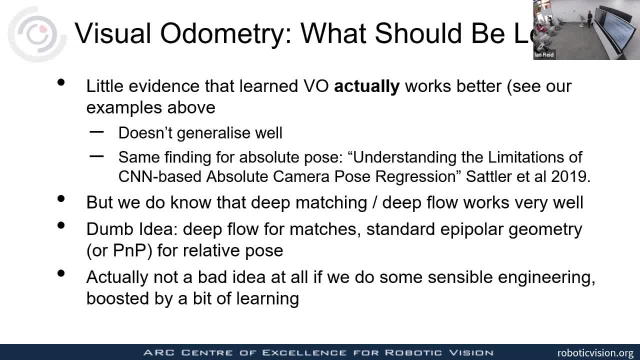 than we have with just using standard geometry. But we do know that deep learning works very well for matching problems and for optic flow problems, And so the dumb idea that my student Huangying Zhan engineered into a really beautiful system was that we use the deep flow for matches. 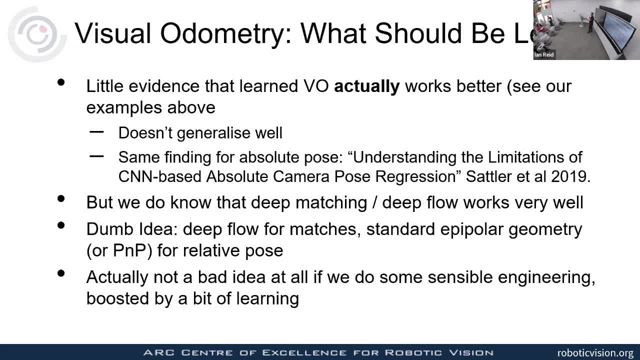 and we use standard epipolar geometry for estimating the relative motion between frames. Or in some cases, if there's no motion then epipolar geometry doesn't work. But if you've got a single view depth estimate, then you can do perspective endpoint. 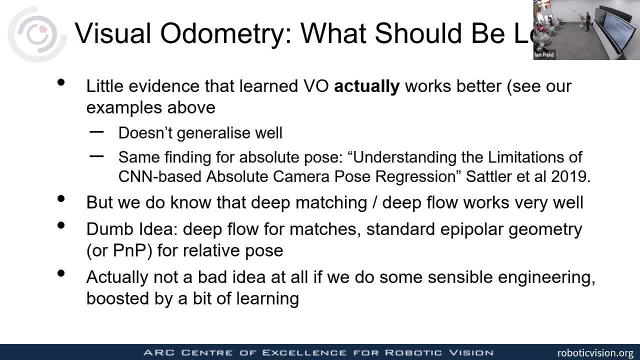 to align your current pose to the depth estimate, And that turns out to work pretty well. And another benefit of having that single view depth estimate is that it sets the scale, which is a real problem for epipolar geometry typically, So it turns out that this is not actually a bad idea. 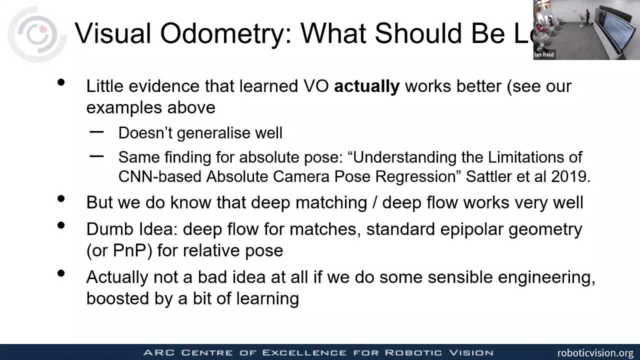 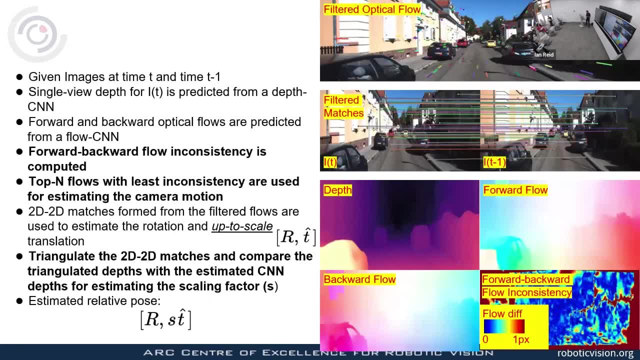 if we do some sensible engineering, that's boosted by a bit of learning, rather than replacing the engineering with learning altogether. So this is a very busy slide, Apologies, but the basic idea is that if we've got images at time t and time t plus one, 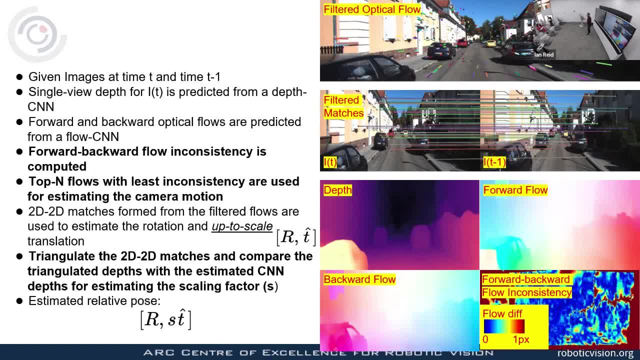 so this is monocular visual odometry, trying to work out the relative motion of a camera as it goes through the environment. we're not so cared about the map, So we have these images at time: t and t minus one. We predict the depth map. 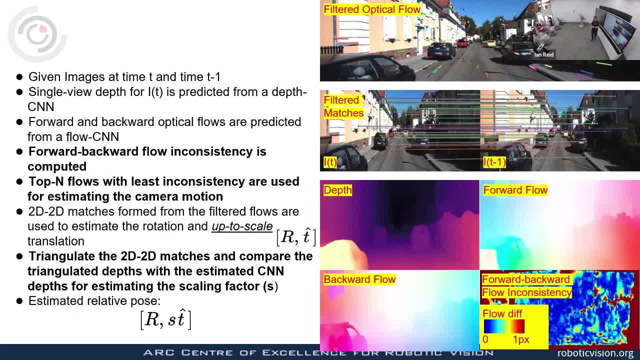 We also predict a forward flow and a backward optic flow And we look where they're consistent. One of the problems with using optic flow or any kind of matching is that you might match into regions that are occluded or unoccluded, And that causes outlays. 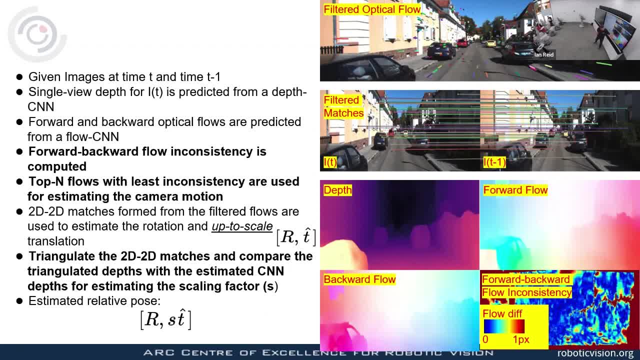 So this very simple check of consistency between forward and backward, you can see that check here: Blue areas: it's consistent, Red areas: it's inconsistent, because there are things that are being exposed in the scene as we move through it that actually don't have a physical match. 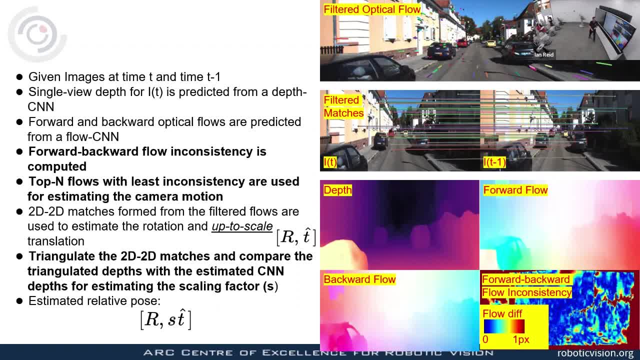 in the corresponding image, And so we shouldn't be trying to match there. So what Huangying did was to look, just to take the top end of these flows. So here are the ones that have been filtered via that top end criterion. Take the very best ones. 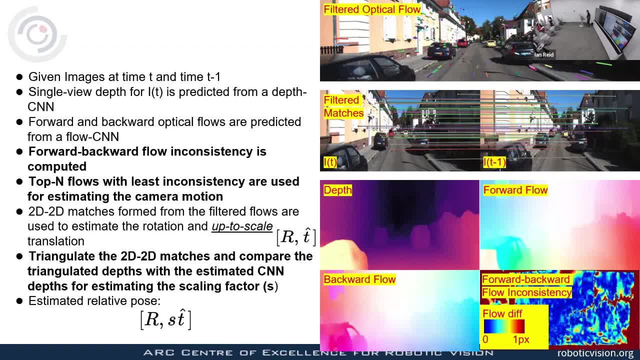 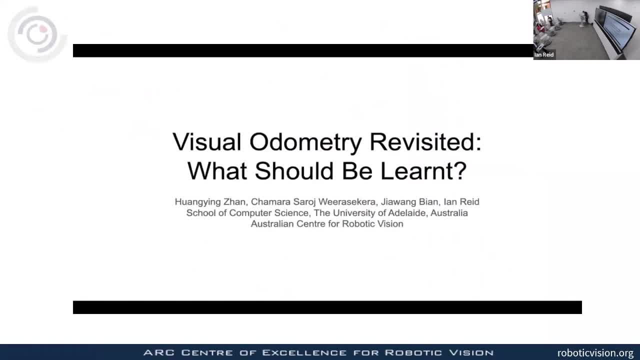 and then just use standard geometry And, having done that, we end up with a system that actually works remarkably well. Again, rather than bore you with the details of bold numbers and the like, let me just show a video that's working. Try to show a video that's working. 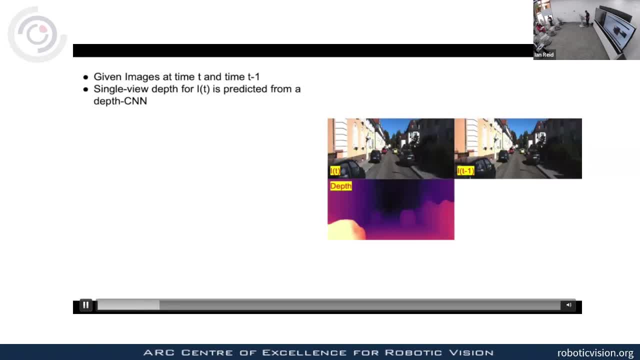 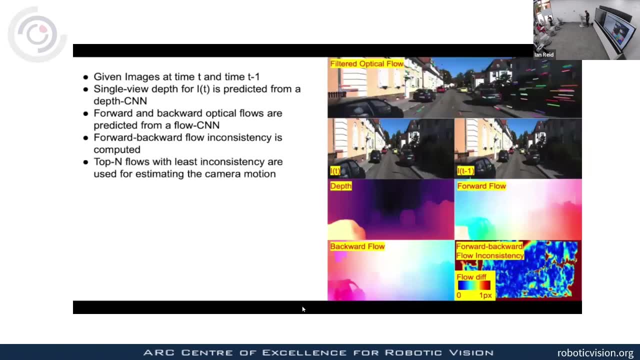 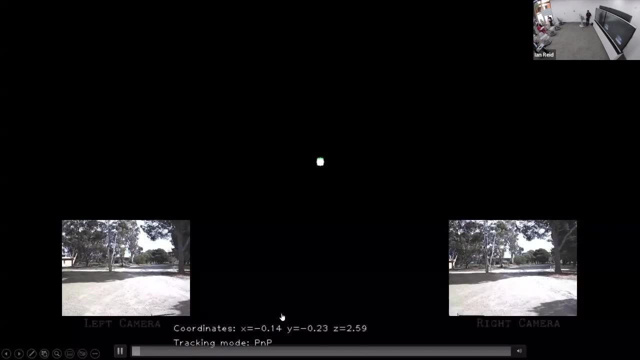 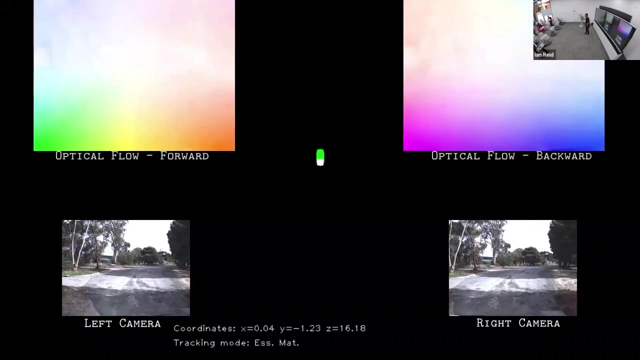 I might even try and skip forward a bit. if you've seen this already, I'll give you a different video, Cut straight to the chase. So this is actually a slightly newer version where we're doing stereo visual odometry. So there are matches, not only temporarily. 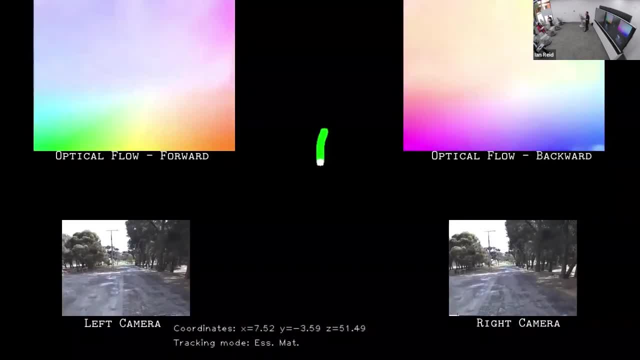 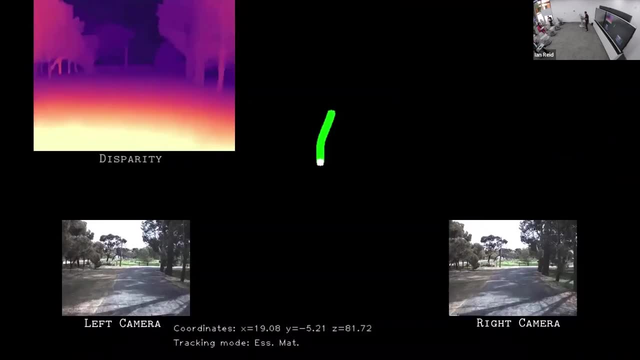 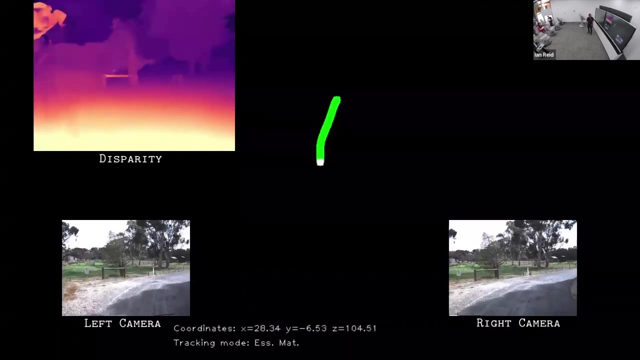 from time t minus one to time t, but also between left and right camera. And the matches now are being done using the raft matching criterion, which is the beautiful algorithm out of Princeton. So what you see here, this is the disparity that's been estimated. 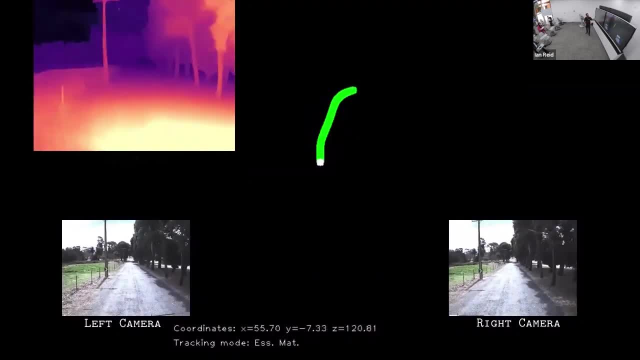 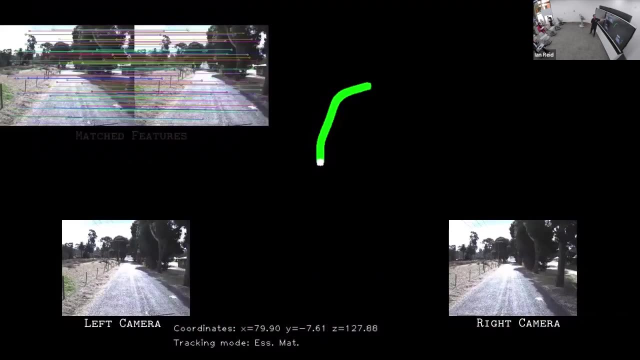 using the raft stereo. We're also doing those temporal matches, as I said, And what you can see here is the trajectory that's been estimated. So these are features that have been matched, from time t minus one to time t that are being used to estimate. 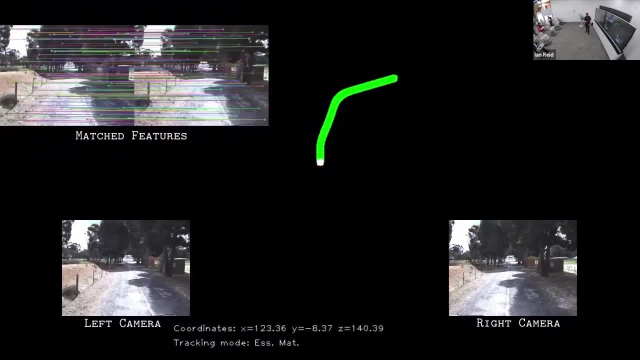 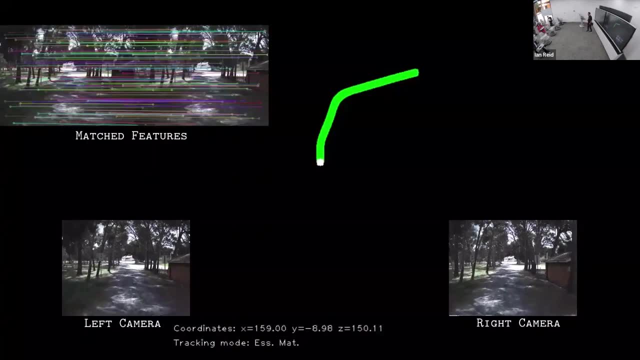 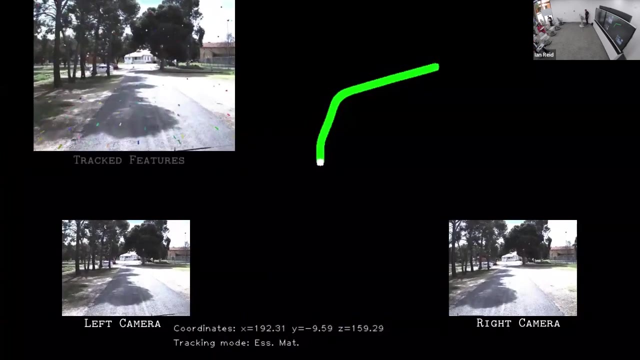 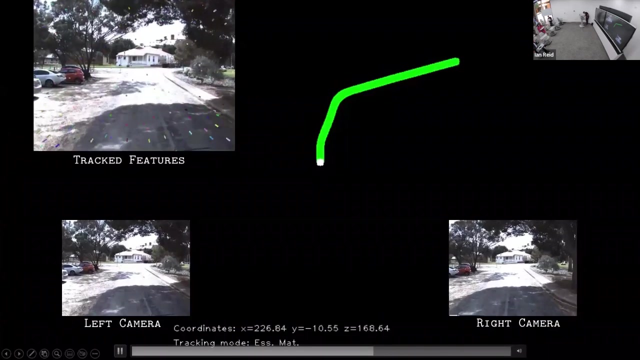 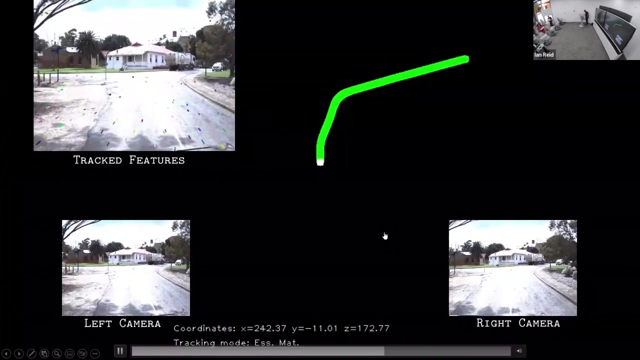 that relative motion of the camera pair And I think at some point, hopefully, this video is going to speed up and you'll see the rest of the trajectory overlaid on a satellite view. So I'll tell you what I'm going to do. 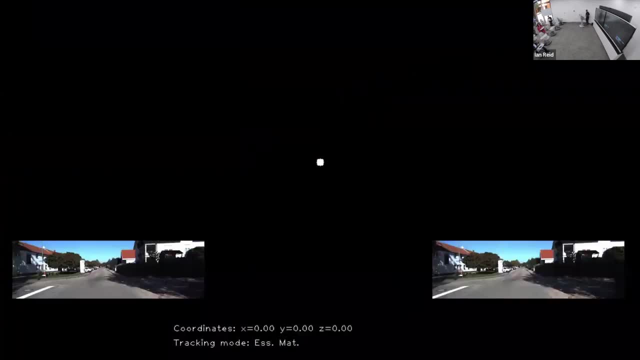 You can all see the video later And then obligatory version running on Kitty, which is the standard data set that everyone, everyone uses. I'd rather show you the one taken from Roseworthy, because it shows it's actually working in the field rather than just offline. 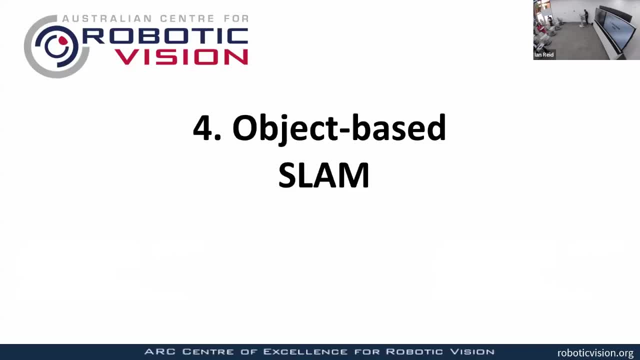 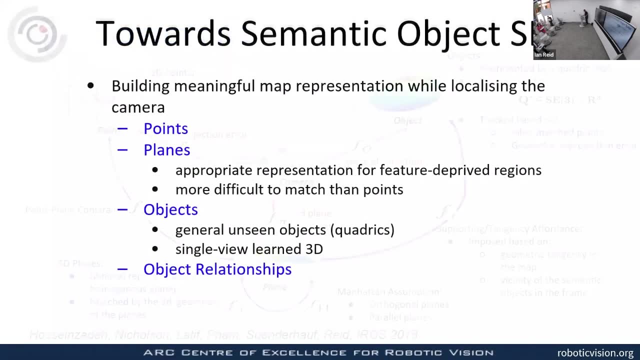 But so I'll skip that other. That says four- I think it's supposed to say three- object-based slam, And I think what I'm going to do in the interest of time is I'm going to skip over these. This is really just the idea that 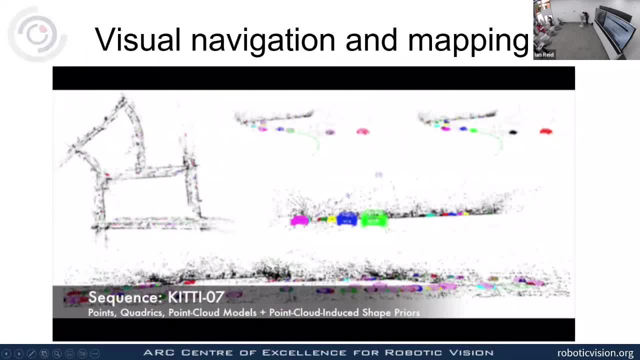 if we can do object detection out of the box, that's the first thing that we're going to do. So if we can do slam out of the box and we can do object detection out of the box, we can also, it turns out. 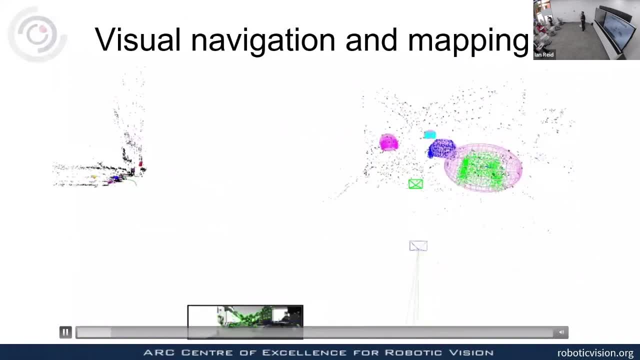 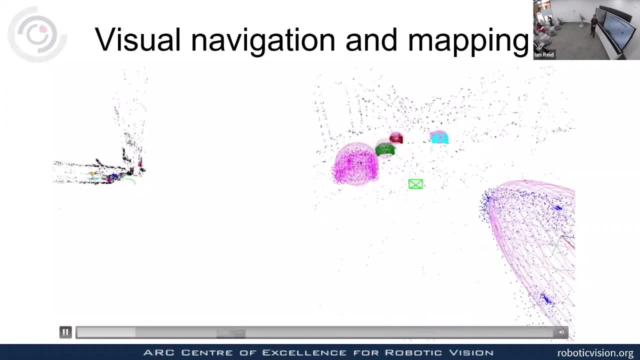 and I'm not going to talk about how we do this. we can do shape reconstruction out of the box. So this is the reconstructed shape of a car that has been detected on the side of the road. We can insert those models into our geometric 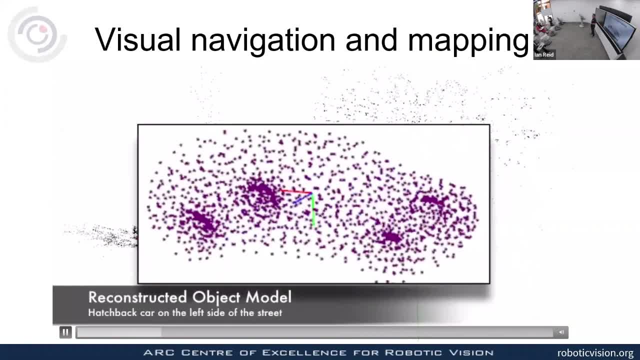 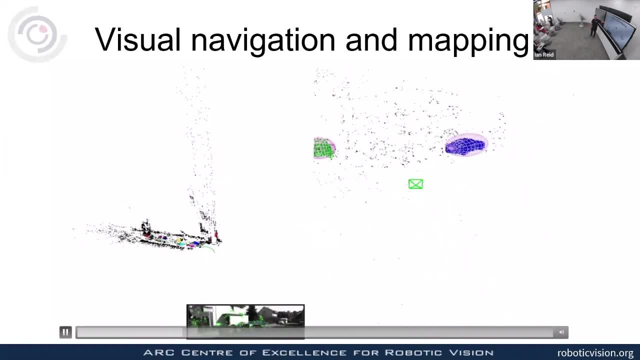 geometric map of the environment, And so we're starting to build towards a model that's not just a map of the environment, but a map of the environment, A map that is no longer just a set of points but is actually populated with objects. 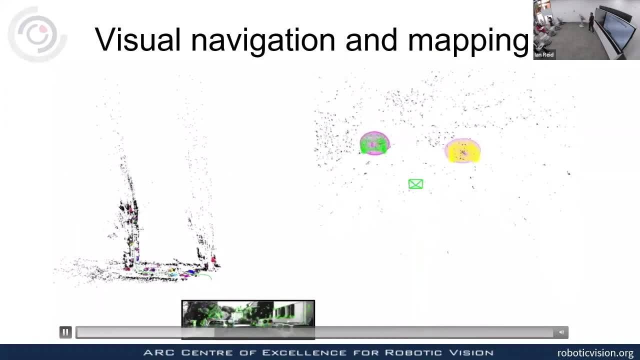 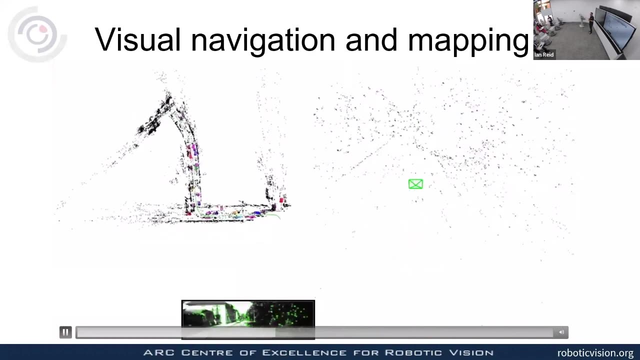 and regions and so forth. So this particular version this video doesn't show detecting planes as well, but the student who created this has the ability to represent generic objects, as ellipsoids, planes, as planes enforce constraints between planes, and objects enforce constraints between planes and planes. 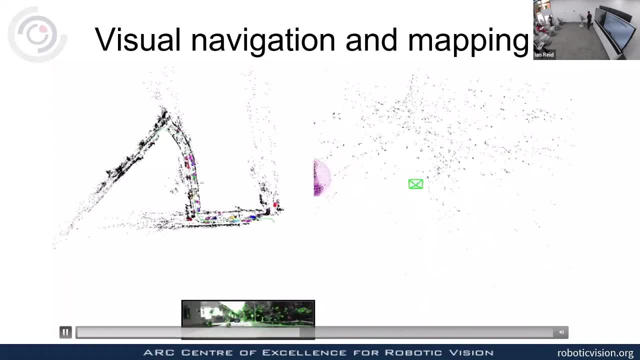 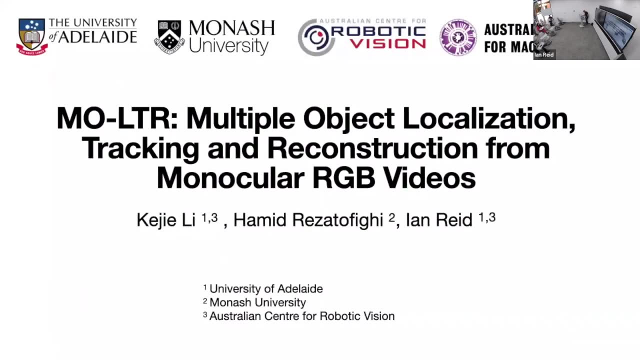 and also use points sericot and so on and so forth in the environment to localize. And I'm going to skip over the next couple of slides as well, because before I finish I do want to talk a little bit about some of the stuff. 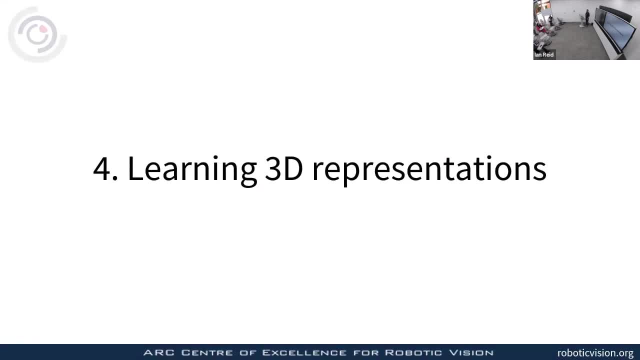 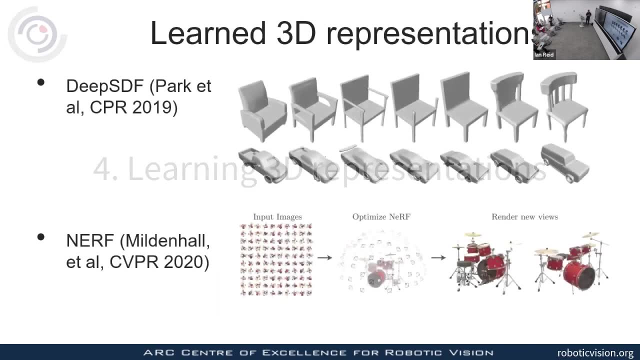 that we've been doing, And this is, in some respects, hot off the press. Some of it's not even published, but I just want to throw it out there as things for people to think about. We're very excited about this idea. well, 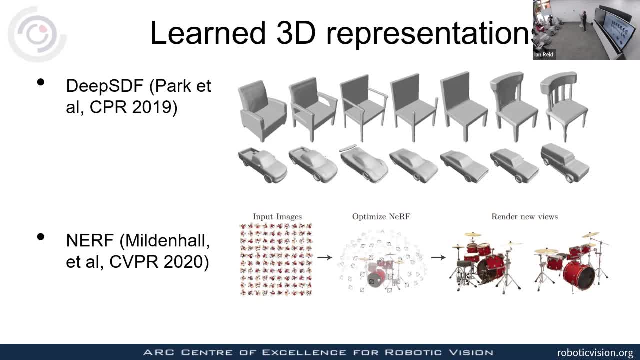 the whole community is very excited about this idea of NeRF. If you work in computer video and you haven't heard of NeRF, then you've probably been living under a rock, despite the fact that it was published only two years ago. But prior to NeRF was something called DeepSDF. 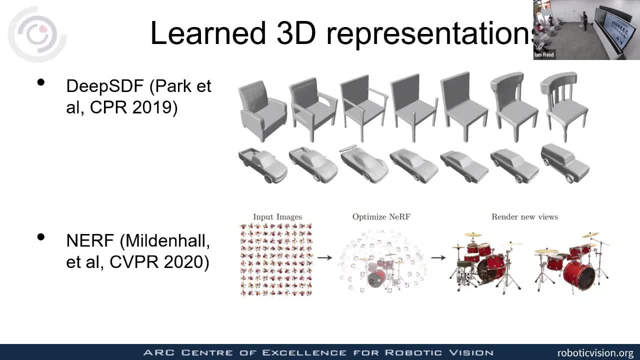 and there are a couple of other papers published around about the same time as DeepSDF. So this came from Richard Newcomb and his group at Facebook Reality Labs. This came from Ben Mildenhall. The basic idea that's at the heart of both of these is pretty. 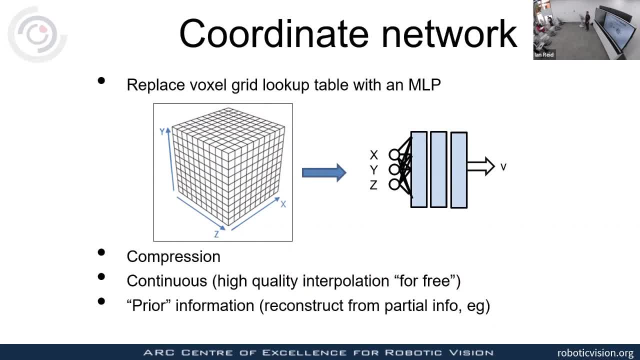 much the same one and it's potentially very, very powerful, and that's why people are excited about it. It's the idea that you can take a voxel grid representation. So a standard representation of 3D space is that you have a voxel. 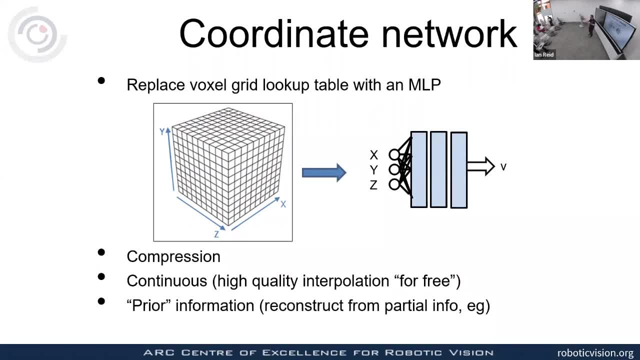 grid and you just say: is this point occupied or is it not? That's your representation of space. You can extend that, still on the voxel grid, to something like a signed distance representation, where the value at any voxel comprises the distance to the nearest surface and that TSDF. 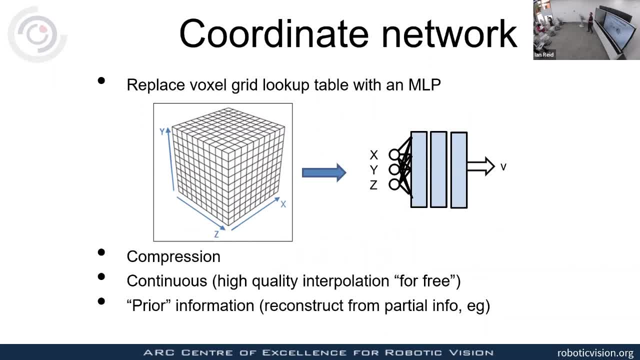 the truncated signed distance function. representation turns out to be incredibly powerful and is at the back end of connect, fusion and various other cool algorithms for reconstructing using RGBD data. But the idea behind DeepSDF and behind NeRF and all these other things is that you 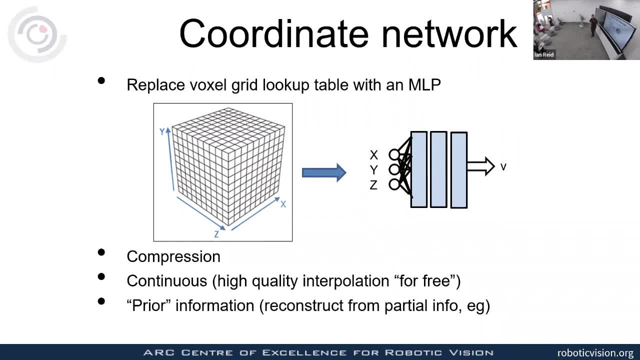 can replace this voxel grid with- which is essentially just a lookup table of your chosen representation- with a multi-layer perceptron. So that's what this is: You pass in a coordinate- x, y, z. So over here, you pass in an x- y z coordinate. 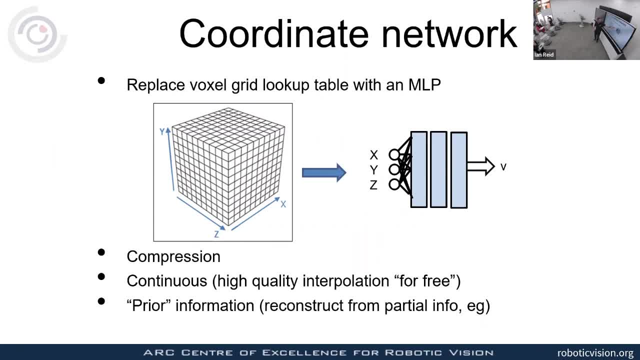 and you get a value because you've got this massive lookup table Here. you pass in your x, y, z to an MLP, You learn that MLP and it produces a value. v that says what is in the case of DeepSDF. 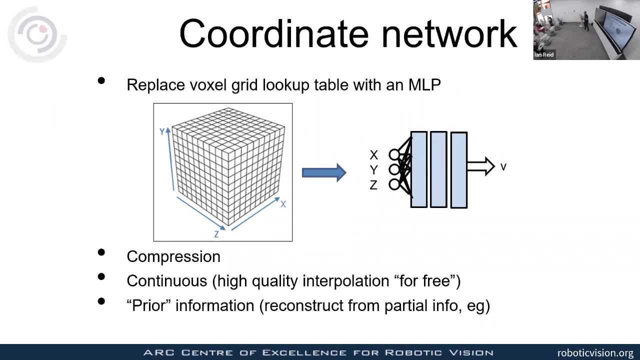 it tells you what is the distance to the nearest surface. It could just be a binary value, It could be occupied or not occupied, Or- and this was the beautiful insight in NeRF- it could be something much richer. It could be things like the density of the surface. 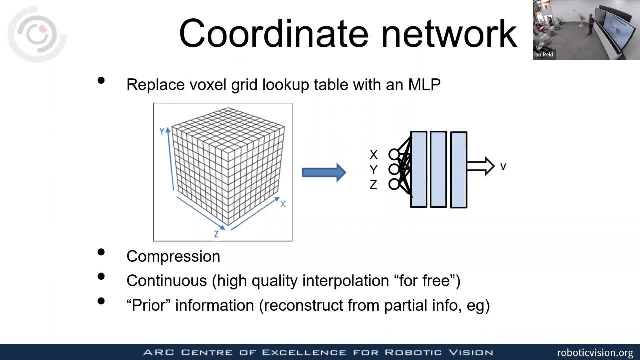 and the color value or the radiance and so forth, So you can then start to use it for novel view synthesis, which is what NeRF was doing. But it's a nice representation for a whole bunch of reasons. One is you can get some potentially 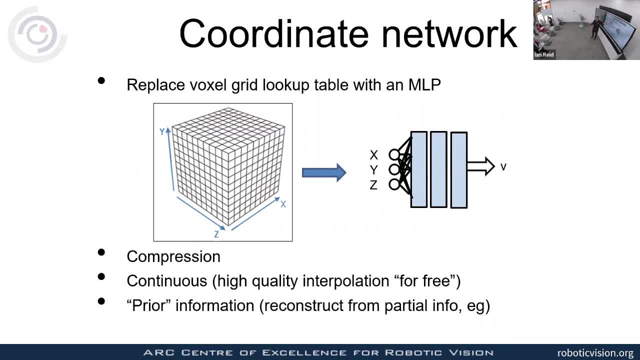 massive compression. There's a lot of redundant information in the voxel grid that if you choose the size of your representation judiciously then you can get quite a lot of compression, sometimes at the cost of speed that goes. It's a continuous representation. 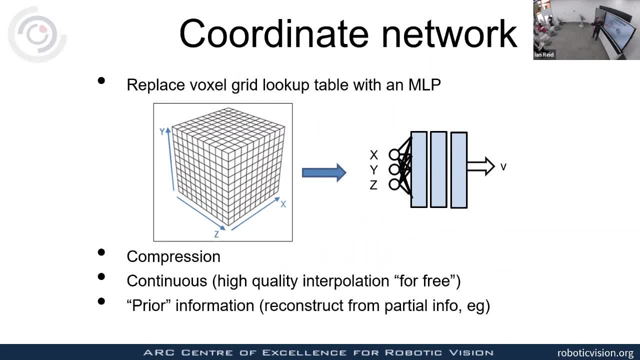 So no longer do you explicitly have to do interpolation depending on the size of your grid, but you actually get high quality interpolation pretty much for free. It fills in the gaps for you. These values that you're passing in here don't have to be values that you trained on. 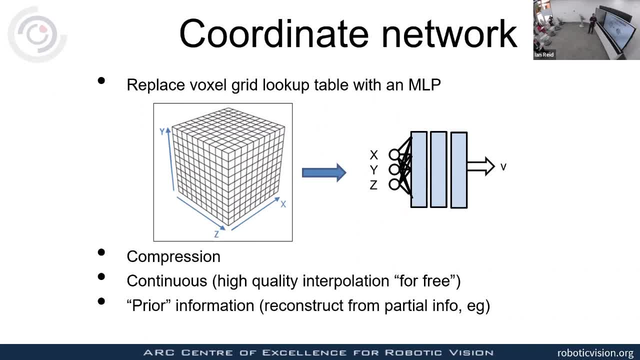 on. they can be values that are intermediate between things that have been trained on, and i think the thing that's most exciting for me- and i don't really know how to do this, people are starting to get to this, but i think it's a very exciting area- is that it can capture. 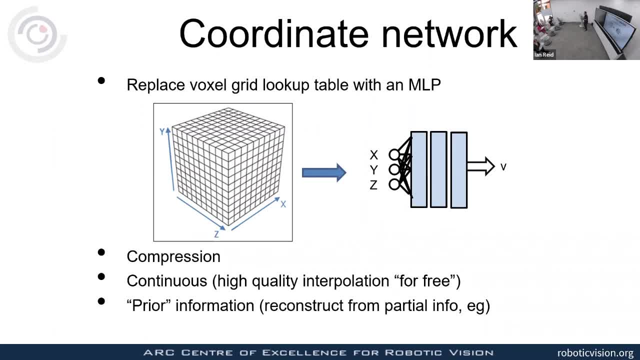 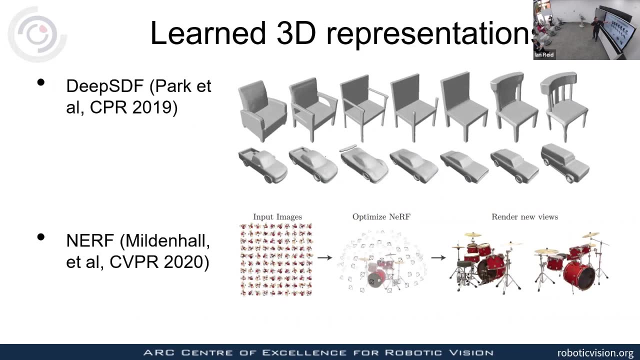 prior information. this is something that has sort of got lost in the rush to replicate nerf itself. if you go back to the deep sdf paper, what they were doing was saying: well, i can actually condition my lookup on some information that i've already got, and so if i see half of this chair, i can. 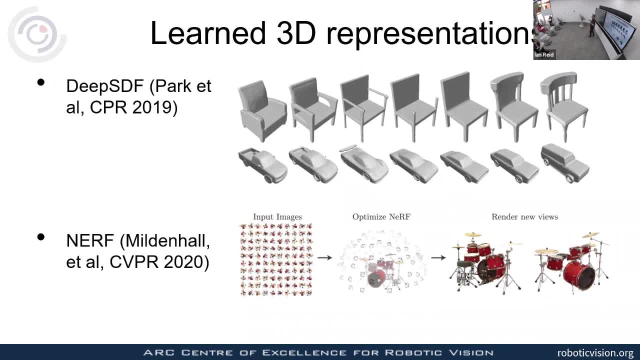 reconstruct the other half of that chair. so it was a class-based learning that they had in the weights of the network, not an instance specific learning, and most of nerf work is instant specific. the great thing about deep sdf was it was class specific um how, how you can leverage that. i think 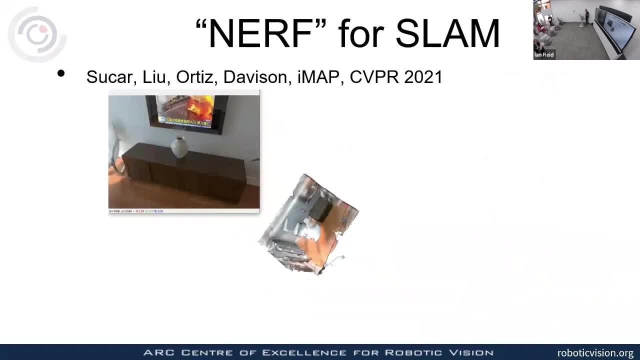 is an open question, but but we're starting to think about some of those things. one of the things that people around the world have thought about is: can you use nerf, uh style or deep sdf representations in a science system, and so the first people to do this were um andy. 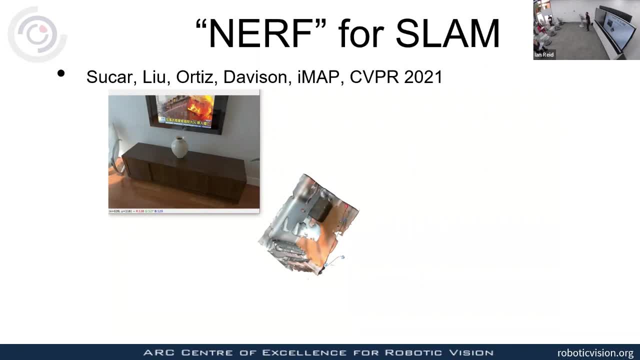 davidson's group. they created a system called imap, um, which was great. i don't want to take away from from that. they were the first to do it. there were some limitations to that system. uh, there was some real cleverness to the system, but one of the problems with it was that it only worked with 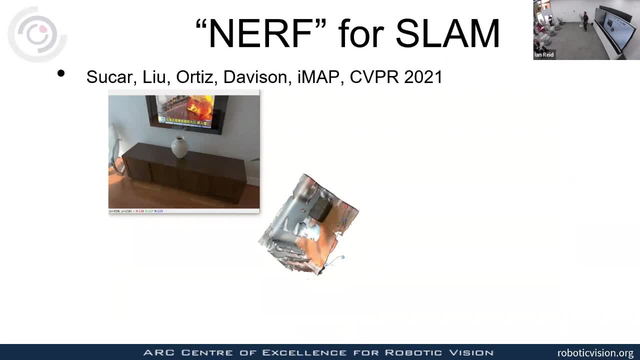 the depth camera, and, and in fact, the depth camera was the only one that worked. with the depth camera, they were using the depth in slightly cheaty kind of ways, but also not using the depth in ways that would have improved performance quite considerably. so, um, and in particular, they were trying to 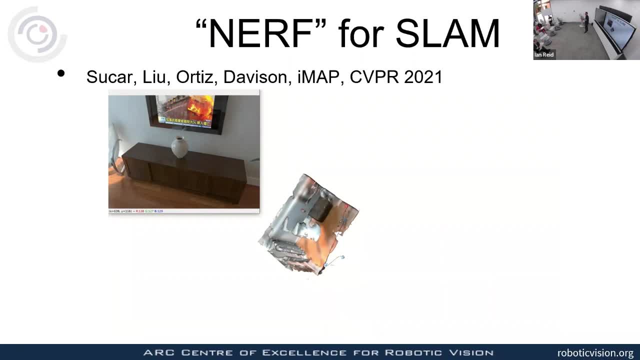 localize the camera with respect to the nerf representation that they had built. so you're trying to build this nerf representation incrementally and they were trying to localize the camera with respect to that, despite the fact that actually what they've got for free from the connect is not only two images but two depth, two dense depth maps. 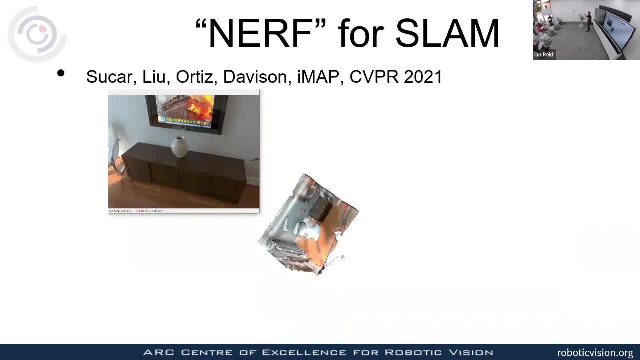 but you could. you could just use iterated closest point or standard epipole geometry to work out how the camera has moved. um, and actually that turns out to be a whole lot better. so, so this is one of the things that, uh, one of my, um, one of my current students did as the first. 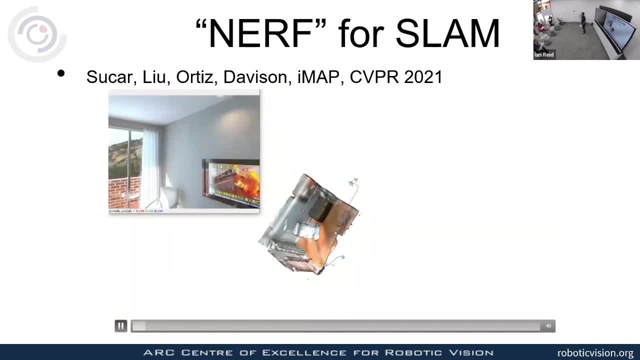 thing in his phd was to say: okay, well, let's create an implementation of imap, but we're not going to localize the camera with respect to the map, we're just going to work out what its relative motion is using standard epipole geometry and standard iterated closest point. it turns out that that works faster and better than that imap. 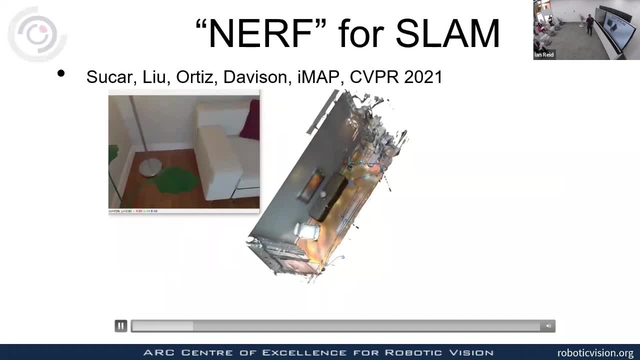 so so we're not trying to use deep learning for stuff that it's not actually very good for, but we are still using that, um, that mlp representation of the environment, which turns out to be great, and you can see that these flat surfaces here really do come out as flat. 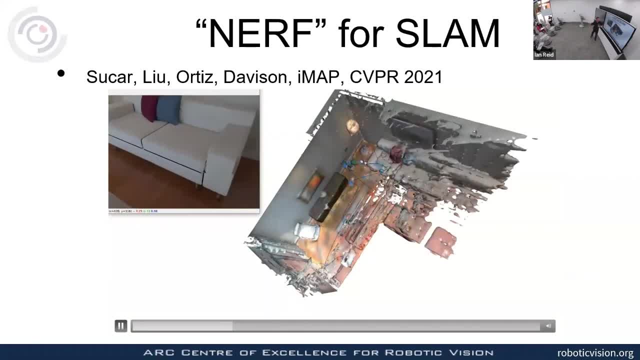 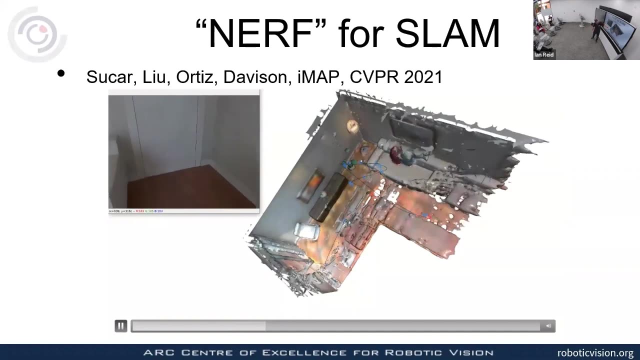 and that's um, that we pretty much get that for free from the, uh, from the earth representation. and i think this video goes on a bit so i won't subject you to to the full amount, but you can see that this, this, this particular system that greg made, um probably. 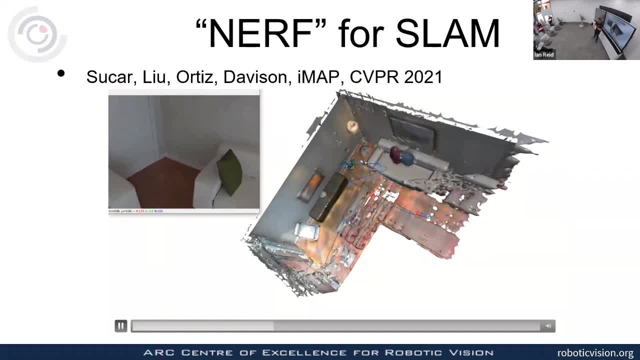 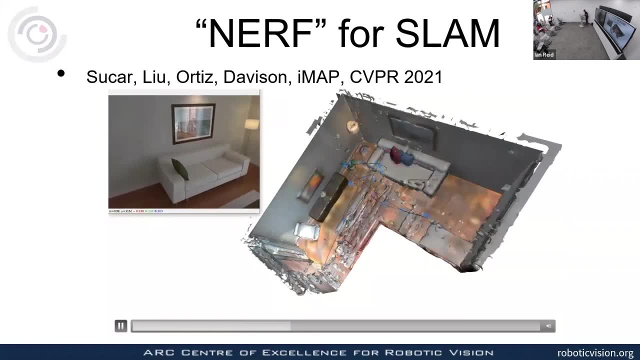 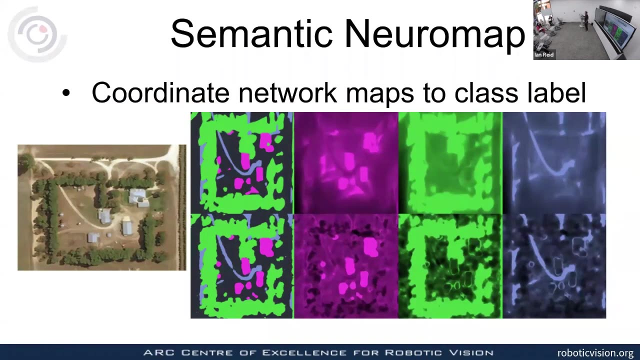 can't see it, but there are cameras being localized, keyframes being dropped along the way, and it's doing a really good job of reconstructing that scene in a dense manner with quite high fidelity. the other thing that we played around with is the idea that you can use 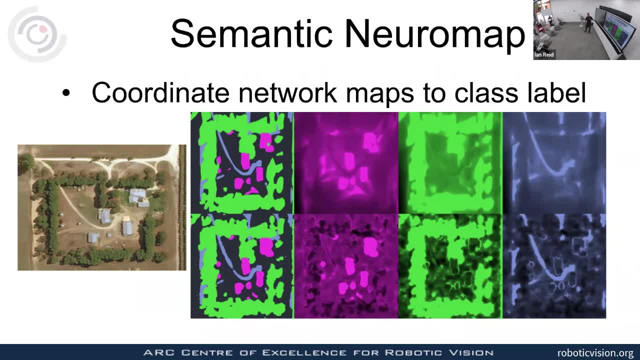 neural representation for a semantic map, so we can take a satellite view of something and we can convert it to class labels. so in this case it's being converted to building vegetation, road and and other stuff. but but what you're seeing here is not a um, just a grid of pixel. 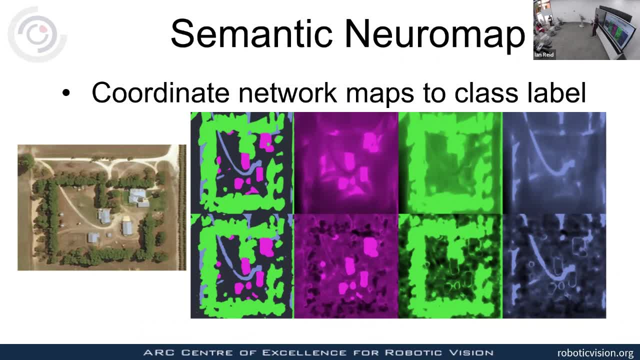 values. what you're seeing here is a reconstruction from- uh, an mlp. so this is a neural representation of the classes. so we can query any point in this mlp and say: what class does this have? um, and that's being reconstructed. so, in fact, what we reconstruct is a series of one-hop vectors, and you can see. 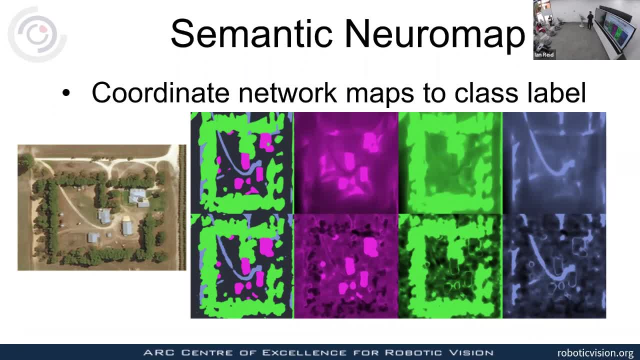 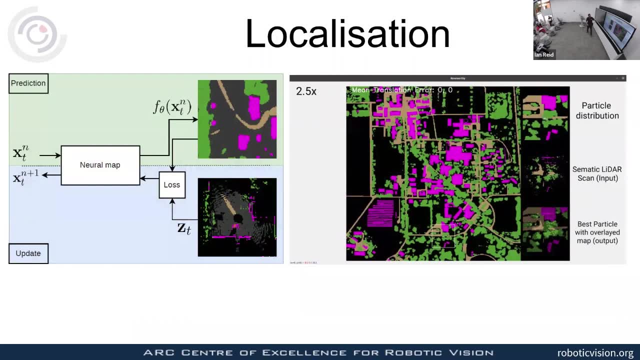 those here, um, and i won't go into the detail of that, but what we've used that for is for doing localization of a robot. so up here we have a um. the neural map is our representation and we can predict what we believe the scene should look like at what we believe the current. 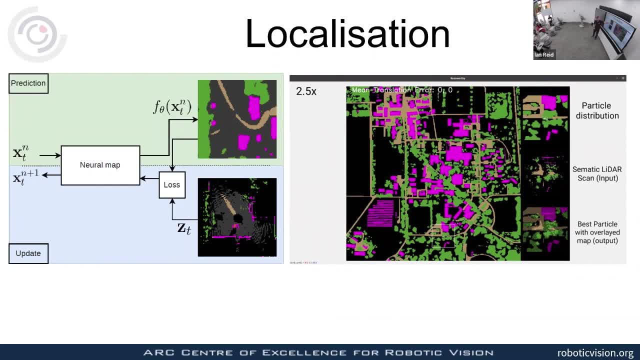 location should be, that goes through the network and so that generates what we predict the scene should look like down. here we have a real observation. this observation has been taken with a lidar that has then been segmented into those, those classes, so this was acquired by a. 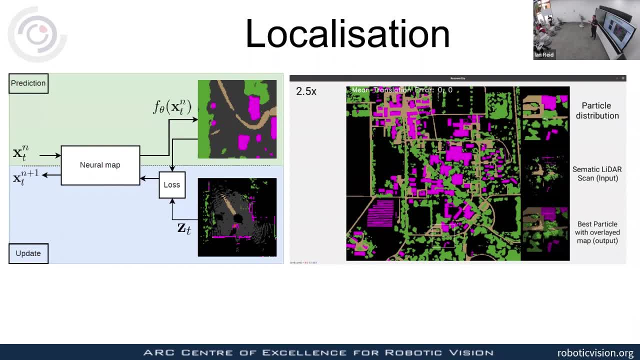 satellite. this is acquired by ground level lidar, telling us what's in our immediate surrounds. and that's what we're going to do. is we're going to go back, propagate that as if it were a loss in a in a network? we're not going to change the weights of the network, but we are going to back. 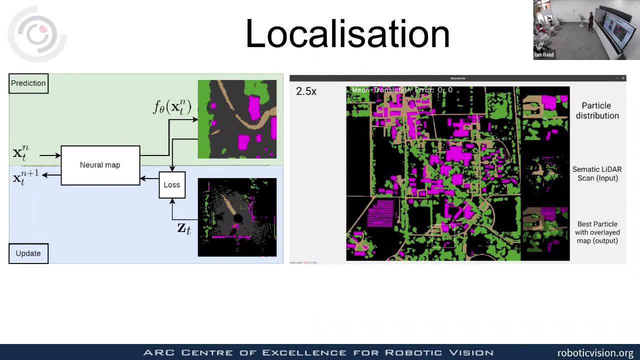 propagate that to find out where our next location should be, basically using the network to do gradient descent to find where this is at relative to to the the overall map. so if i start that video you'll see that running. in fact i think is it running already. 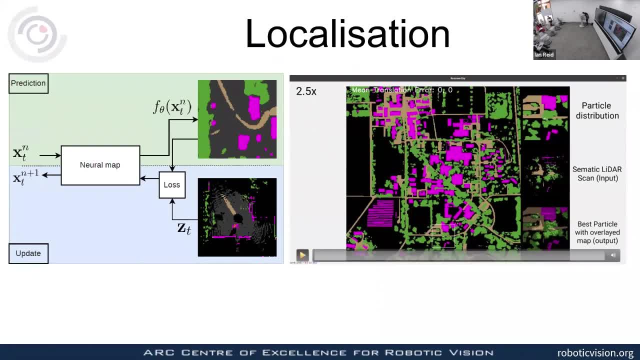 it's running now, so you'll be pleased to know i'm nearly done. okay, so this is the overall map of the scene. there's a distribution of particles here. we're using a particle filter to represent where we might be, so this is a distribution over where we think we are and this is the output of the lidar. so we have a semantic segmentation. 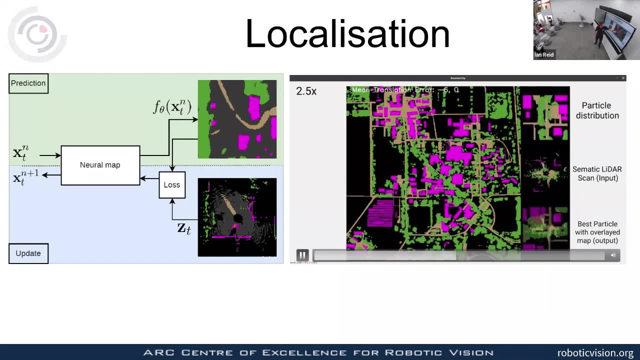 of the lidar. we're trying to find the location in the map here. that is the first point of the map best fit for that lidar, and so you can see the box here. that's it moving along, localizing the lidar to the overhead view of the scene, and what we've been able to show is that that converges with a. 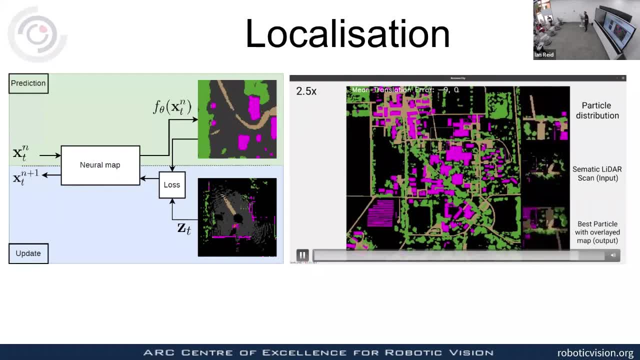 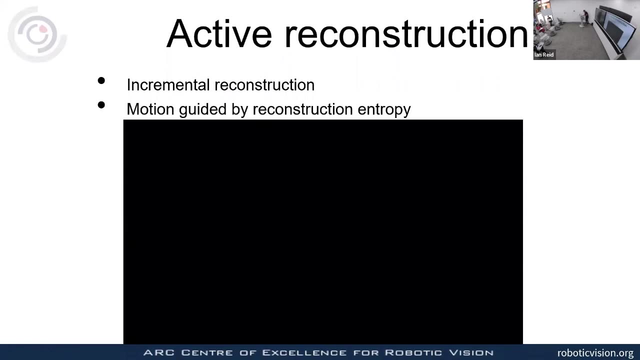 much wider basement of convergence and much faster if we're using the semantic neural map than if we're just using a standard pixelized grid as doing a brute force or gradient based search. and i'm going to skip over the last bit because it's not well actually. no, i'm going to, i'm going. 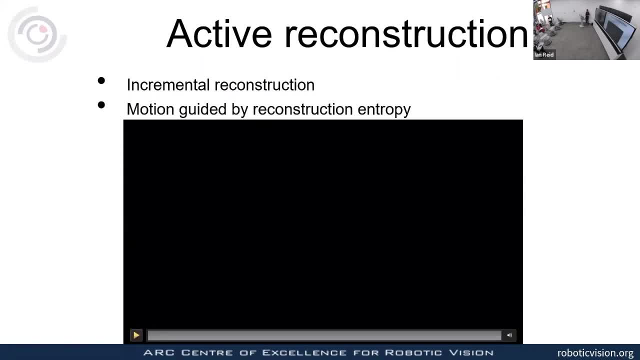 to show you this video. so we've also thought about how can we do active reconstruction. a lot of the the nerf work is based on the idea that you start with a large number of views. but what happens if you have- uh, if you start with only one view and you're trying to build up that can you use? 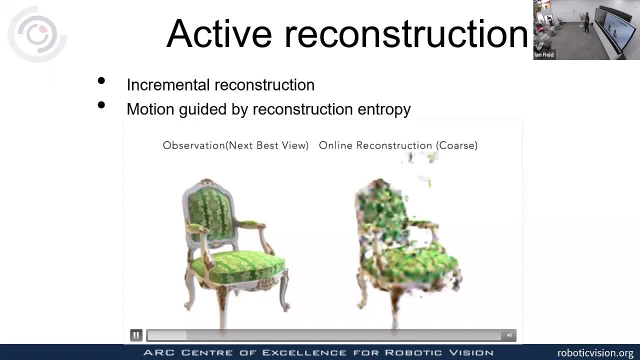 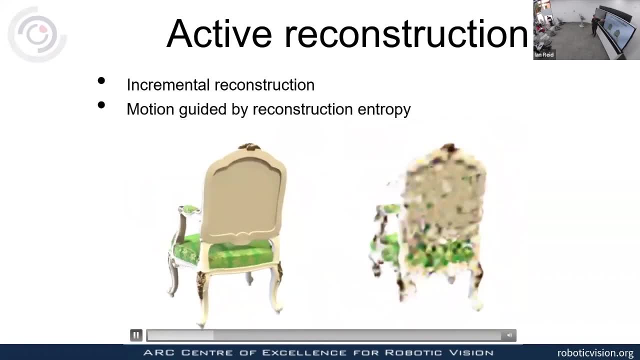 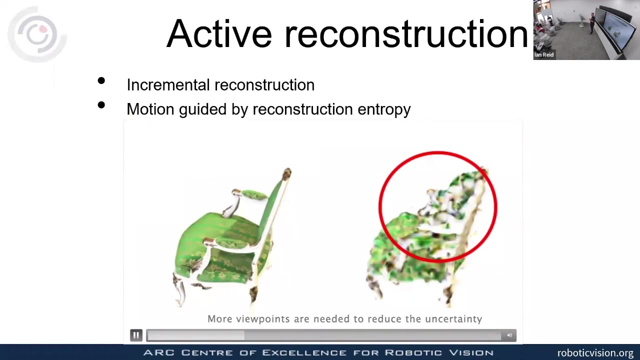 the fact that, uh, you, you've got some uncertainty about what the shape looks like to guide where you should move next. so that's exactly what we've done here. we're doing incremental reconstruction, and the motion of the camera is now guided by the entropy that we see in the physical reconstruction. one of the things that about. 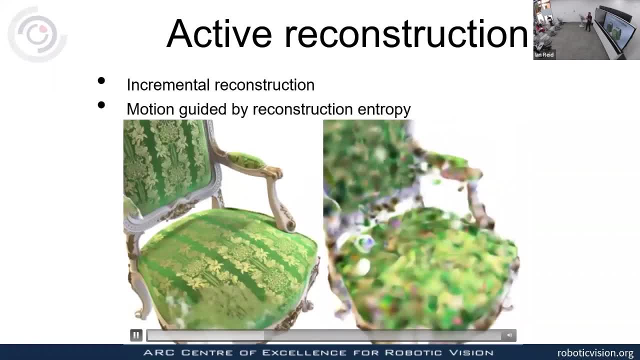 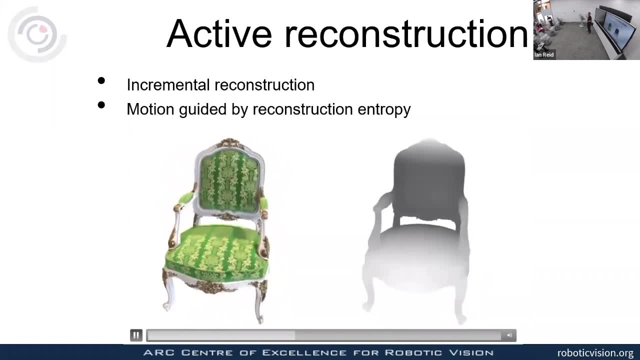 nerf is that it's mostly interested in the quality of re-rendering of an image. as a someone who dabbles in robotics, i'm more interested in the quality of the reconstruction rather than the quality of the rendered view, and so um. so you can see here some 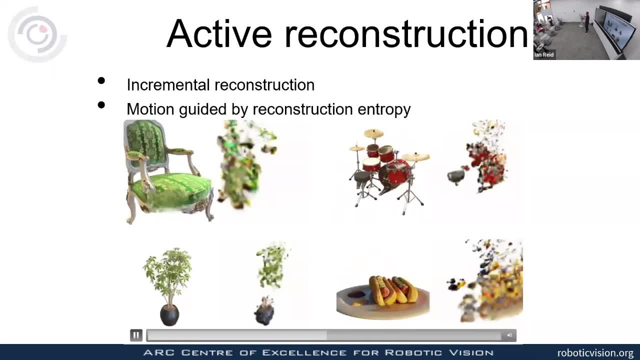 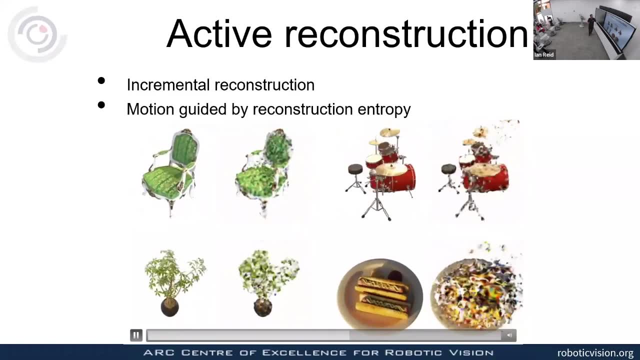 examples of the quality of the rendered view and so um. so you can see here some examples of the is that we've used active reconstruction where physically guiding the camera to move to places that are going to reduce the entropy of the reconstructed scene. um, so that's what's happening. 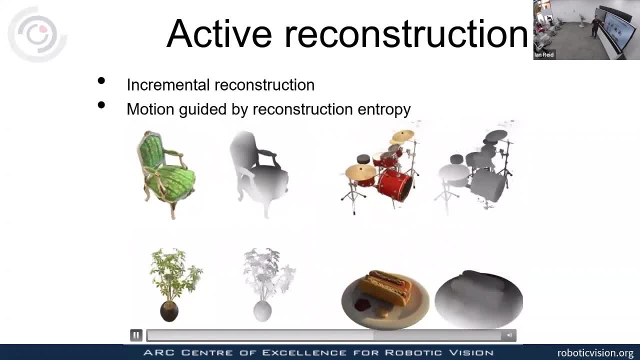 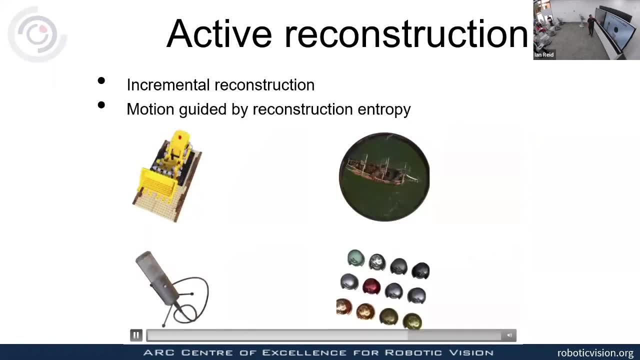 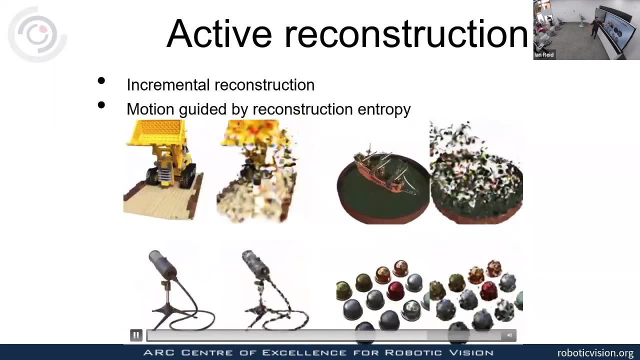 on the uh, uh in those views and then, once we've acquired those views, we can throw them at uh, something that will do a refinement of the shape, and you can see here, from a small number of views, we're getting um, so so this is happening pretty much in real time. we're acquiring this model. 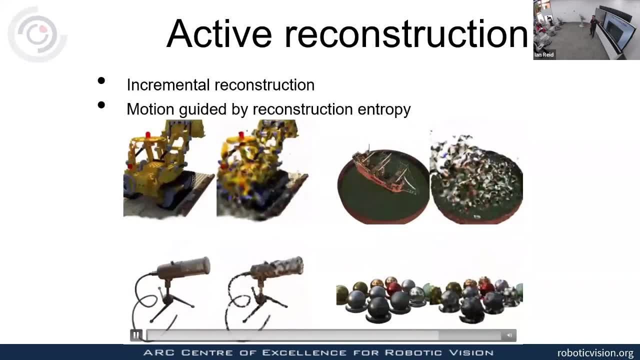 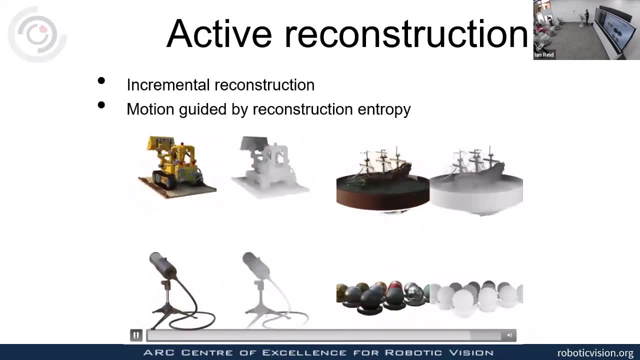 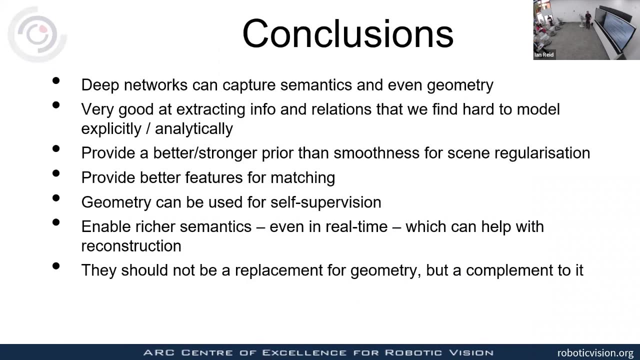 model. it looks nasty, but actually, once it's refined it turns out to be very good. so offline, we can then refine and we end up with something that's really quite high fidelity in terms of its shape. okay, so various conclusions. first of all, as you've seen, deep networks can capture. 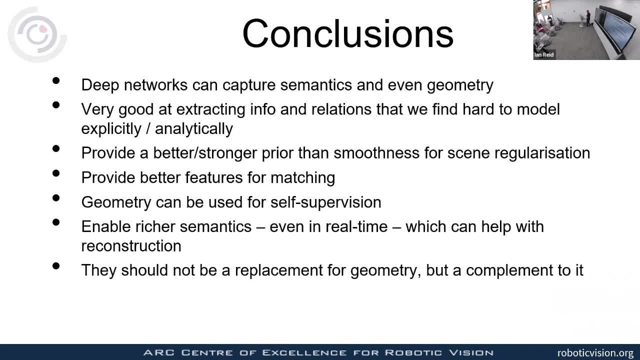 semantics, and they can even capture geometry in in quite interesting and powerful ways. they're very good at extracting information and relationships that we find hard to model explicitly or analytically. but to me that says we should use them in instances where we do find it hard to model these things analytically. if we can model something well analytically, then 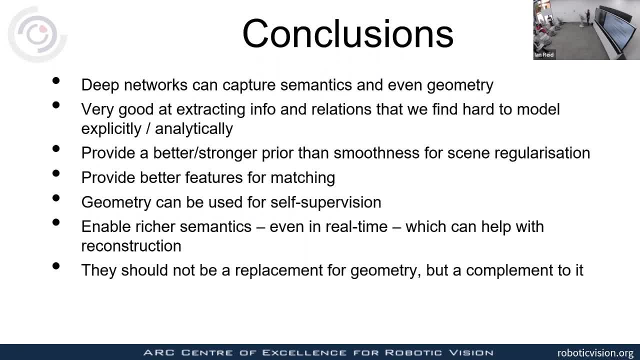 then i think that we should. deep networks obviously do certain things very, very well, so they provide better and stronger priors for smoothness, for scene regularization. they provide better features for matching. i've also shown that we can use geometry for supervision so that we can then boost the performance of other geometric systems at a later date. 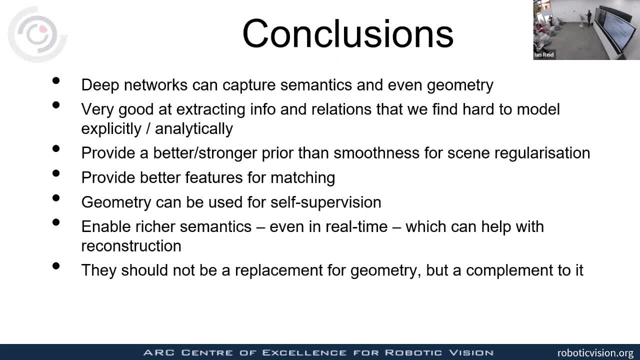 they obviously enable richer semantics and sometimes even in reconstruction, which can help us with, uh, even in real time, which can help us with reconstruction? um, and- and i guess part of the message- and maybe i've banged on about this a little bit too much during the talk, but i think 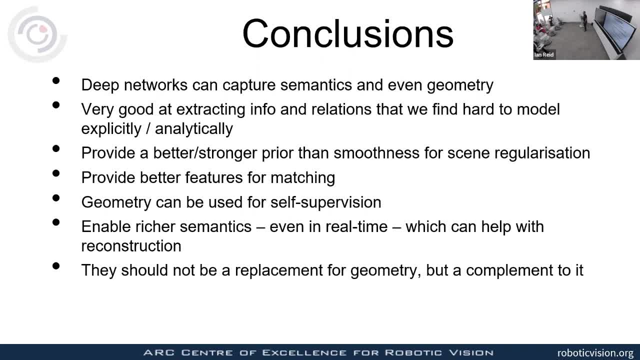 that deep networks should be a supplement for and a complement to geometry, not a replacement for it. i think it's the wrong way to say. we're going to just going to use feed forward and it's going to produce geometry, um, or it's going to produce semantics or anything we should be thinking about. 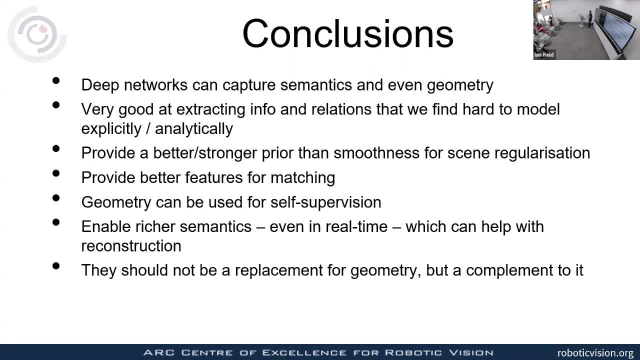 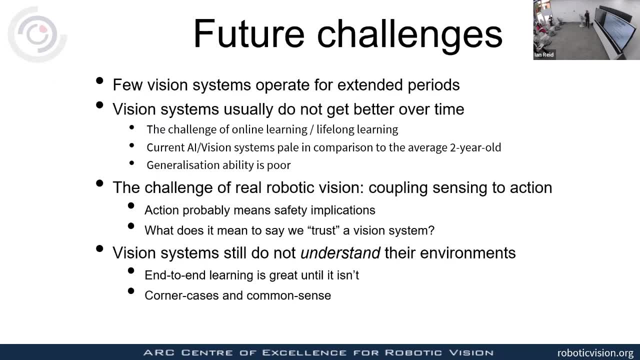 what do we know how to do now and how can we use deep learning to make it work better, rather than replace it with deep learning? so what are the future challenges? well, there's still lots. um, in fact, my talk tomorrow went very well, but I should say sort of before july. was this amount of knowledge that i have as our data that we're going to be taking about how we can actually 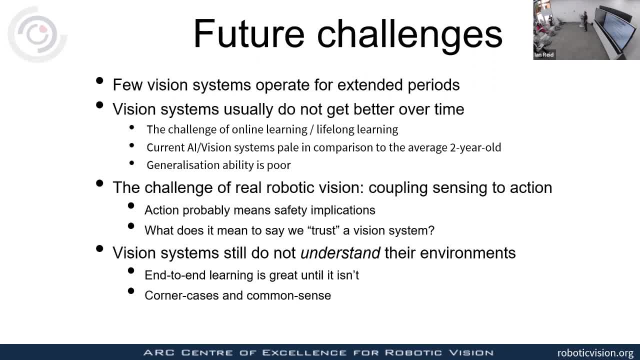 I'm going to show a something that I saw when I first walked into Mike Brady's office. Many of you might know Mike as the, I think, the original president or interim president of MBZ UAI And he was my PhD supervisor. I walked into his office in 1988, I think it was. 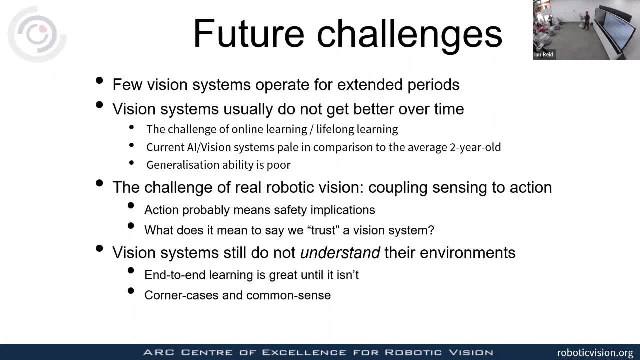 And on his wall was a handwritten note from Olivier Fojerals, who's another one of the founding fathers of computer vision, And it said: in five years time all computer vision problems will be solved and we will be out of a job. If they have not been, then I undertake to buy Mike a six bottles of very good claret, or he will do the same for me. 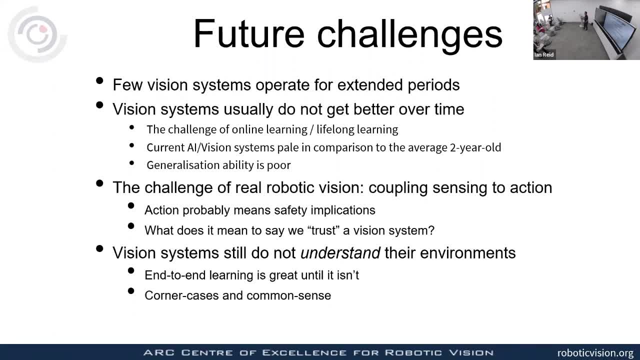 That was written in 1986.. Needless to say, Mike won that bet. I've never asked him what claret Olivier actually bought him, but few vision systems operate for extended periods, So that's something. If they're going to be part of a robotic system, they need to be able to operate reliably over extended periods. 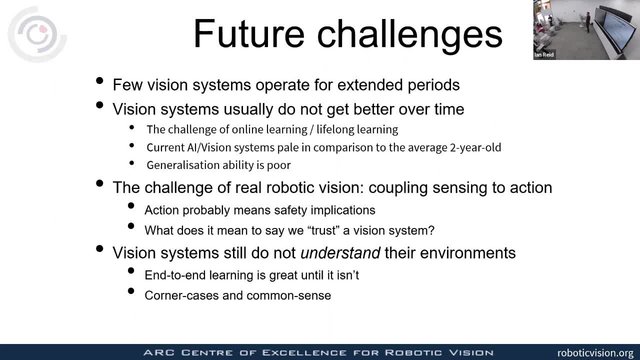 They usually don't get better over time, And some of the self supervised methods that I've been talking about, I hope can be a step along the way to making these things work better over time. So we still have this challenge of online learning and lifelong learning. 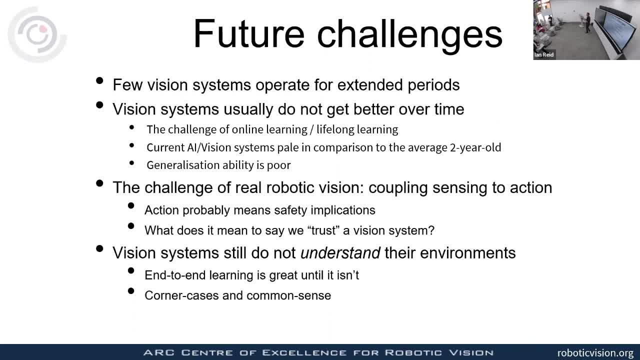 In particular, even current systems that are so impressive compared to 30 years ago when I started, they pale in comparison to the average two year old And they don't generalize. We now know that we can throw a huge amount of data at these things and they can do pretty well. 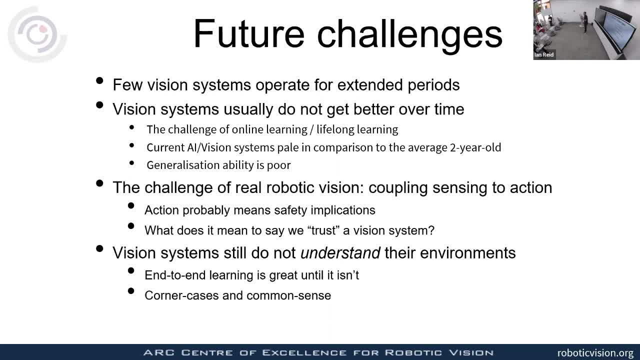 But show them one picture of a horse and one picture of a zebra. They won't be able to distinguish between where an average two year old can probably point to lots of other horses shown a single example. So their generalization ability is poor. 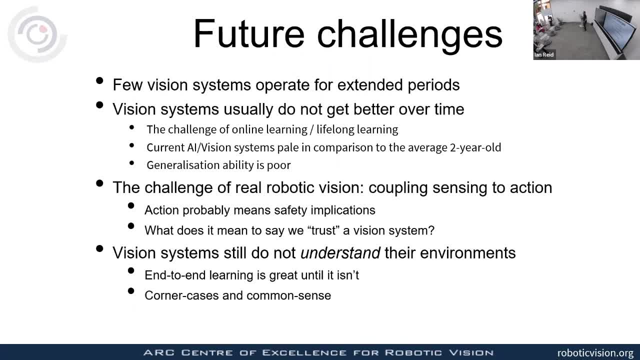 And for me personally, the challenge of real robotic vision is how do we couple sensing to action, And one way of doing that which is just to say: well, let's just suck in pixels and join that to imitation learning or reinforcement learning. 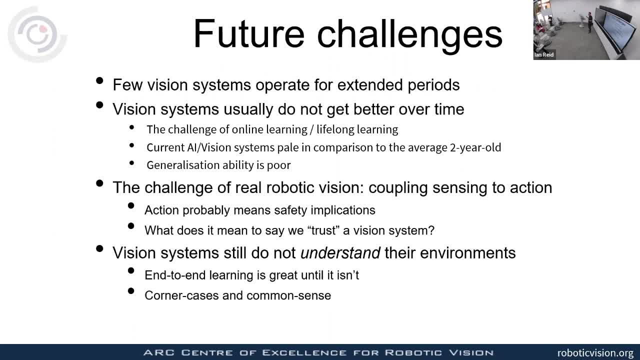 To me that has some pretty serious safety implications. It actually works incredibly well And my postdocs and students are repeatedly showing me to be wrong in terms of how well it can work. But I struggle to see how we can ever trust a system like that, because I don't think we can ever be sure about things like corner cases. 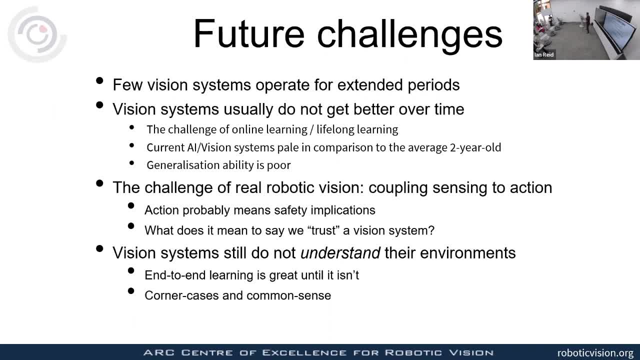 And common sense, And that's because the vision systems still don't really understand their environments and they can't tell us why they went wrong if they went wrong. I don't have answers to those, but I think they're really fascinating questions for us to be thinking about in the future. 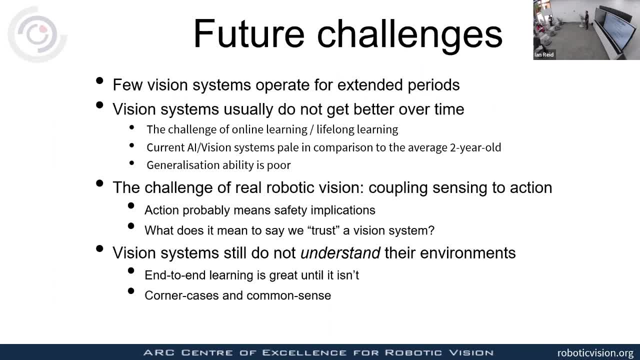 And I'll stop there. Thank you very much. Questions. Thank you very much for an interesting talk. So I have a couple of questions. The first one is that in the start- Yeah, You mentioned substituting the intensity values with the D feature representations. 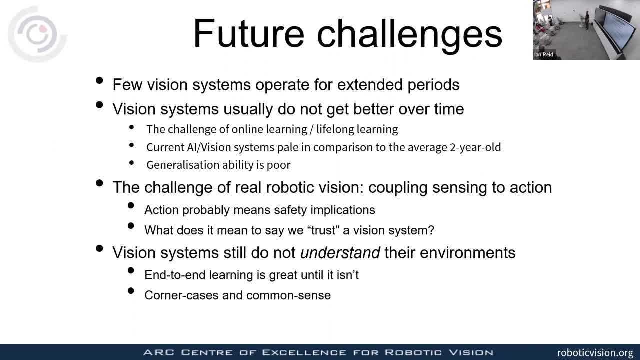 So I wonder what was the dimensionality of the features that were used there? Yes, So in that instance I suspect they were about 32 dimensional, But I think the dimensionality of those features I don't actually know the details of that. 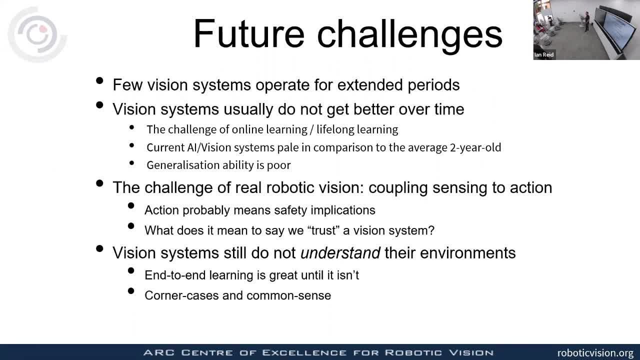 But in that instance the dimensionality is less important than the receptive field of those features. But I think what makes them work so much better is that they've been computed over quite a large receptive field And that means that a point here on the wall looks quite different from a point here on the wall in terms of its feature representation. 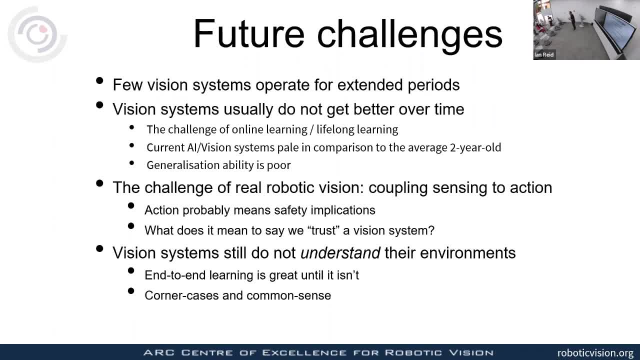 So I don't know, I'd have to talk to Siraj who did the work, But I suspect that a relatively small dimensionality would be enough to capture the differences between that point and that point, Providing the receptive field is wide enough. I mean, the reason I asked this was I was just wondering whether the intuition was to use or get more the semantic representations or use more low level feature representation that replaces handcrafted intensity or RGB based features, just to get a better localization. 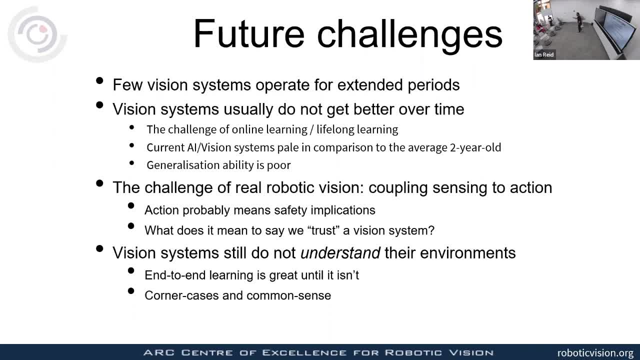 It's the latter Most definitely. You can, of course, use those features to go further, to be able to get semantic representations and so forth, And at the moment a lot of our systems we almost have a separate system for doing this, a separate system for doing that. 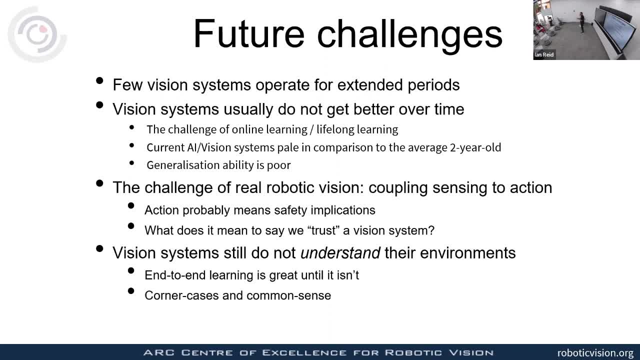 But perhaps we could be just learning generic features that are good for all of those tasks. I don't know that anyone's done that, And we were certainly thinking more about the localization ability. One of the things I didn't talk about in that particular work was that we then we did some self supervision there. 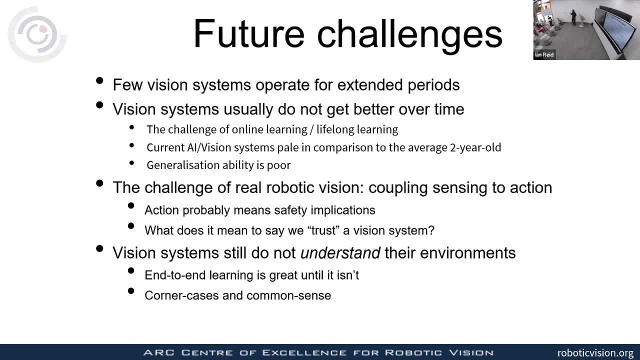 So those features that were being matched, we would look at how well they were matched And if they weren't matched well, we'd use that as a back prop signal to try and improve the features themselves once we'd localized the camera. And my second question is: you also mentioned here in the future challenges about the applicability of these vision systems working for an extended period of time. 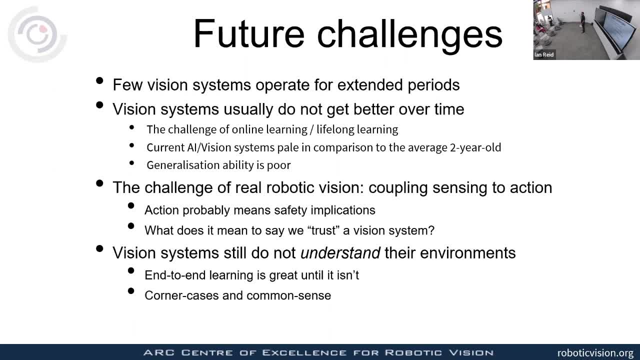 So in that regard, for instance, long term visual localization is kind of a very practical issue. Yes, There are day and night changes. Yes, And there are seasonal variations and weather variations- how we can effectively get six degree of freedom for accurate camera poses. 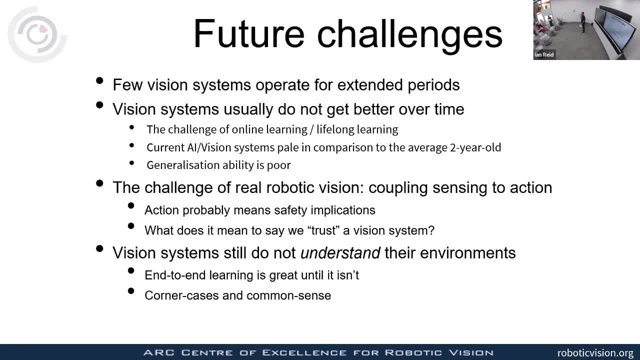 So recently there have been work by the groups of Joseph Sivich and Freddy Carr. They have introduced a data set called visuallocalizationnet And they showed that a lot of these methods- visual localization methods- kind of struggle for this long term localization. 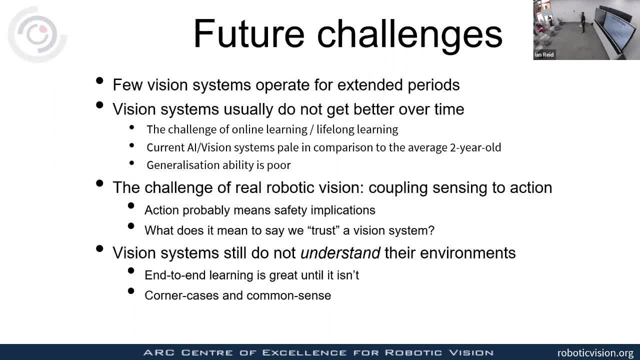 So I just wonder where, what do you think where the community kind of stands at the moment, and what do you think could be done? Yeah, so my colleague, Mike Milford, who was an investigator with me in the Center of Excellence for Robotic Vision, has made his entire career around localization. 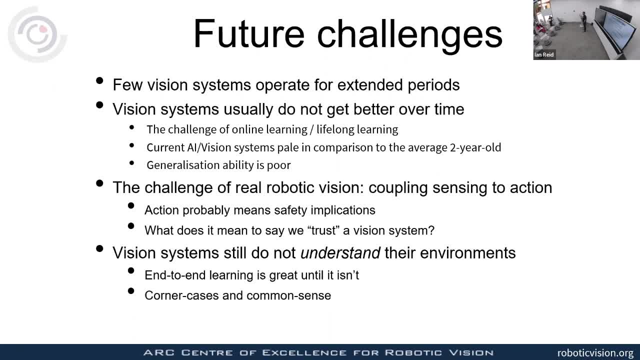 That's pretty much the only problem that he thinks about these days, And he's particularly interested in those changes in weather and scenes and so forth. I don't have a solution, So various things that we have dabbled with have been along the lines of doing domain transfer. 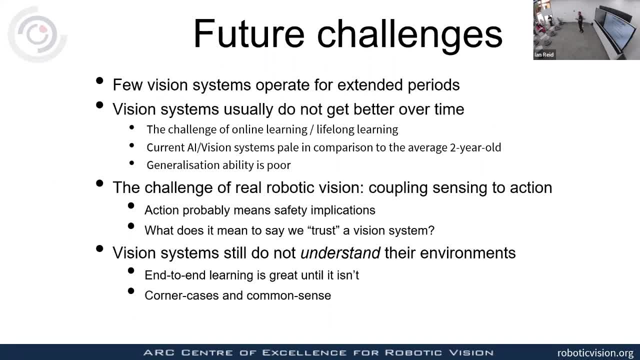 But maybe what you've got is a huge data set that works during the day. How do you and can you make it generalize to the nighttime? And perhaps the way to do that is via domain transfer. That domain transfer might be, for instance, using a GAN or something else. to you condition your GAN on the daytime. 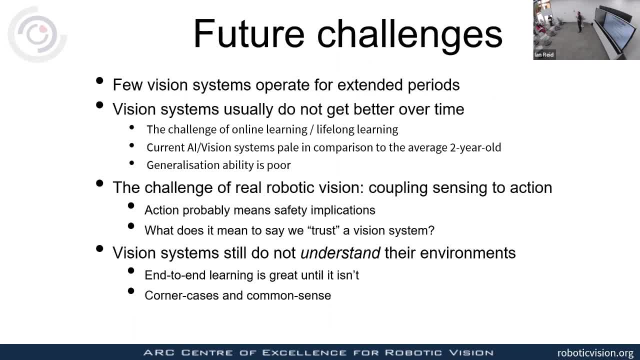 And you try to generate a nighttime version. The same thing And you could do- and we've shown some success doing that- The other approach that actually for some applications works really well. it's practical, but I think it's very nice. 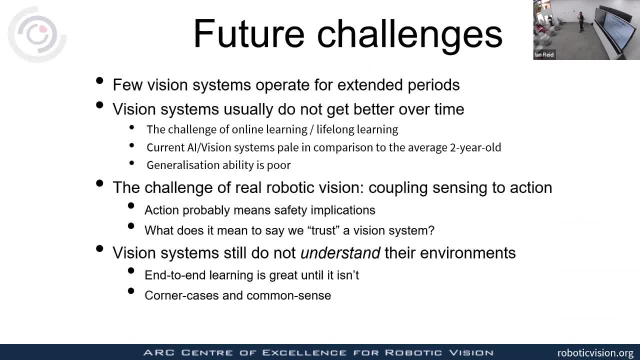 So Paul Newman has this idea of the experience And he uses the fact that if you're driving through an environment, you've got a whole bunch of other cues that tell you that you're driving through the same environment. You don't just have to rely on the visual thing. 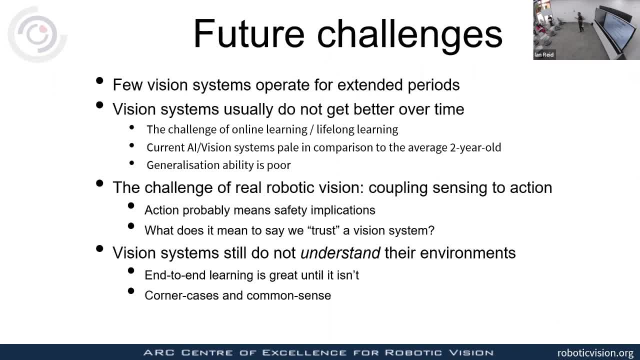 You've got, maybe, odometry, You've got relative motion and all of these things. So he says: I know that I am where I was two weeks ago, But it looks different, Maybe because there's a lot of cars parked there, Or maybe it's snowed. 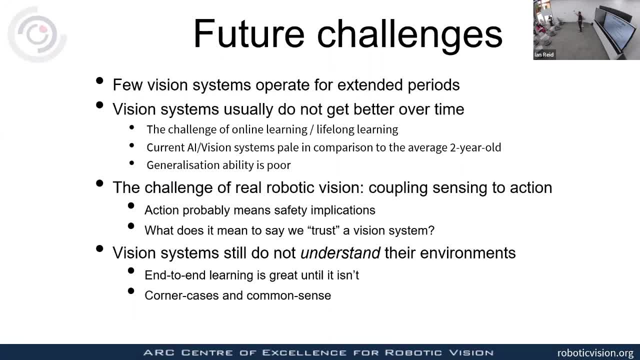 But I know that I'm in the same place, So what I'm going to do, I'm just going to keep what he calls visual experiences. You just create this big database And the more you do it, the more experiences you accumulate. 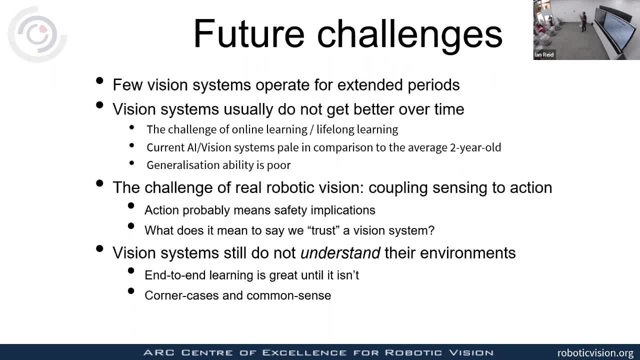 And you get better and better at localizing And I guess that's the equivalent. So I've been around in vision for long enough to know historical solutions to various things as well, And object pose recognition was one that taxed people in the early days of computer vision. 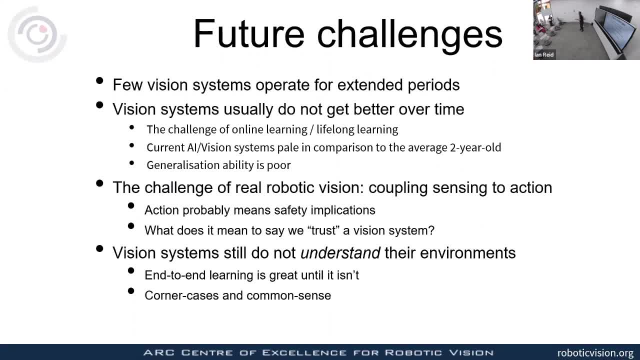 And what we all tried to do was to come up with geometric invariance that if we could find those things in the image, they would automatically give us mathematical information about the pose. And so there's stuff from Joe Mundy, There was stuff from Grimson. 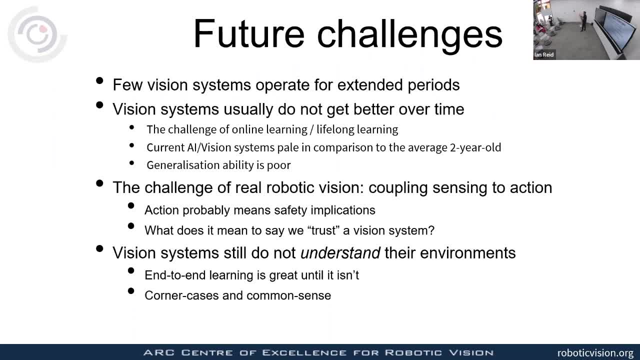 Lozano-Perez And so forth, Where if you found these geometric things- the surface normals or the angle- then you could get access to the pose. And I think we were worried about that because we didn't have much compute power, We didn't have much memory. 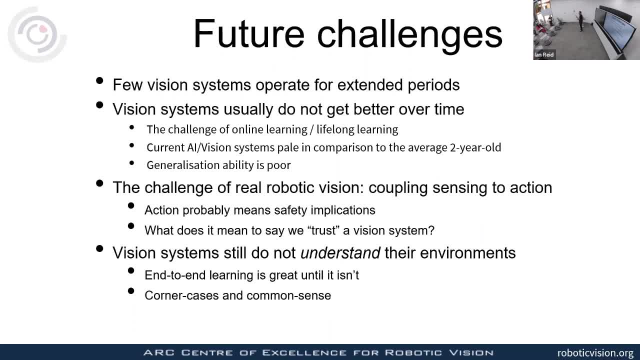 But what's turned out to be a much more effective way of getting recognizing pose, for instance, is just to look at many, many views of the object, And the Newman solution to that, The Newman solution to the changing appearance of things, is very much in that. 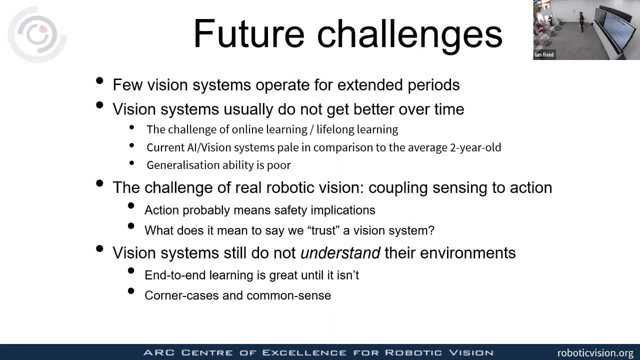 You just say, OK, well, memory is not so much a problem as it used to be, And searching big things is not so much a problem as what it used to be. Let's just continue to build a big database and search the database. 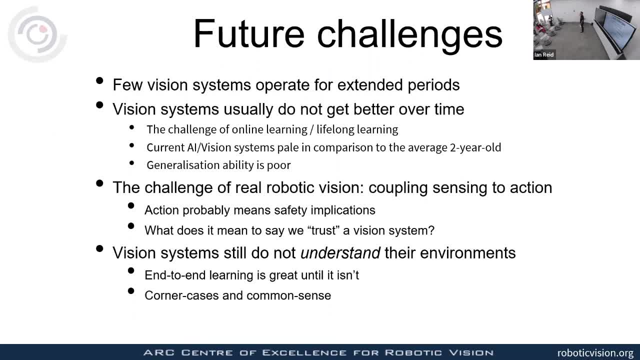 That's actually pretty interesting. So my last question is regarding the fact that you mentioned that generic feature representations is kind of important in this context. However, there's also, for instance, recent attempts in making general purpose vision systems. For instance, if the community is solving different tracking problems- single target tracking, multi-target tracking- how we can have one single unified architecture, that kind of inputs? 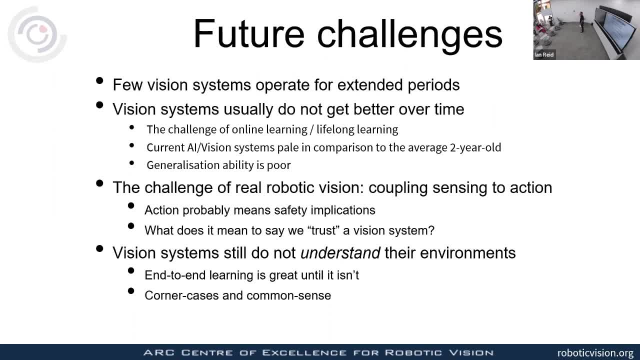 The input is the same but the output can be different. It could be multiple targets or single target. I just wanted to believe that could be the way to go also in geometry, for instance, having general purpose systems that kind of solve different geometry problems. 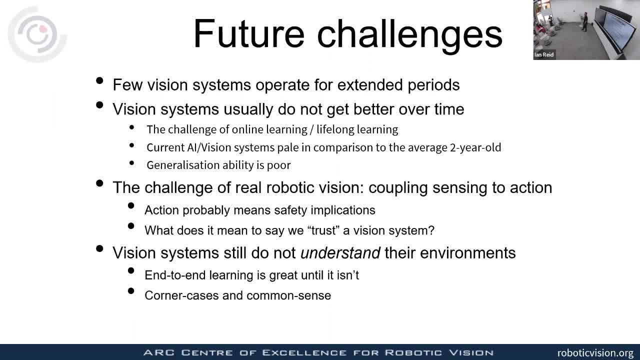 OK, Thank you. I haven't thought about that particular problem, But yeah, I can see that it could be valuable. I worry a little bit, maybe that are we asking too much of a particular system to get it to solve all of these problems? 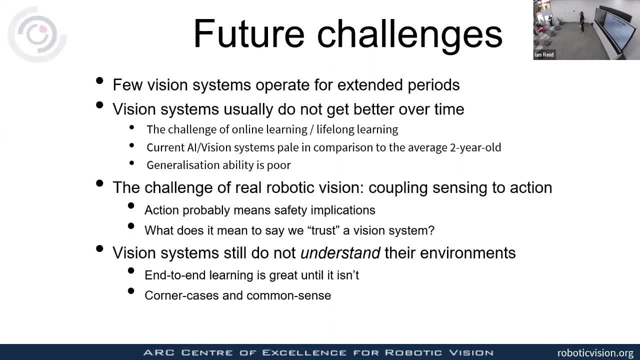 And do we even need to do that? I think probably. well, let me give you an analogy which may or may not help about my thinking, And this is in terms of robotic control. And there are various people who've thought about: well, how do I do robot control when the environment changes? 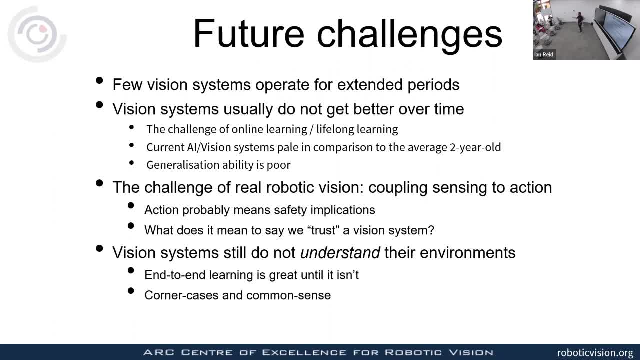 Do I have a switchable control regime- Maybe that's the same as your all singing, all dancing network- that can solve all of your tracking problems. Probably, to get it to do that At some point, you've got to have a switch that says: well, this is the environment that I'm in. 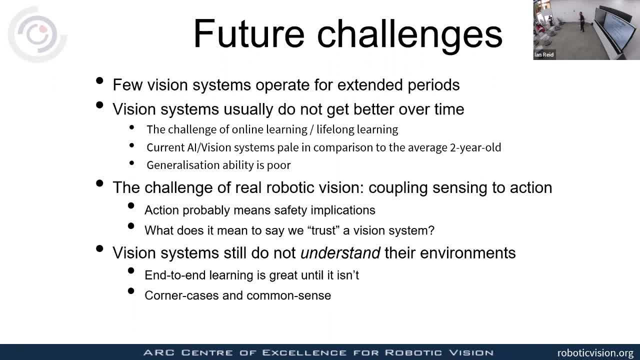 Choose this one or choose this one, or choose this one. And a nicer solution in the robotic control one is one that Jitendra Malik is touting at the moment, which is to say, you try to model the physics of the world and you have one policy to move your robot. 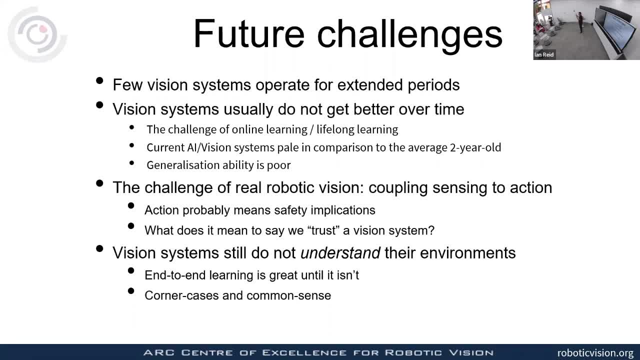 But that policy is informed not just by the current state of the robot, But by your measurement of the environment as well, the physics of the environment, And we're thinking about that in the context of sensing, where we want to be able to do sensor fusion between vision and lidar.